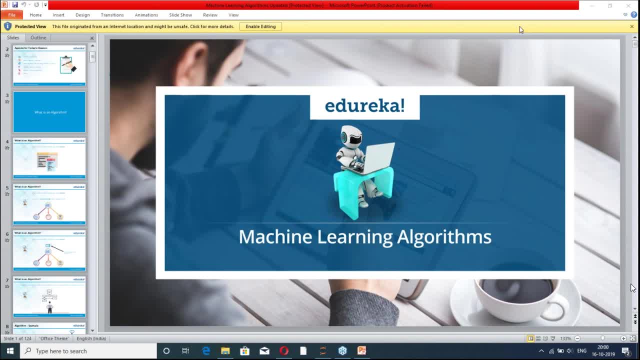 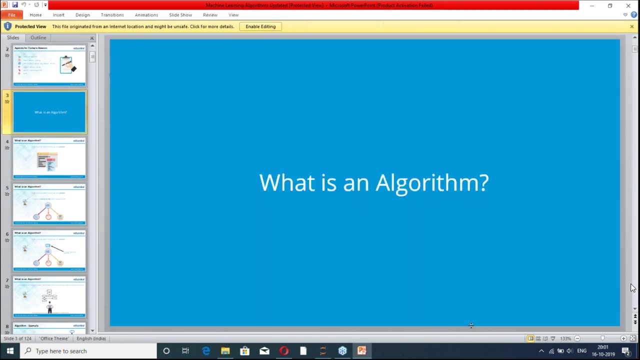 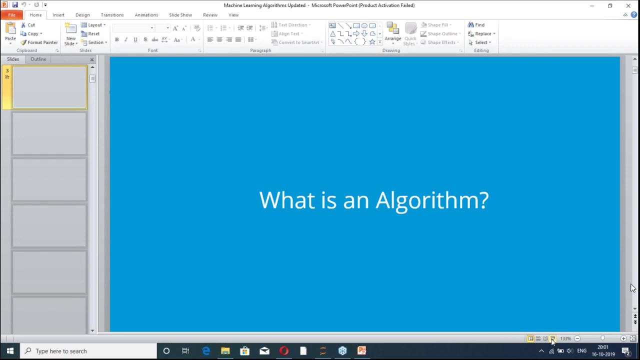 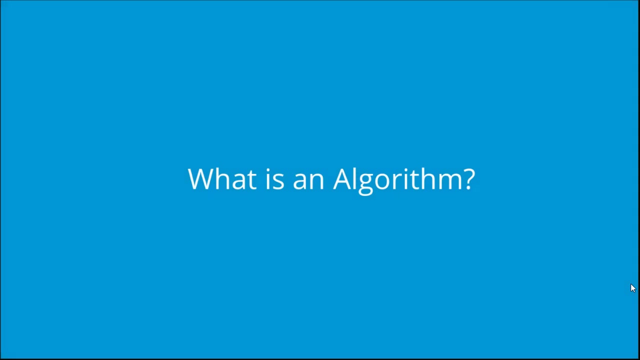 Am I audible? Yes, great, So we can go ahead. Okay, so, before starting the things, we are going to talk about some of the basics, even though some of people might know about these things or might have attended earlier lectures in which we had a little bit discussion about them. 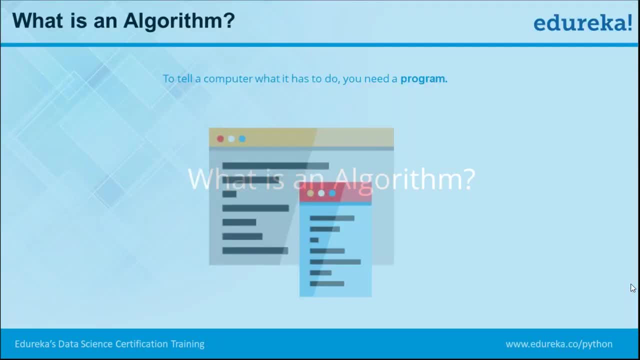 So let's talk about what is an algorithm? So algorithm is the way to tell your conversation that what it has to do, right? So you have some steps, you have some problem in your hand which you want to solve, and the problem needs to be solved by, in reality, by the 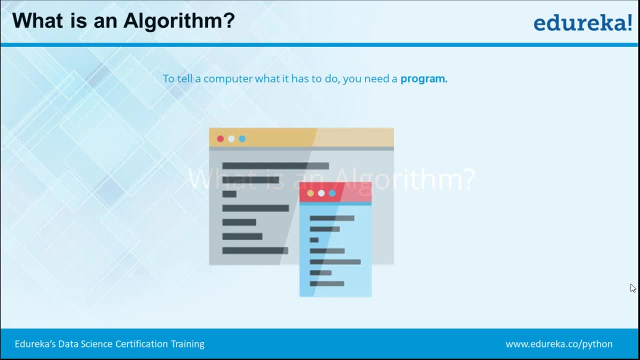 computer, But you will tell the computer that what are the steps which it needs to carry out so that your problem can be solved. And that is what you do through by writing a program And through the program you are telling what is exactly. the algorithm is right, Or we? 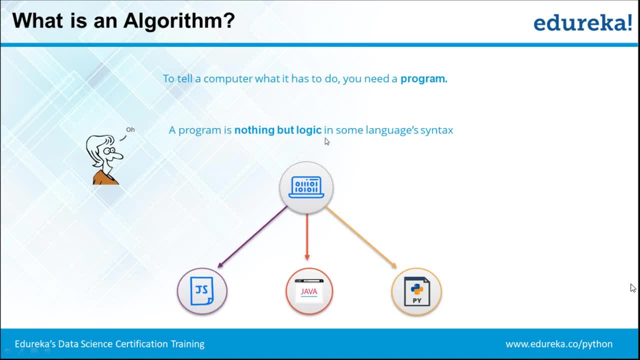 can say: the program is nothing but the logic, right? So logic how the problem should be solved, They should be the first step, they should be the next step, and so on further. So these things are your logic, which you are defining using some kind of language, syntax. So you 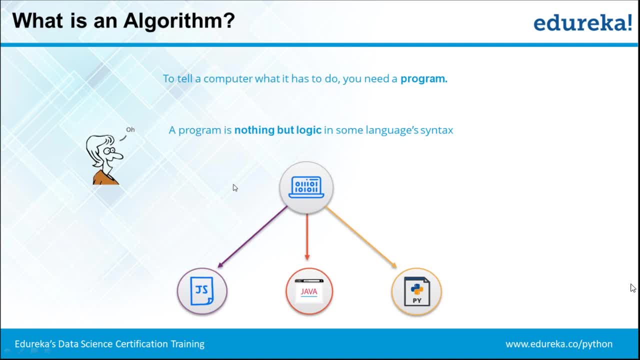 might be using Java, maybe Python or JavaScript, right? So any programming language you might be using to tell your computer exactly what it should do, right? And that's two in the form of the steps. So that should be the first step and second step, and so on. Okay, so let's. 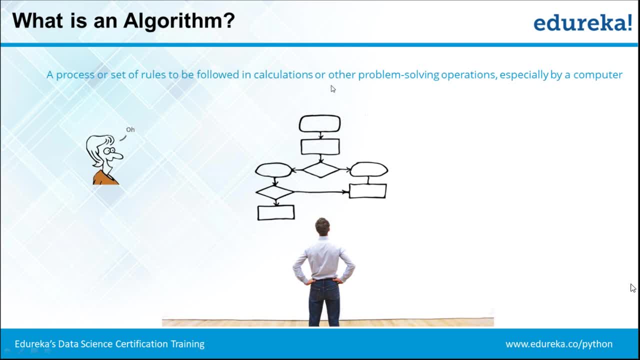 talk about a process of set of rules to be followed in calculation of other problem solving operations, especially by a computer, right? So this is what we have done, exactly: You are telling what to do when at particular time, right? So let's say you want to write. 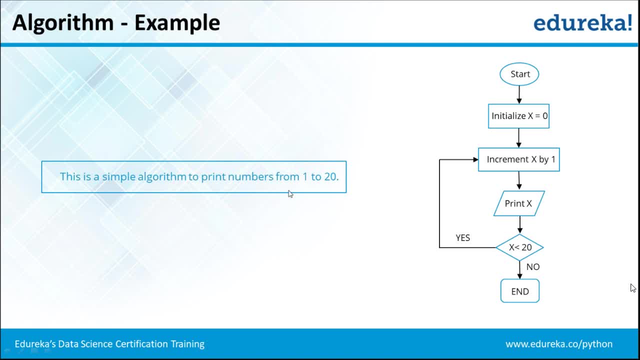 an algorithm which will print the numbers from 1 to 20.. So how you are going to do this thing? in a simple way, Let's say I'm using first one variable which we are, to which we are allocating value 0, right? So after allocating value to 0,, then we are going to 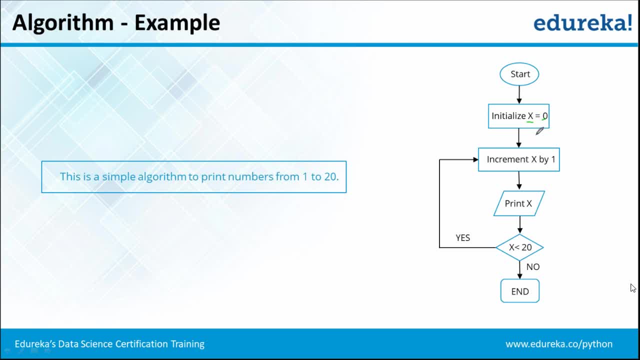 you increment the value of X by 1.. So after that? so what become? X value is 1, and once it becomes 1, what you are doing here you are printing the value of X, So it will print the one. then you check. the condition is: axis is still less than 20, right If it is less. 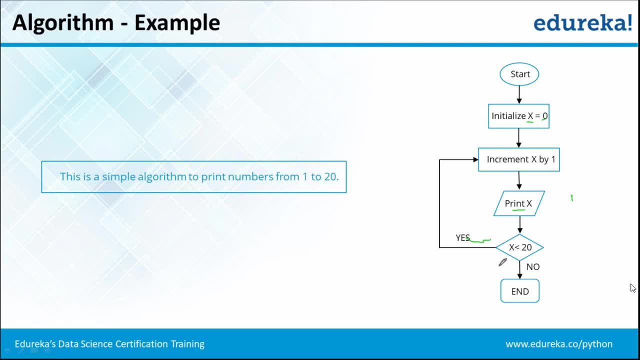 than 20,, then you will go here right, or if it is not, then towards the new you will come and here your program will end. but when it is one, it means still it is less than 20.. So this condition would be true. you go again back to this loop, where again you are saying: 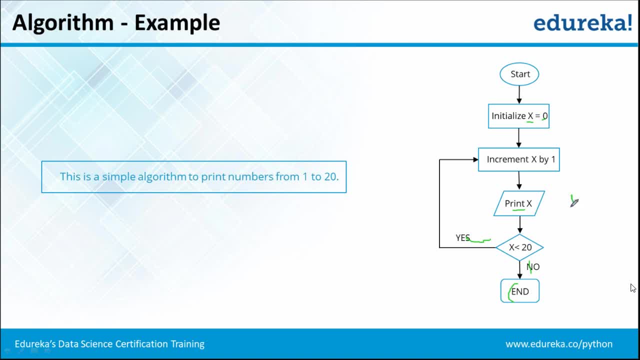 it. increment the value of X, buy 1.. The latest value was one. when you increment it by one, it becomes 2, then you print the 2, right And again you do this check condition. So you keep doing again and again this same thing until you reach the final point where 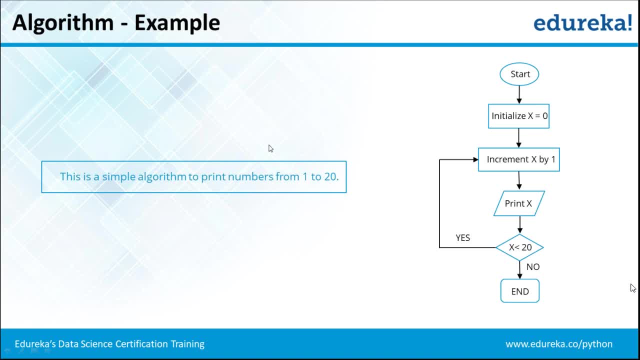 you have printed all the numbers- 20,, right? So this is an algorithm. all these, This is a rules You are telling to the computer so that computer will follow these rules and do the work on your behalf. So let's talk about what is machine learning. 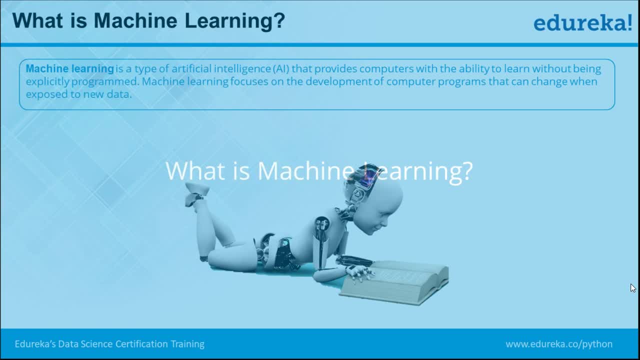 So machine learning? is that so, is it? so? there are two questions might be here. First of all, yeah, definitely, we're going to see what is machine learning. Secondly, is the machine learning algorithm is exactly the same kind of the algorithms which we have been talking till now? 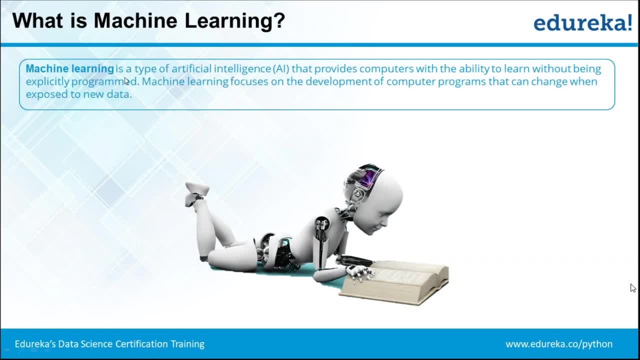 or is it something different compared to that? So if we talk about the definition of machine learning, then it is a type of artificial intelligence that provides computers with the ability to learn without being explicitly programmed. So here we are bringing one term that it is giving the ability to learn right. 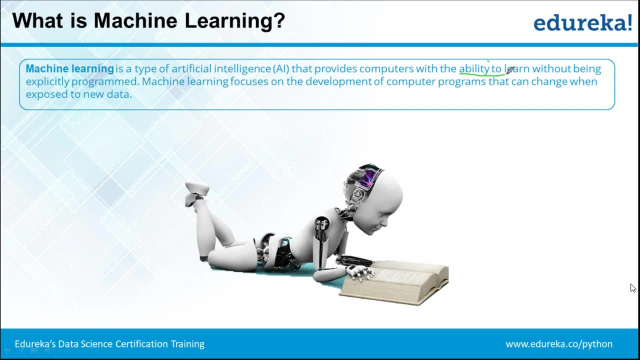 So it is giving ability to learn to the computer itself. So computer will learn automatically on its own. We doesn't need to program it explicitly, right? So what does it mean programming explicitly Like if I am writing a program where I am telling each and every staff 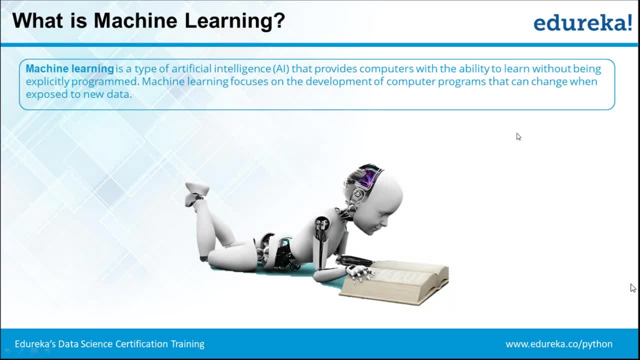 to the computer that it should do now this thing, then this thing, then this thing, then this is equivalent to programming explicitly. But if you are not telling it, but you are giving the ability to computer to take on its own decisions, right. 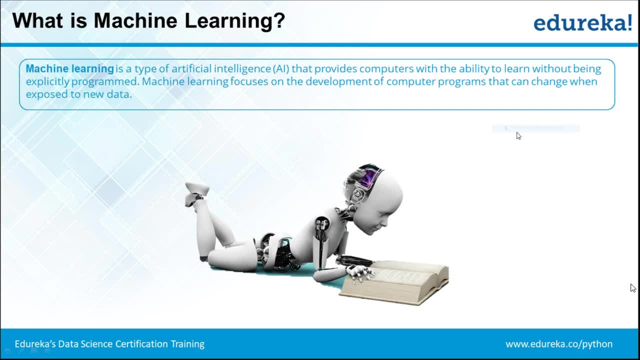 So after that, you don't tell exactly how to print the number from one to 20, but you just tell: print the number one to 20, but it has automatically learned how it can do this stuff right. So learning this thing that so that you doesn't need to. 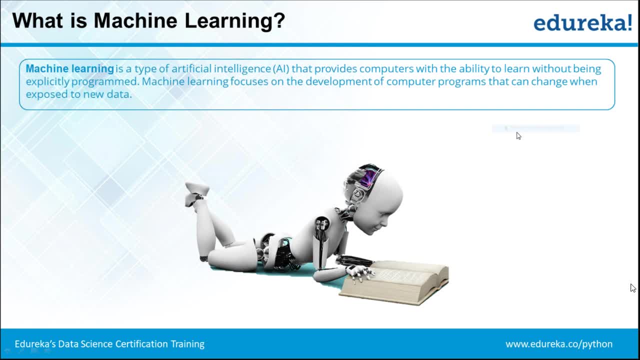 explicitly learn right. So we give these steps to the computer to do the or to carry out some kind of task, right, That becomes your machine learning. So we are giving the ability of learning right. So, like human being, if I talk about this particular, 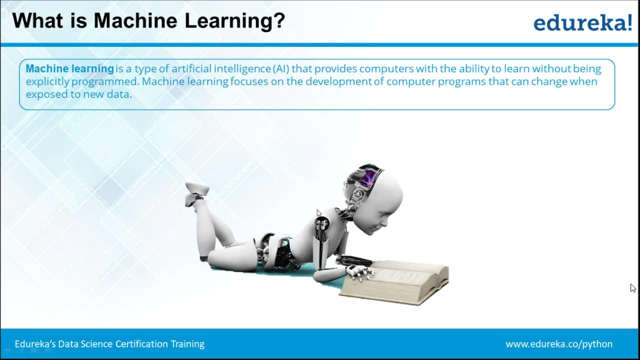 if I talk about for printing on, let's say, writing the number from one to 20 to somebody. once I teach you this thing, then you learn it right. And it is not only one thing you learn, but many things you learn. 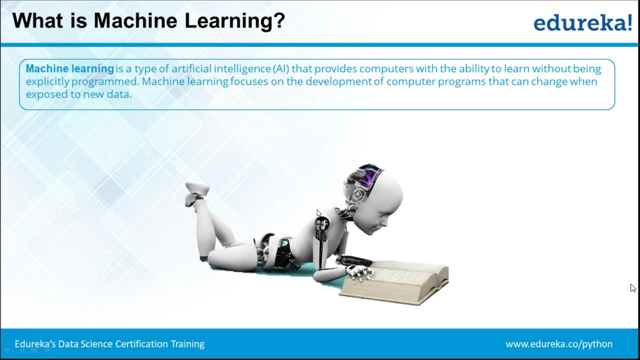 And then I doesn't need to tell explicitly right, And then I doesn't need to tell explicitly that what to do at which particular case, Then whenever any such situation arises, you automatically take your stats right. So the same thing we are going to do here. 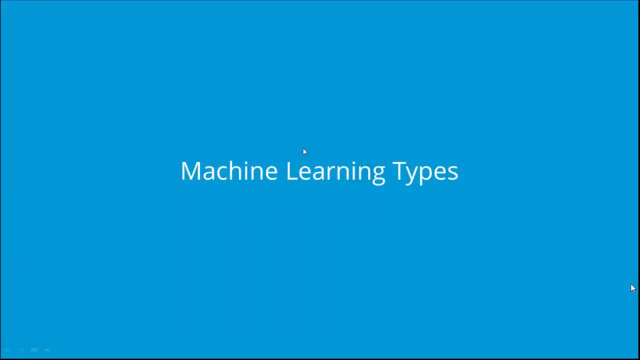 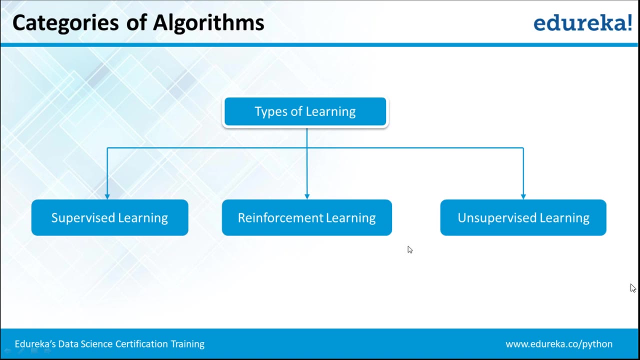 when it comes to machine learning. So there are different types of machine learning techniques, are there? One is like supervised learning, reinforcement learning, unsupervised learning, right. So we had a little bit introduction to them day before yesterday. So quickly we will go again here. 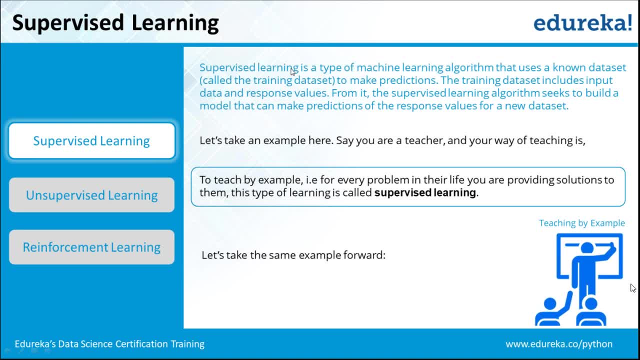 So supervised learning are those kind of algorithm where you are supervising the training right. So, in reality, what do you mean by even you are is that you are not only giving the problems right. So it is equivalent. let's say: I want to teach you mathematics, right. 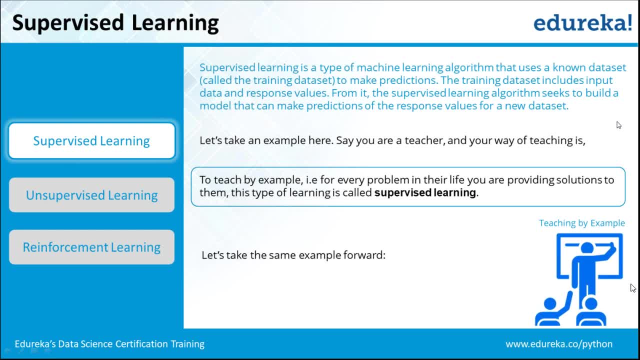 And I bring, let's say, a book. I took a book and in the books there are, let's say, a hundred questions are there in my book. So out of these hundred questions, what I might do is I take the 70 questions. 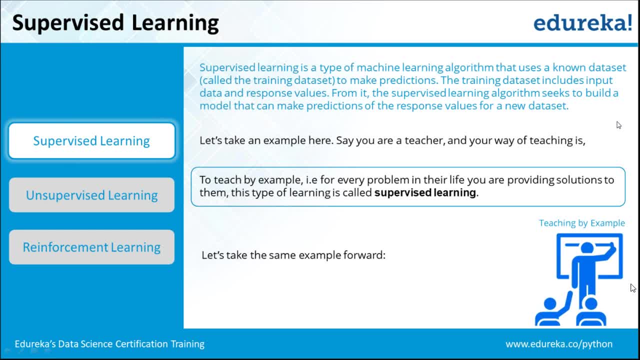 I show you those 70 questions, and while showing those 70 questions, I show you their answers as well. to you right? So what I am doing here is I'm not only showing you the question, but I'm showing the solution to that. 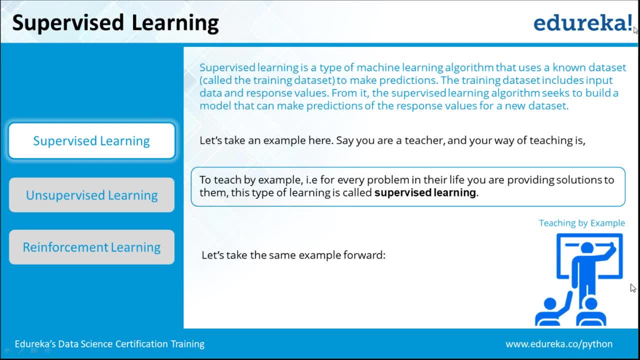 So it means this is supervised learning, because I am telling you how to solve the problem right, Or what is the solution for each of these problems. So these kind of technique becomes supervised learning, because we are supervising this right. So you learn now these using these 70 examples. 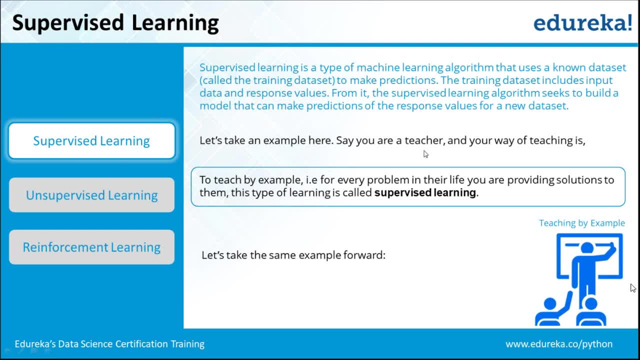 Under supervision or by looking at the solution of these and then, for the next 30 question, might be conducted as a test for you, where they will be knowing exactly that how good a particular person has learned right. So the way we check with the human being, 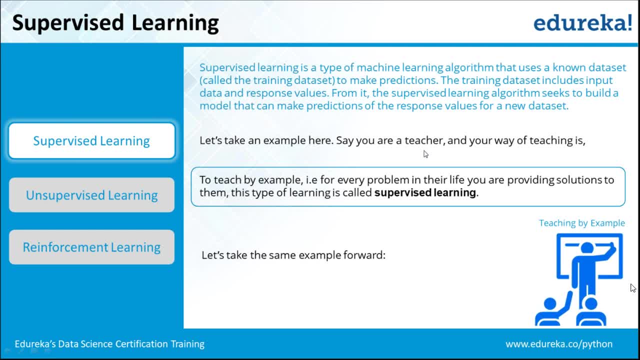 by conducting the test. similarly we do with the, our machine learning technique. First we give them the problem, We give them the solution. Then it's the duty of the machine learning algorithm that it find out What is the relationship between the input and output, or begins a problem. 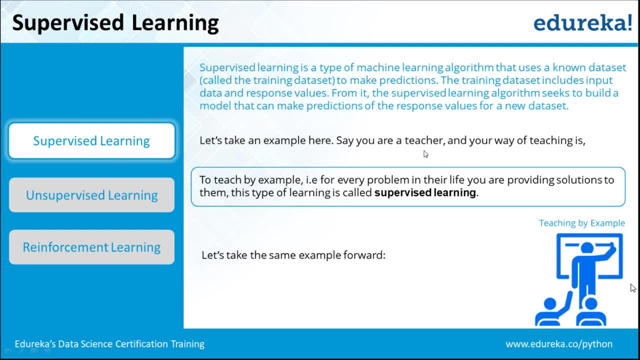 and the solution so that we are not telling it exactly that how it can reach to the solution. but we are giving the problem, We are telling what is the solution for that and automatically machine learning techniques start learning from by looking those problem and solution on its own. 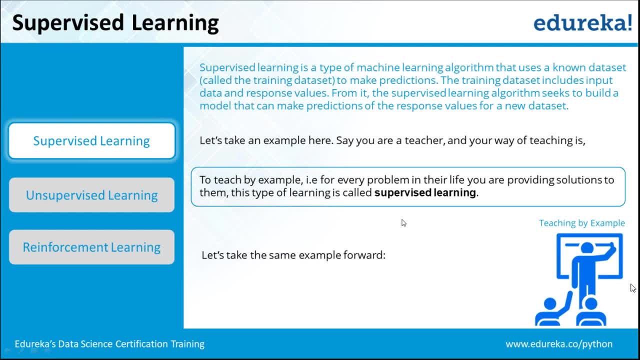 and later on you can make the test, give 70 questions and it will 70 question. you teach that maybe 30 questions. you keep in secret with yourself And then you do not show the answer to those 30 questions to the algorithm. You just give what is the what is the questions. 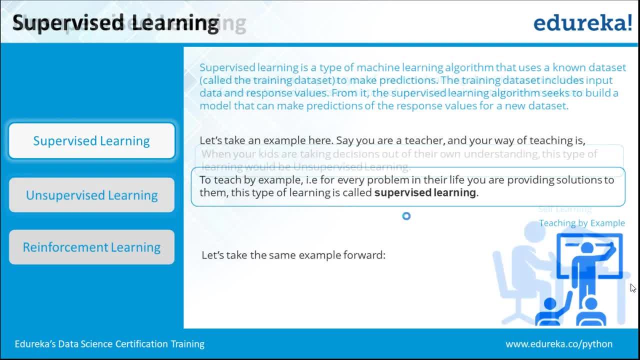 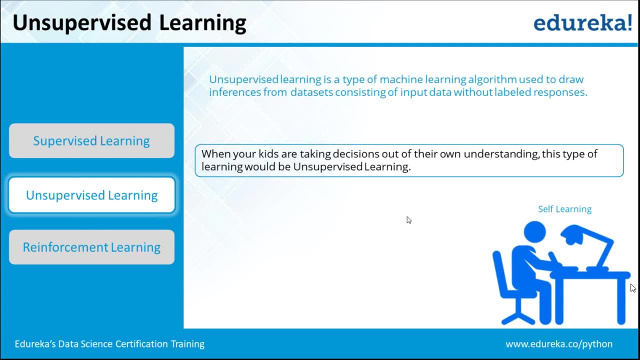 and then it will give you the solution. and when it comes to unsupervised learning, nobody is giving you the solution, right? Nobody tells you so. for example, let's say: if I want to you to learn, let's say from images, right? 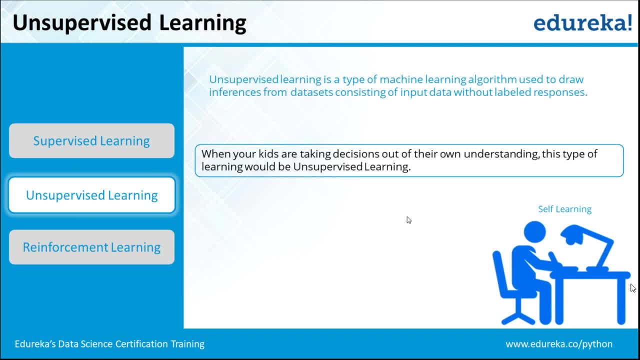 So if I give you images- for, let's say, it is a fruits image- I give you the fruits image and I tell you also that which fruit image it is right. This is apple, This is mango, This is banana. So this is a supervised learning. 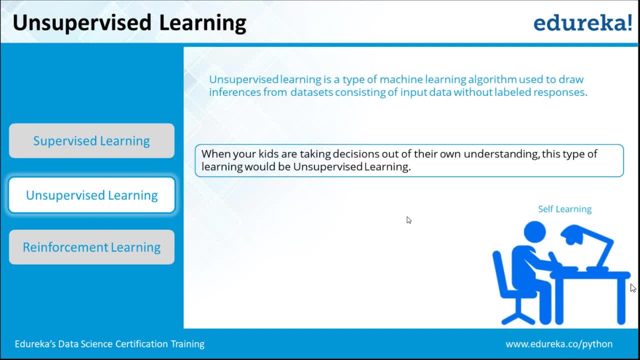 because I am not giving you only the images, but I am giving you the solution. What is the name of these images? in unsupervised learning, We do not show the solution right, We just give you the images and from the images you have to learn right, so automatically. 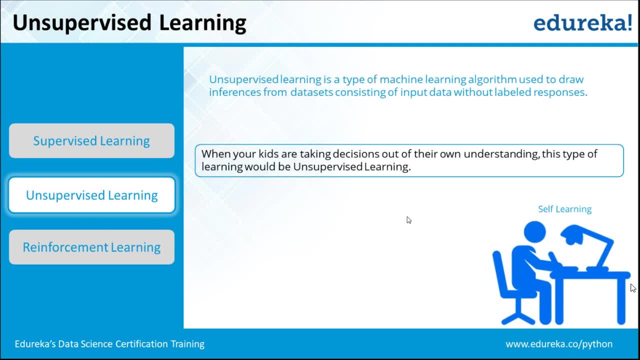 So this is where it comes to unsupervised learning. It's mostly is like work is of the clustering, actually Our grouping, so that you, by looking the images, you can group the similar images together, right? So this kind of techniques where nobody is supervising the things, 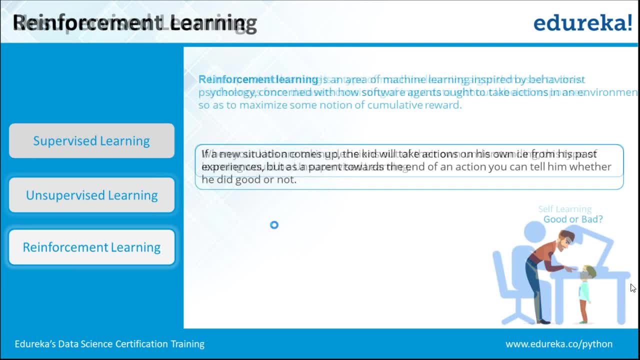 we call it as a unsupervised learning. Next is the reinforcement learning. This uses the psychology of human being, right, or the child behavior, the way a child learns from his or her parents, right. So whenever child is doing something good, you, the parents, 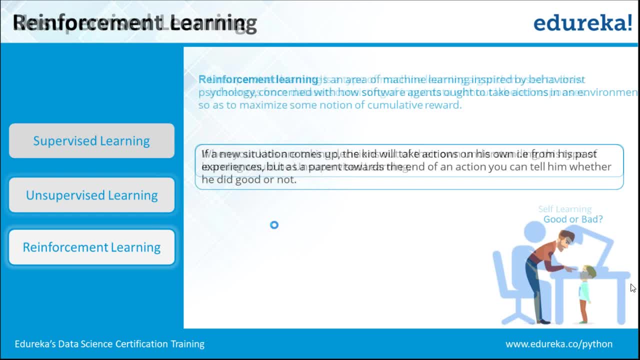 of the child, appreciate the child and because of which I'll understand, okay, this particular situation. This is the action which I need to carry out right and similarly, whenever child is doing something wrong, You might become angry or you might say: do not do this thing, or whatever right. 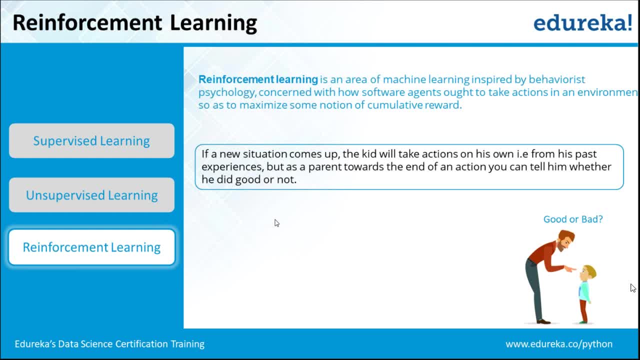 But you are telling somehow, or is true, The child is able to make from the context that in this particular context He should not take this particular action. So same with the reinforcement learning, and it is about teaching the skills to the, to the computer right. 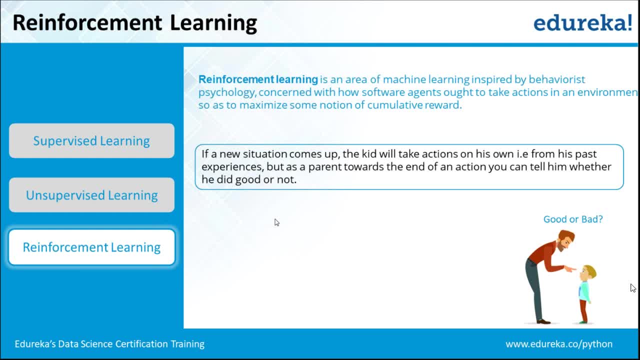 So there are like skills We might want to teach our computer how to drive the car right now. What is driverless car? are there in which computer is operating no driver computer itself take the action. So this is a skill right. So similarly we have other things nowadays. even I think I told you guys earlier 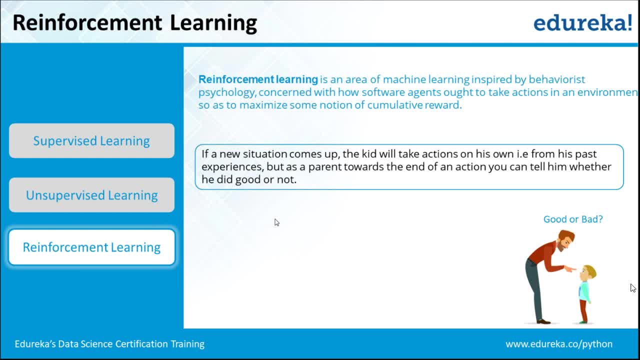 as well, that there had been system, system had been made which is music system- right, That is music production actually system. Then you doesn't need to do anything and this particular AI based system can generate the music as any human being generates, and that's not something completely random. 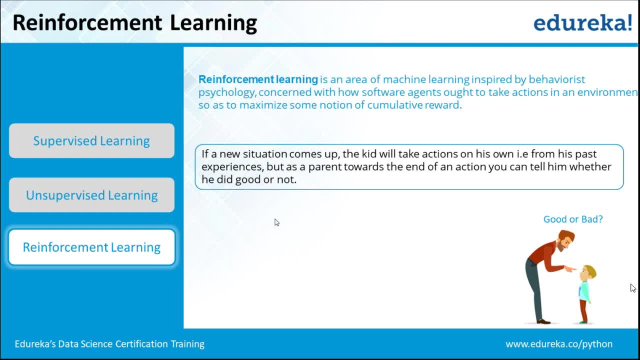 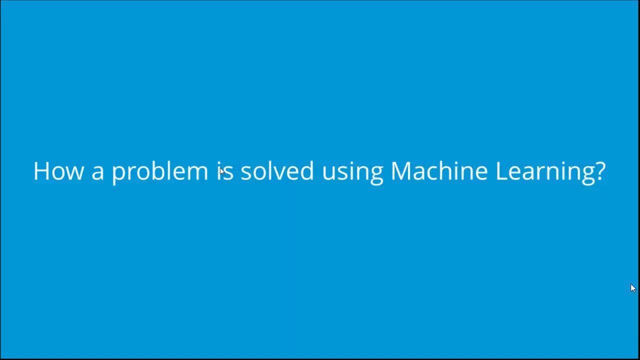 but very melodious and properly, with taking care of all the rules of the music or notes or whatever those are. So they are reinforcement learning used. or if you want to make a system which can learn, let's say, chess, You want the computer to be a very good at chess, that you use. 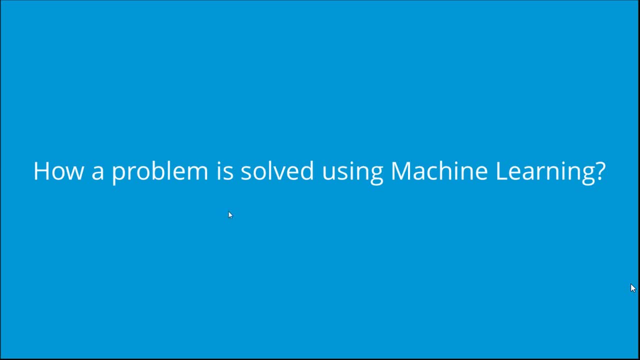 Use reinforcement learning and I don't know if you guys are aware about this. one game- I think it is its name is play go. probably it's a Chinese game, or I think I'll fuck. go with the game or play go. I don't remember exactly the name. 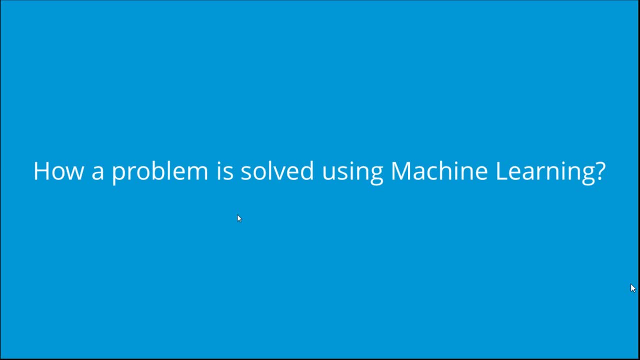 So this game was taught by the. so this game was learned by the computer. first by using the reinforcement learning where it takes action again and again. It is learning by, like human being, only where it plays again and again. So it played many times against itself. 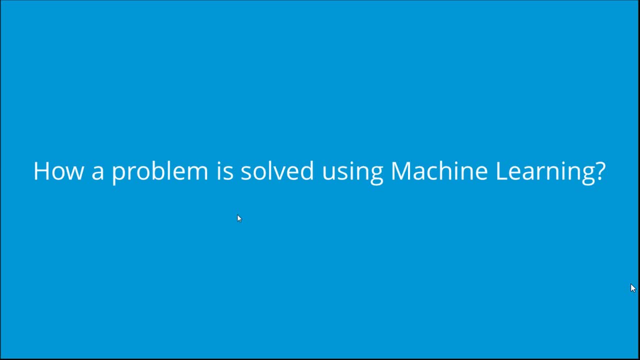 Computer played against itself this particular game and was learning this strategy that it was playing right by looking at the what good thing a score it is getting- or bad score is it is getting- by taking a particular action and after that, after it is being trained and they conduct a competition against a world champion of this game. 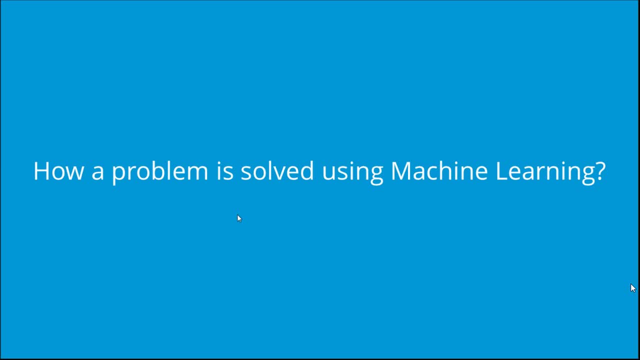 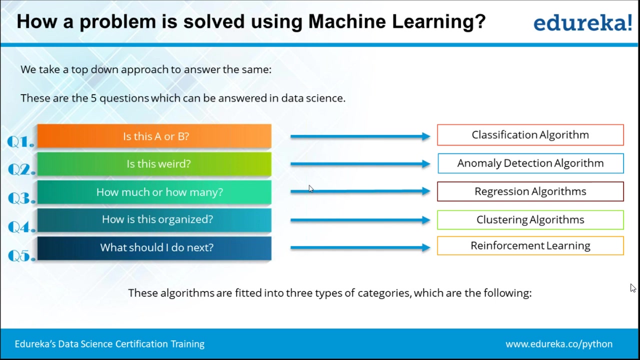 and computer bag has beaten that particular champion in the game right. So you can see how powerful this reinforcement learning is. Let's see how a problem is solved using a machine learning. So some of you, the older one who have seen the first class, might have gone, seen already this slide here. 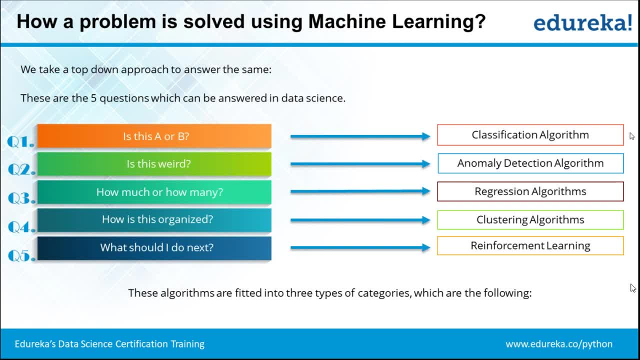 We say there are different kind of techniques, are there right? So the top three techniques like classification, anomaly and regression, they all are the supervised technique. only this clustering by is the unsupervised. and reinforcement already you know it's itself. So what is when it comes to supervised learning? 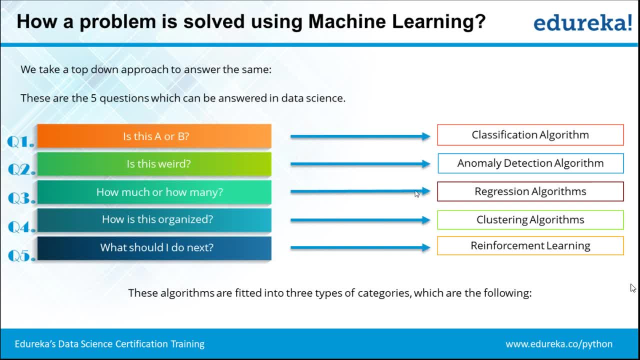 We are saying we are not providing only the input to the computer, but we are providing the output values also to the computer, right? So, like images, we are not giving only images, but we are telling also that what would be the output of, what is the name of those images? 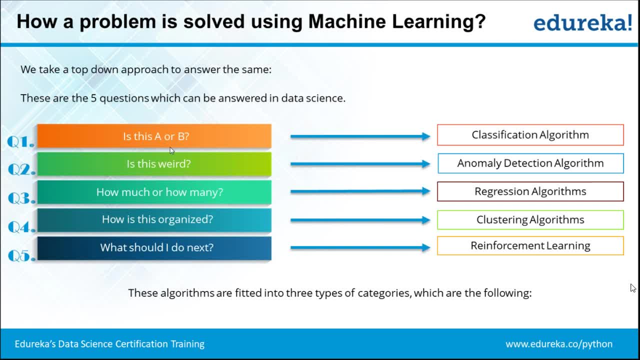 so that it start learning, right? So now we call their output values the kind of, let's say, we are talking about fruits images, right? So five fruits images. It might be there, right? So jaggery Achilles saying hello, Yeah. 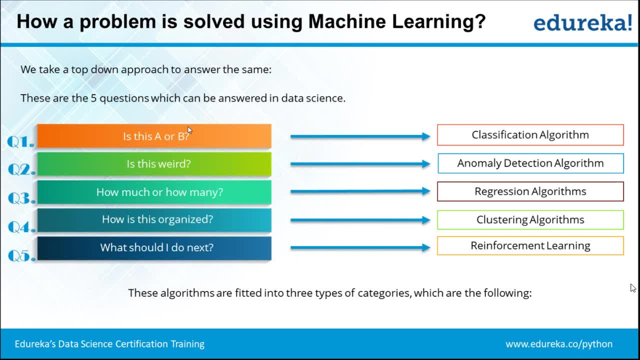 Hello jaggery, Is there any question you want to ask? So whenever anyone I want to ask question, feel free to write your query. Okay, so we have been discussing about the. so we were discussing about the classification technique right or classes right? 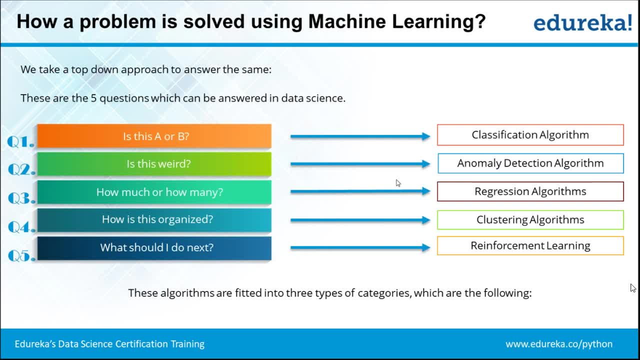 So output values are given. Now, what kind of output values these are? that is what is defining the type, Let's say the number of output values. our problem has is limited, right? So let's say we are, we want to detect whether a person has cancer or not. 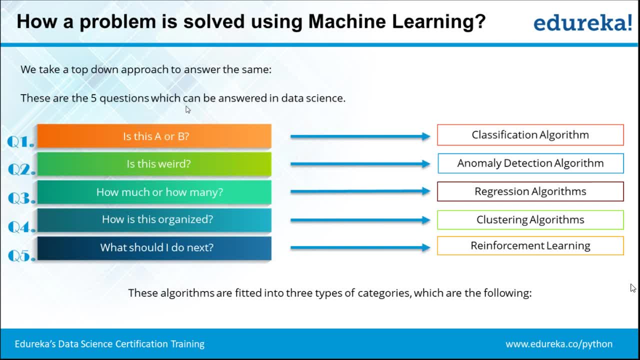 So there are only two output classes that that person will have cancer or he will not have. so that become a classification algorithm and only is something where the thing is out of group, completely right. So a week say that anomaly, like is this weird, something, right. 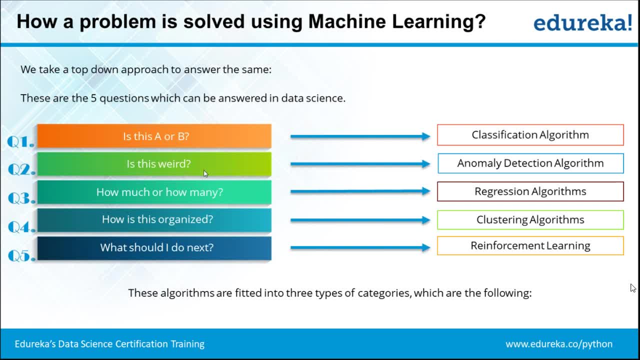 So, for example, if we are doing, let's say, a lot of transactions are being done in the back and we are looking that: is there any transaction which is fraud in my system? If there is any transaction which is fraud in my system, it is far away from the normal transaction on most of the transactions. 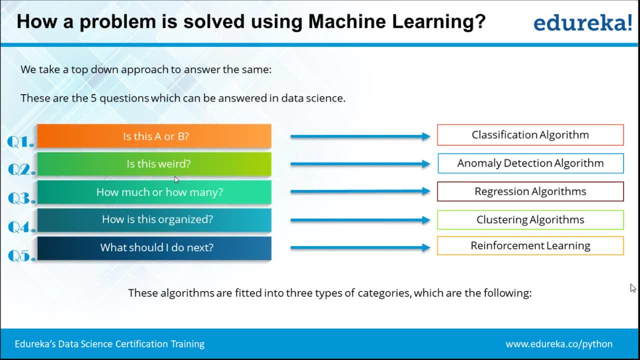 That's kind of issues where we are finding something which is not following the general pattern. We call this thing as an anomaly detection algorithm, regression, where we start having unlimited classes And say, right, So, for example, if I'm talking about the temperature, temperature could be anything. it might be 20 degrees Celsius. 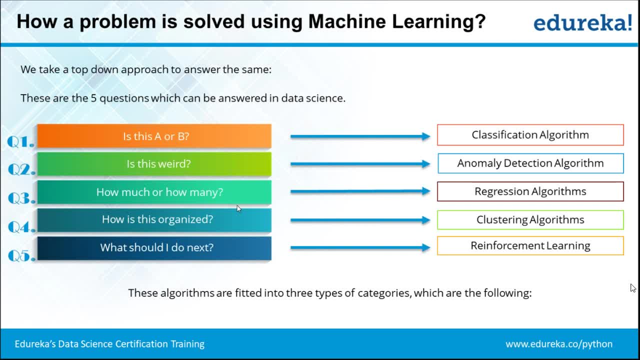 25 degrees, 20.1, 20.11, depending on how accurate we are, How precise our temperature sensors can give right. But yeah, this is. we can say infinite values can be given by regression algorithm, clustering algorithm. How you are organizing something right? 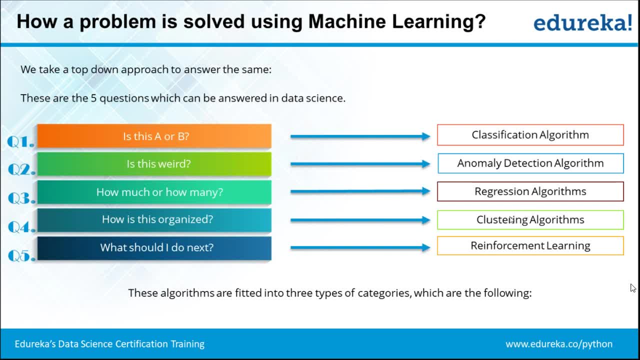 So like, for example, grouping of the things I took example earlier as well, that is, of the articles, right? So let's say you have created a website on which you allow anybody to post the articles and these articles may depend to any category. So people are just randomly posting the article and they belong to different, different categories. 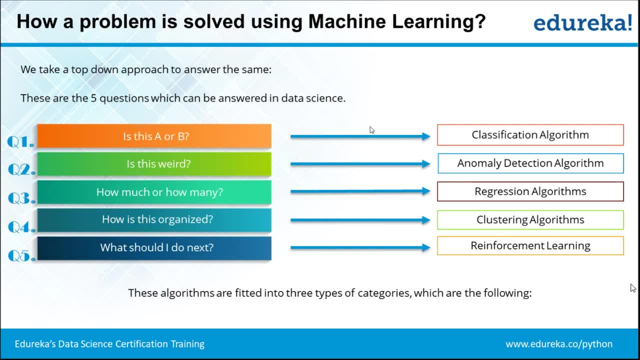 but they are not telling that to which category these particular article belongs, right? So Bharat is asking how we will check the students, question what they are asking. See, whoever write the question, it comes to me and I can read the question for all of you guys. 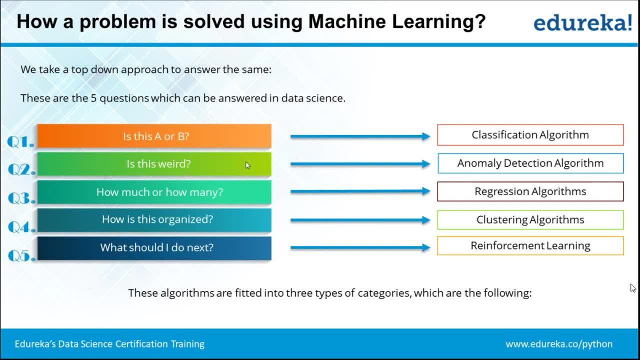 So there is no problem. Whenever anyone has a question, You just ask your question here. I will be doing and I will be reading it for all of you guys and then definitely I will be discussing the solution as the for the question. Okay, 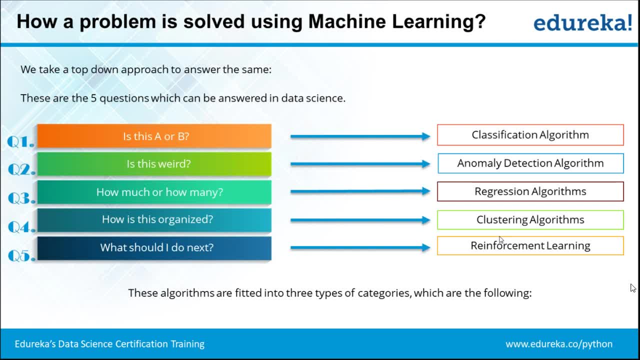 So we were discussing about the clustering algorithm. We say that there are lots of articles has been Posted on your website, right And? but these were not organized. nobody take care of world to decide what category it is right. But now, as it becomes many and many, it becomes pretty difficult for you to organize your website, right? 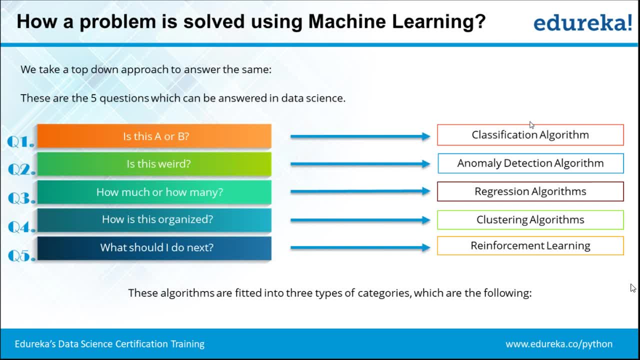 Because people come and then you cannot give what they, you cannot recommend them properly. So what do you start thinking? if I can organize them into a proper categories or maybe enough groups, then I can give good recommendation. Okay, So like, for example, let's say you did you just apply the clustering algorithm? 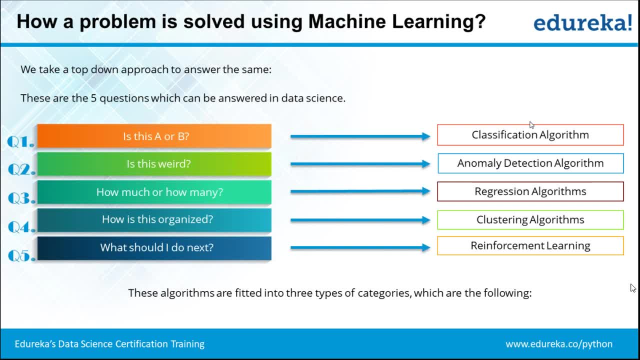 and because of this clustering algorithm, the groups were made in such a way that the articles which look to the singular would be grouped into a one group. the articles which look different, they would be grouped in a different groups. right. So now, whenever somebody is reading one news from one article, 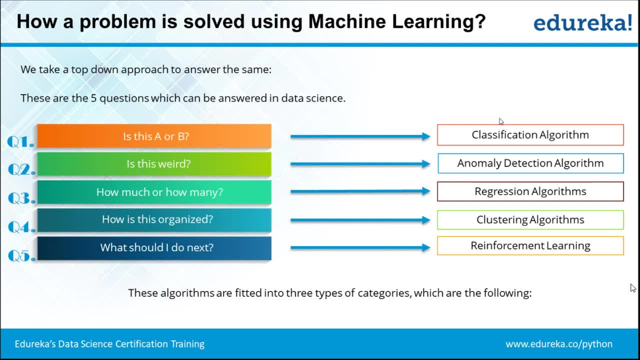 then you can. you can suggest something to the same In a blogging to the same group, right? So, jag, we actually is asking a question I will take because this is like, not related to currently. this slides and off. So you are asking: what is the best certification for data science? 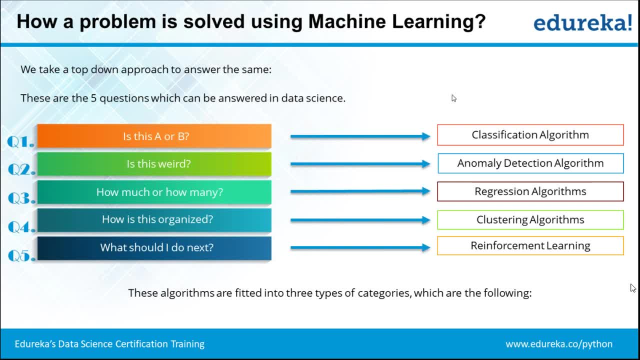 We will be discussing about it and that you just remind me. right Let's, let's focused currently here in the topic. and then we have the reinforcement learning, as I told already to you about the reinforcement Learning right, So it is about teaching the skills to the computer. 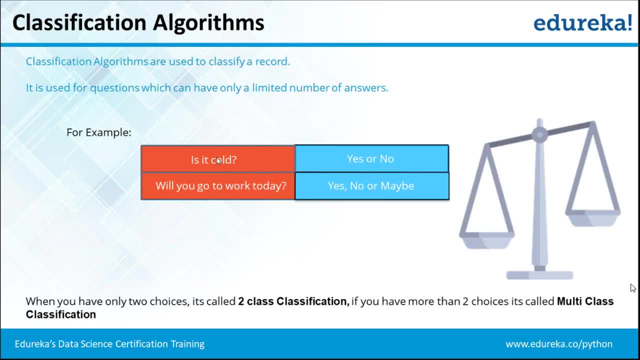 So here, so like classification algorithm They are giving, is it like that? It would be like probably, like where we have been limited number of classes, like we want to know is it cold or not? So yes or no, we can say. will you go to work today? 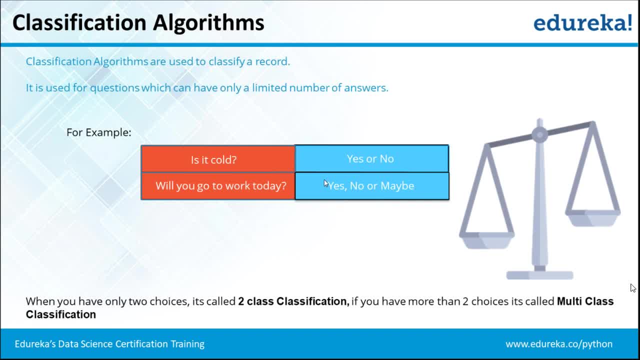 Yes, no or maybe right. So three are set. three output values can be there. So whenever we have the limited output values that can be taken, then we call them as a classification problem. So where we have the two choices, we call it as a two-class classification or binary classification. 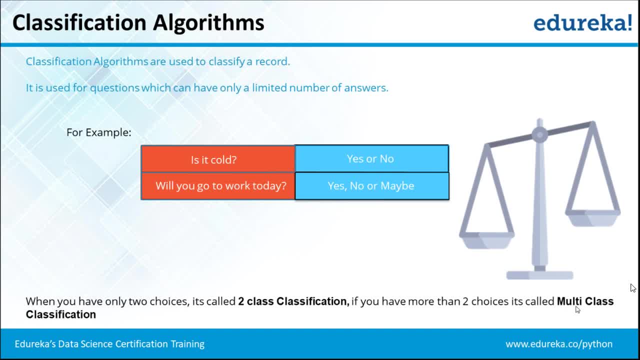 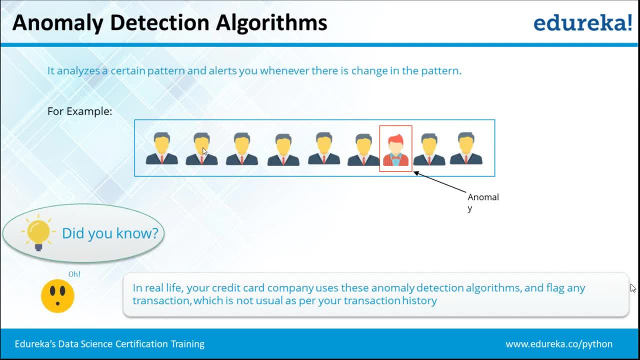 and whenever we have more than two choices in the output classes, we call it as a multi-class classification Here, anomaly detection. So if you see all these people, right, So all them looks alive, right, But just this person is different, right. 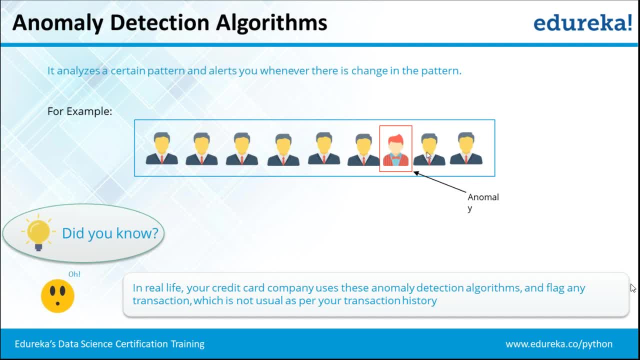 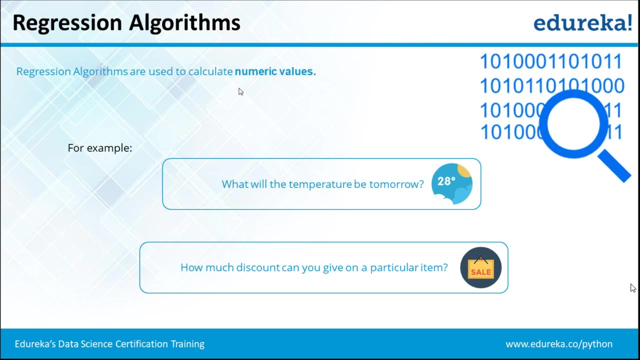 So this become anomaly because this is not following the pattern. What is followed by Most of the data points, right. So anomaly detection is if something is weird, right, Something is not as generalized a common way. So regression algorithms are used to calculate the numeric values mostly. 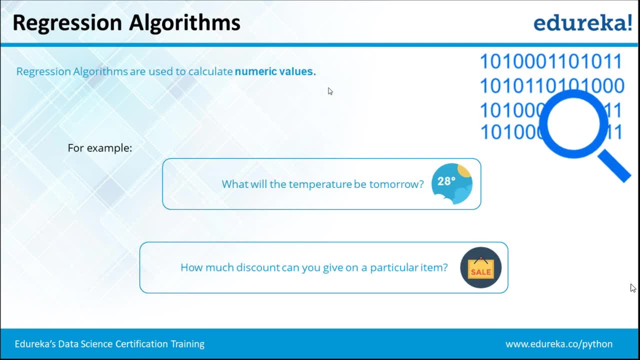 because if you talk about the infinite values, then it is. it will happen with the numeric values, only, right? So, for example, what will be the temperature tomorrow, or how much discount can you give on a particular item? right, So, wherever the numeric values are there, and it can be anything, right. 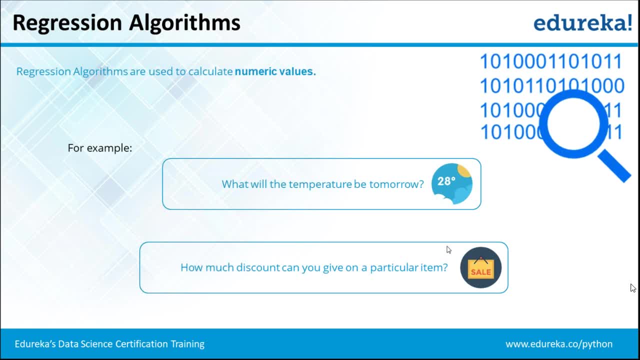 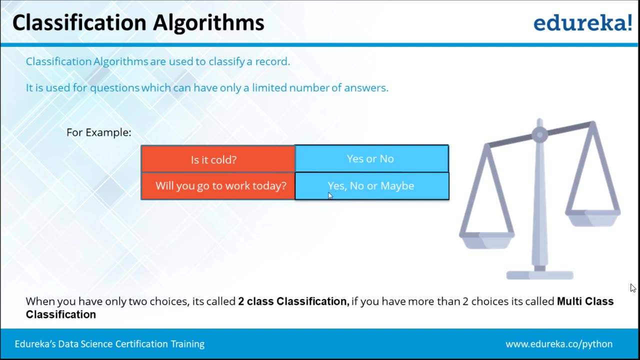 Real values. specifically, we say real values, then it becomes infinity, right, So we use their regression algorithms. technique, right. So if you see here like in classification, you can see here two categories in this push question, only two output values in this particular problem statement. 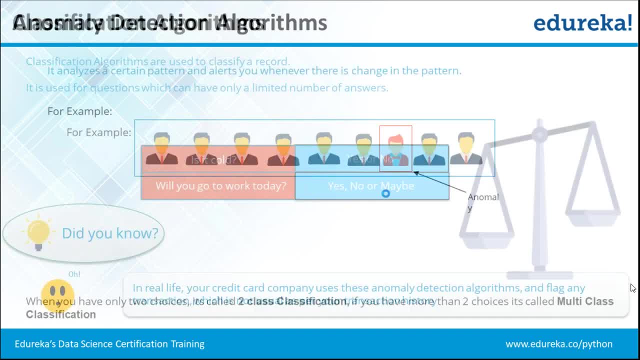 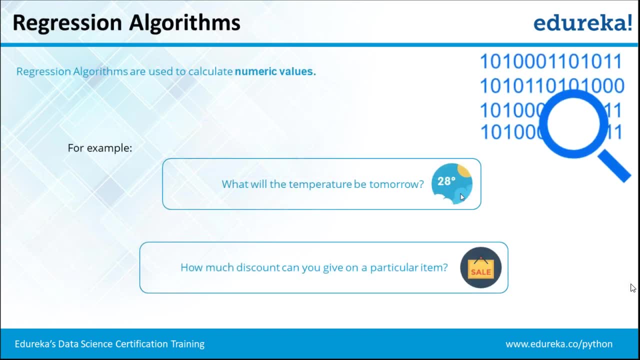 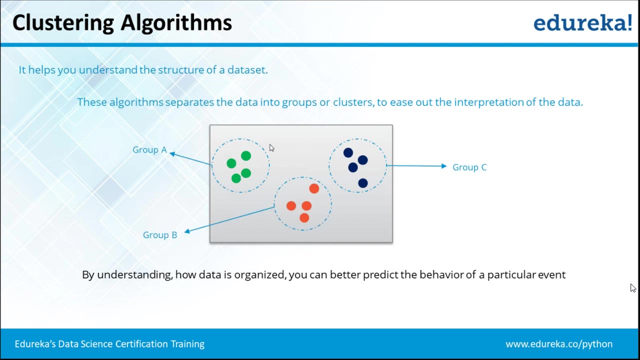 There can be only three output values, but if we talk about the temperature, there it can be anything right: 2526 or 26.1, 26.2.. Infinite possibilities are there, And as we talk about the clustering, it is about grouping the similar items together. 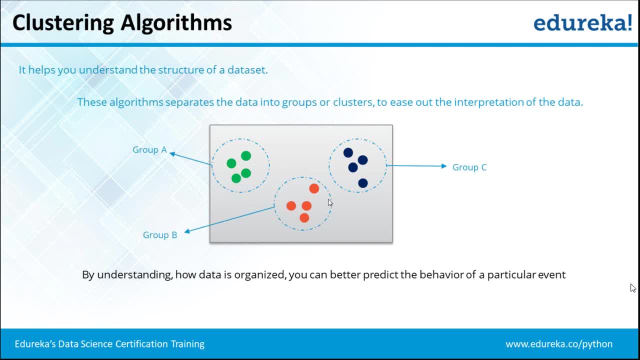 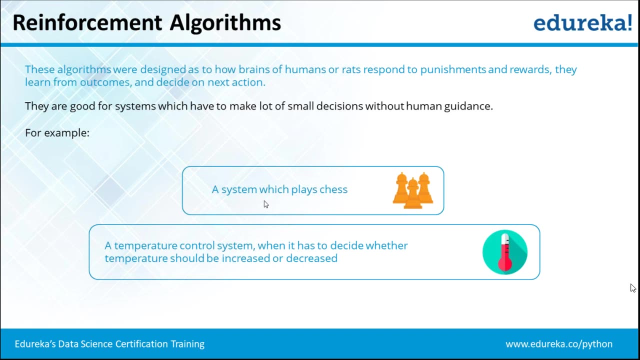 right by looking into the data, So they. it looks into the data and find out which others are items and group them together. So it helps in organizing right. So this is what clustering to reinforcement learning. as I told you already, This is basically most more like giving the skills. 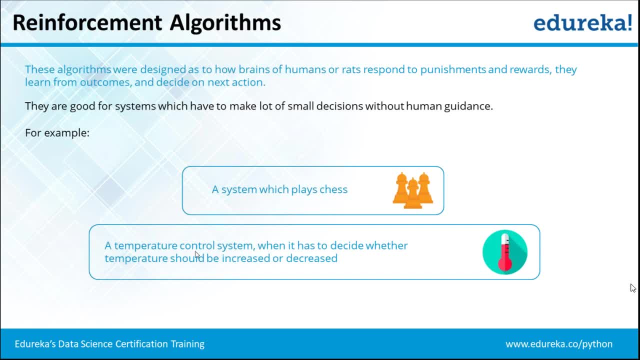 like a system which plays chess right at temperature control system when it has to decide whether temperature should be increased or decreased, right? So like if you sit here, if you sit in your room, and then you feel is it cold, then you start thinking, Okay, I should reduce it little bit or I should increase it, right? 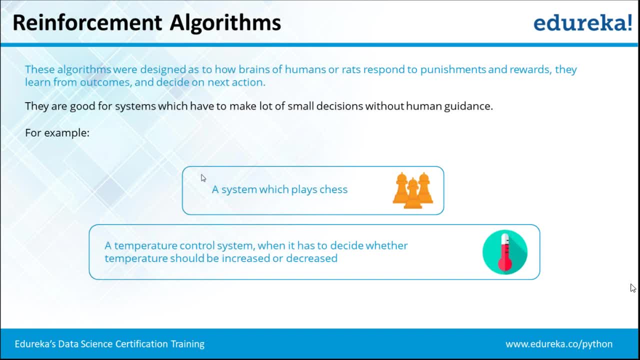 So giving the decision powers here And that work completely on the punishment and reward system, right? So it is more like Doing this tap again and again, So learning by doing. we can say this thing for reinforcement, right? So, for example, if you're talking about the driving car, 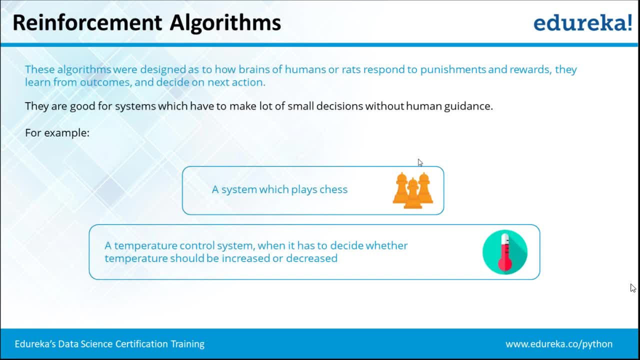 so if it is taking correct turn, then you give the reward. if it is taking wrong turn, then you punish it right. So there is a mathematical way, which is defined, to give the punishment and reward. It is not like every time human being will come and say: 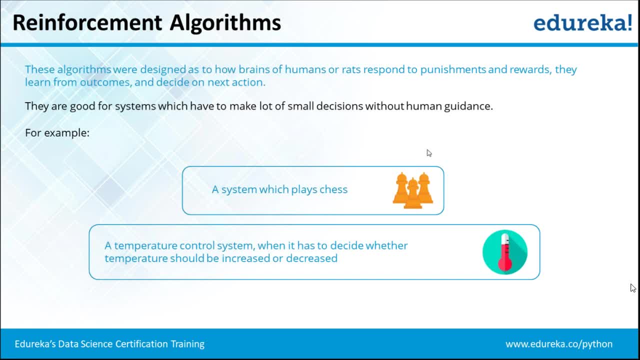 okay, this is punishment for you, This is reward for you, right? But we need to define some function mathematical which would be enough to take, Take care of all the cases for punishing or reporting, So we can divide our algorithms like machine learning algorithms divided into three parts. 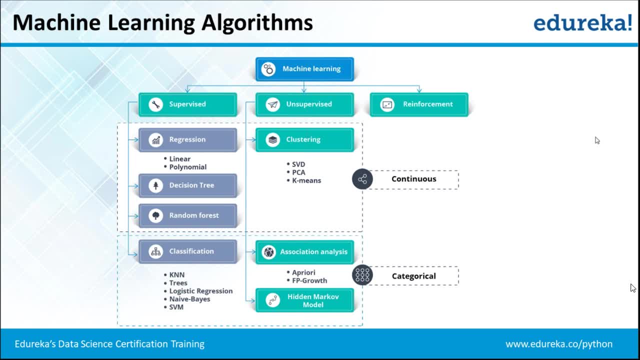 of provisor was reinforcement. So there are many different kind of techniques are there. So, like in supervised, we might have the creation technique. So regression is like linear regression, polynomial regression is there, and then we have the classification technique, So these decision tree and random forest, they are actually coming in. 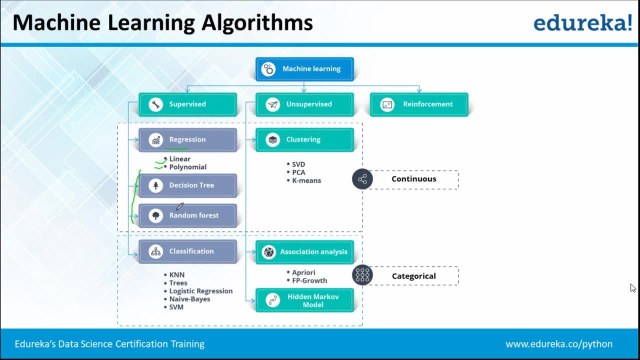 In both cases it is being used for the regression purpose as well as for the classification purpose, right, So you can use for both of them and these further algorithms. These mostly are classification can and trees, logistic regression, name phase, as we remember. some of them again can be used for the regression as well. 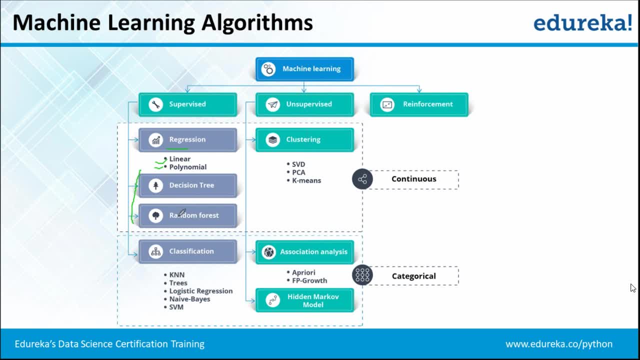 Like KNN, can be used trees- actually This is talking about these trees only- and logistic regression: You can use for the regression name base. again You can Use as we am. again You can use right so many of the algorithm you can find which can work. 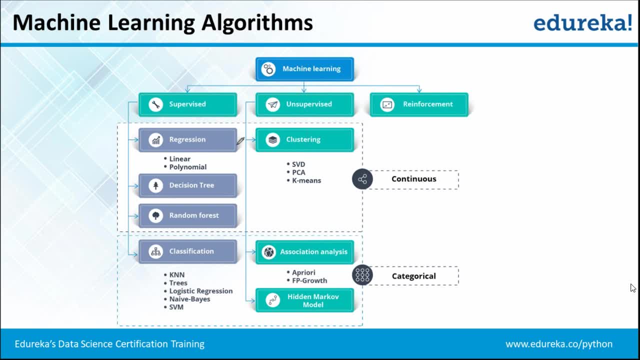 for the regression as well as for the classification as well. When it comes to unsupervised learning, we have the clustering technique. clustering technique is about like we, how do we cluster the items together? So there are different techniques. are there like SVD is there? PC algorithm is there. 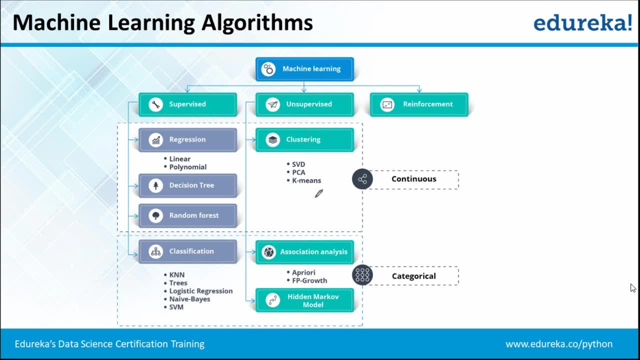 which is principal component, and this is then: K means clustering is there, C means clustering is there, Or we call it as soft clustering. and there is one more hierarchical clustering is there, which is very important, which you guys would be studying from this course, and there are some cases which are also unsupervised. 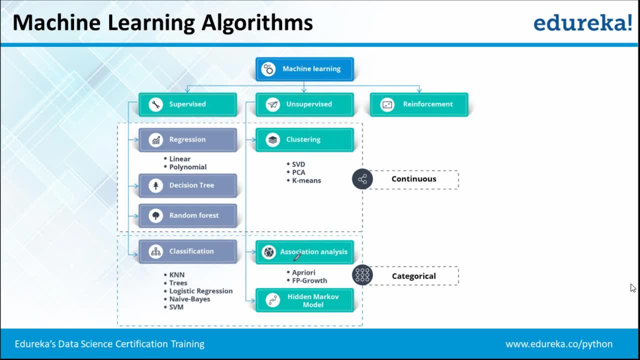 and we call them. it comes under the recommendation system, So Association analysis. there are two algorithms for Association analysis, which is a, probably an F because. so what? for what purpose Association analysis is being used? It is like if you go to the shopping malls, right? 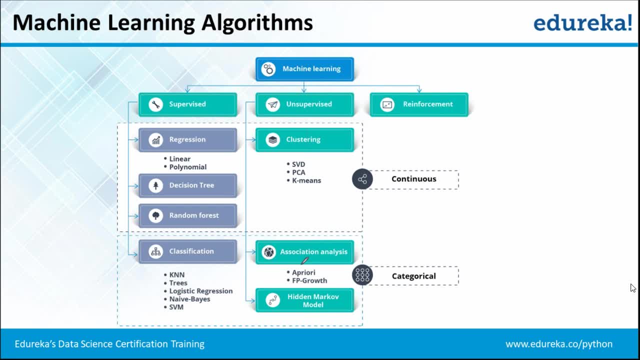 So then you will find the discounts, the way they are keeping the items together in the shopping mall. They have a particular way. It is not like they, they just put the items randomly anywhere, right, But they choose those items very nicely so that items will be put in such a way. 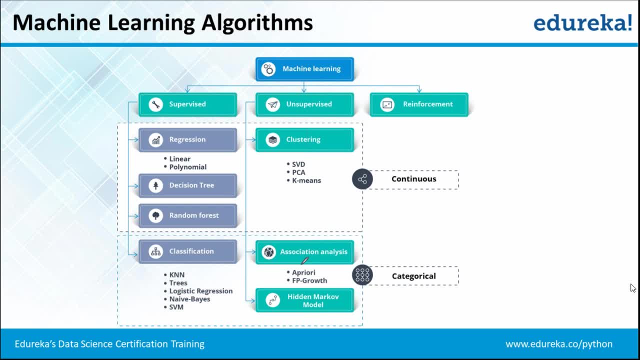 so that they sell, can increase, Right. Let's say you go to the shopping mall to buy the bread, right, and you didn't think to buy the butter already didn't come to your mind that I should buy the butter. But when you are buying a bread, next to the bread you are seeing the butter. 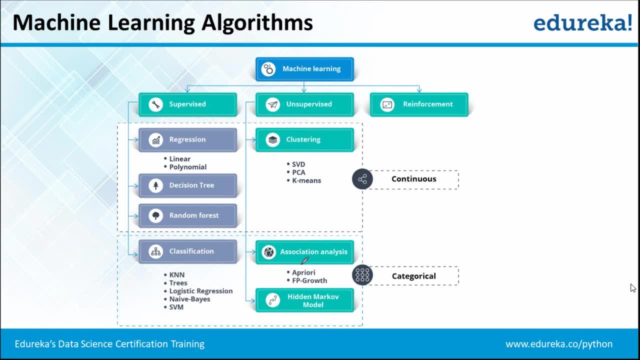 and then suddenly you get the taste of butter also and you think to buy this butter Also, I need right, Otherwise you might not buy the butter and go back just buying the bread. So they are finding that which items are associated with each other. 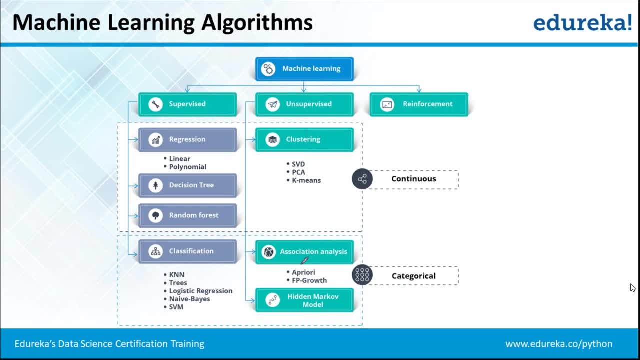 or which can be pulled together right, And then that is what helping them in putting them to increase their sales, right, And not only this thing, that is how, on the basis of they are bringing the offer That you buy this thing at this thing, or combo offer that much percent discount. 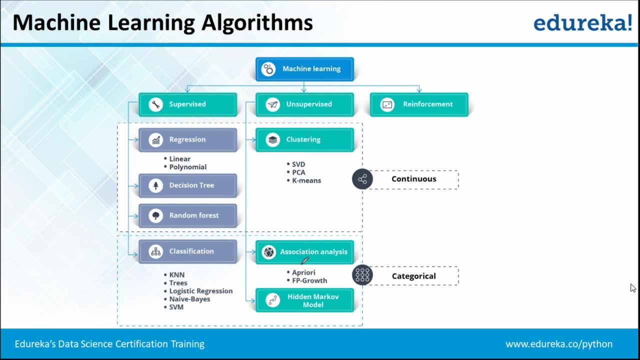 right. They look exactly what can increase their sale of the profit and only then they take the decision. So this is what we call as the association analysis. So this is what happened in the shopping malls. We have one thing here is not written actually: that is the recommendation engines. 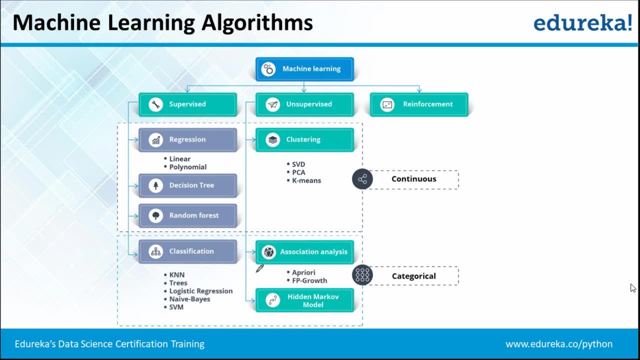 right, So you guys would be learning also recommendation engines, how you can make a recommendation engine. So what is the difference between recommendation and association analysis? association analysis: This is doing in the mostly in the physical stores right of physical shopping malls. Why recommendation engine is being used for for online shopping cart like Amazon, Flipkart. 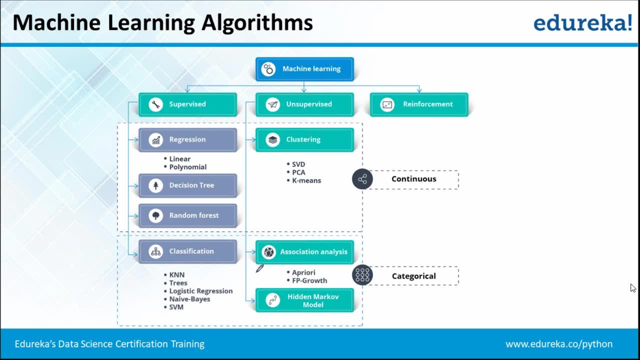 such kind of things places right. That is where recommendation system is used. So why a different kind of algorithm compared to association of? why we cannot use these? because your recommendation we have more freedom, right? We can If different recommendation to different user, right by looking exactly the requirement. 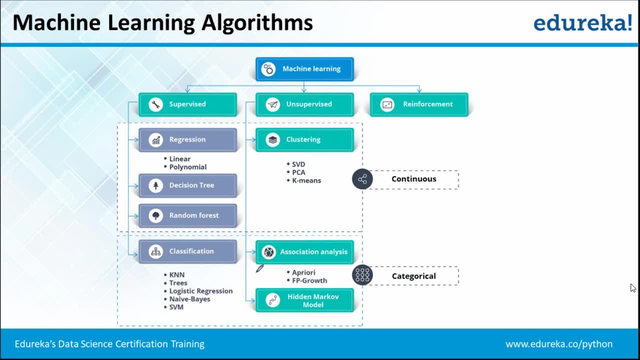 of each user, because for each user we can design a specific or particular web page can be designed on the basis of user requirement, right? So you might see that for one user, the, let's say, if you are watching a song on YouTube, the annual sense watching a particular song and the same song is being watched by your. 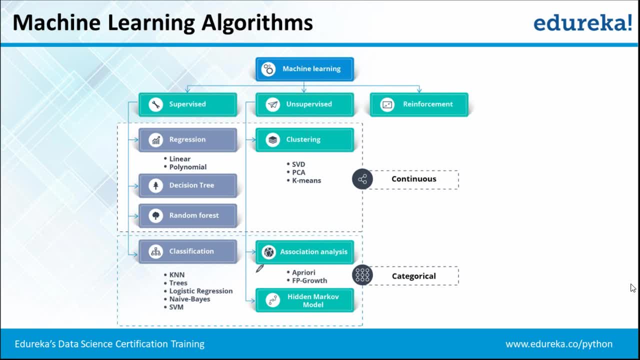 friend, and the chances are there also that the next song which is coming into both of your recommendation might be different as well, right? So this is something very important. So Kadri is asking: can you show us practical please? Yeah, for them, We will be doing one by one today. 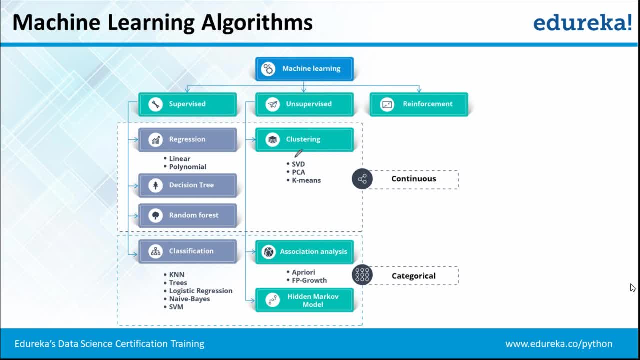 We will be seeing linear regression, practical right, and as the further classes will be going on, you will see other particles. Then we will be having hidden Markov model as well, and then we have the reinforcement learning which I already told about right and hidden Markov model. 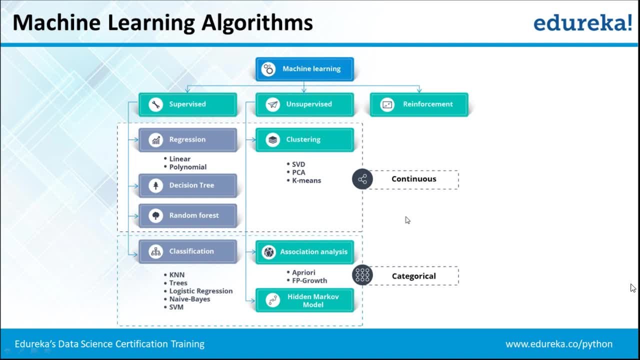 You can think: when it depends on the state, right, if something this is happening, then another thing will happening. and when this thing happens, some other thing happen. when there is a chain of rules that may have been used, the hidden Markov model, or actually there is a states diagram. 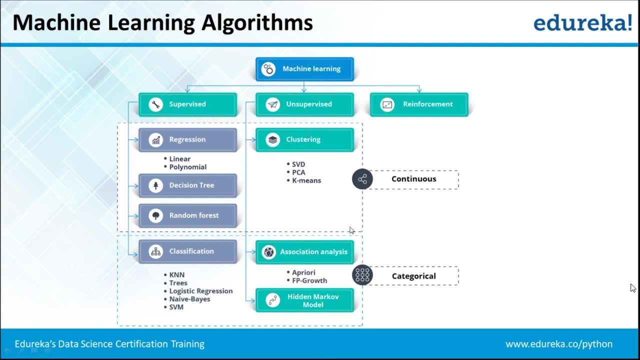 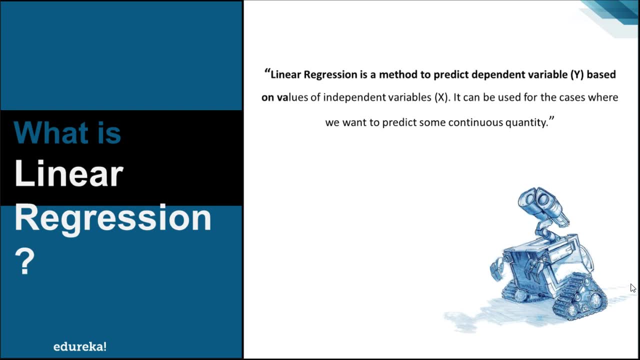 So we will be just keeping it. I will not talk much about here because in a small time it's not possible to discuss it. So we will have the demo related to linear regression in this class. but let's study about the linear regression first of all. what is linear regression right? 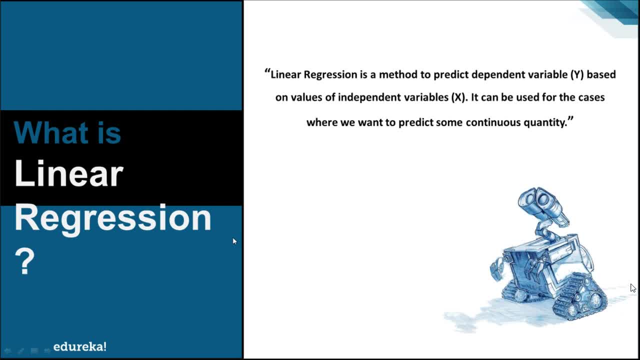 So regression, you guys might have understood where we are saying. the output values might be. output values could be infinite, right, So it can take infinite values, right, possibilities are infinite. What is the correct value would be one only right. So tomorrow, what would be the temperature? is only one. that is maybe I am talking about. 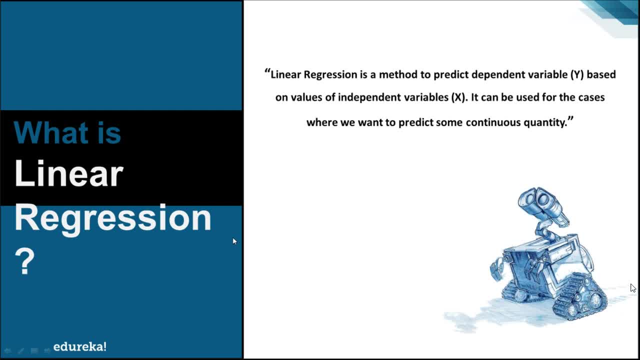 that's a particular time period, and what would be the temperature at 11 am Tomorrow? there would be only whether it would be 28 or 27 degrees Celsius. Let's say only one value is possible, right. But if I say 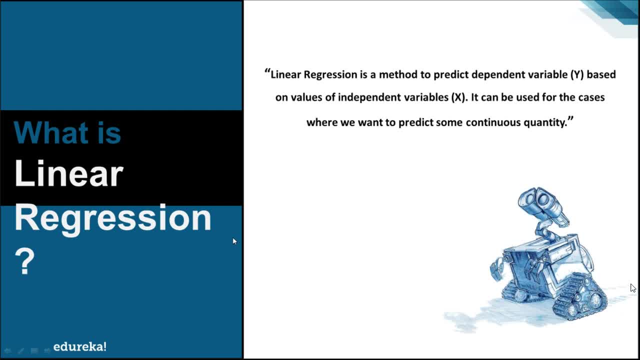 Let's see here What is the possibility? So, infinite possibilities. I can say it might be 20 degrees, 20.1, 20.2 and so on. right, So what linear regression is exactly is? it is a matter to predict, dependent variable. 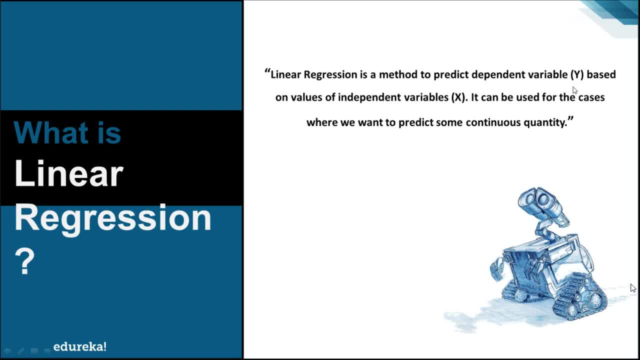 y. So what is dependent variable Why we are calling as a output variable? or in this case we can say temperature, Let's say based on values of independent variable X, right? So some values are given, like X, on which we We can say that Y is dependent, right? 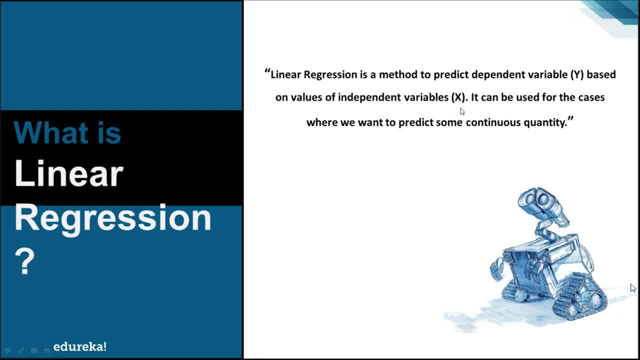 So that is we call as a input variable actually, or input values are there. Let's say what better today, What is the today's humidity and what is today's wind temperature? on this depends What would be the tomorrow temperature, right? So in this case, dependent variable by would be temperature and today's humidity. 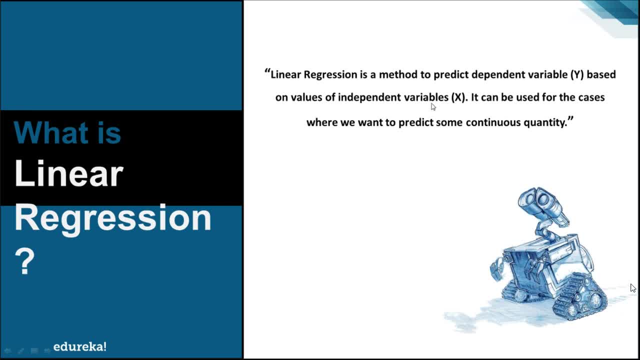 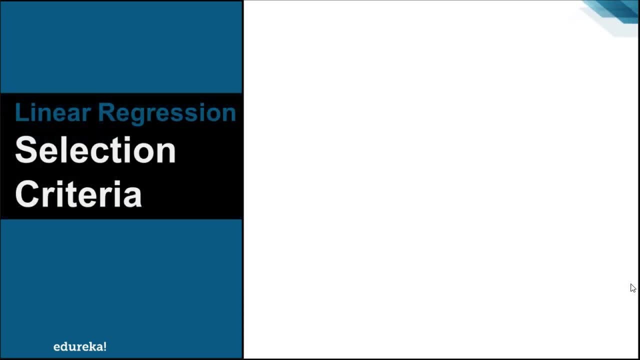 and wind speed would be my independent variable. or we say X, or we can say it as a input variable. So let's see. So we have classification and regression capability. So we'll see quickly you go, rather than discussing this thing, will see where is linear regression. 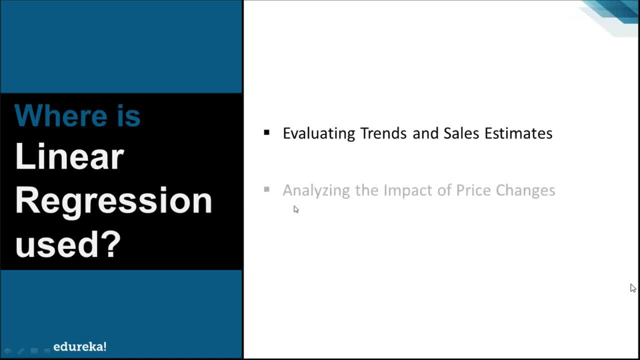 you right. So we will just make it short way so that we can do the practical server, So where it can be used for evaluating trends and sales estimations, analyzing the impact of price changes, assessment of risk- In fact Risk in financial services- and insurance domain right. 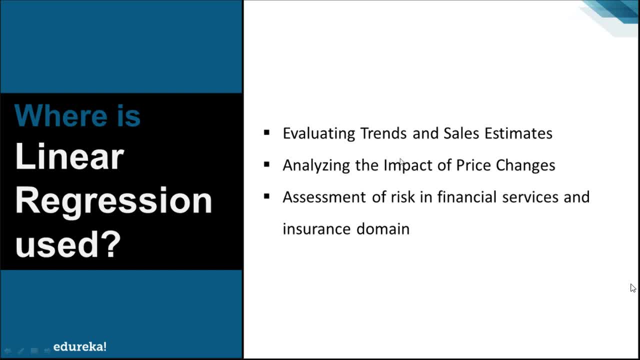 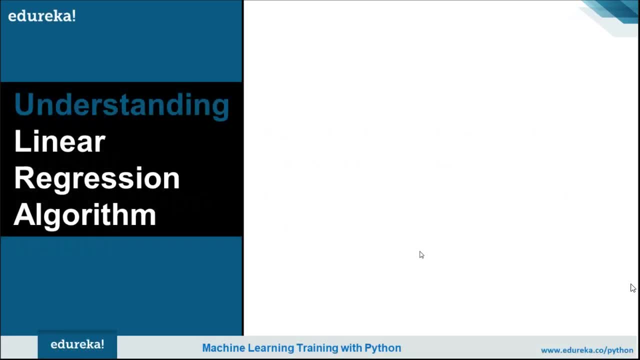 So these are the few places where it can be used, right? So wherever output value is going to be anything- infinitely possibilities- We can use the linear regression. So let's understand linear regression. How does it do actually so linear regression? if you have to think, let's say if I am talking. 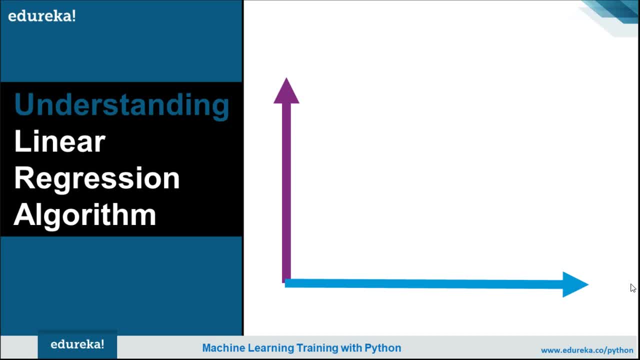 about, there is a one input variable or let's say one independent variable, that is X, right, and the one output variable, Let's say this is a Y, That is our output variable, right. So input variable acts output variable by, let's say, X is my today's humidity. 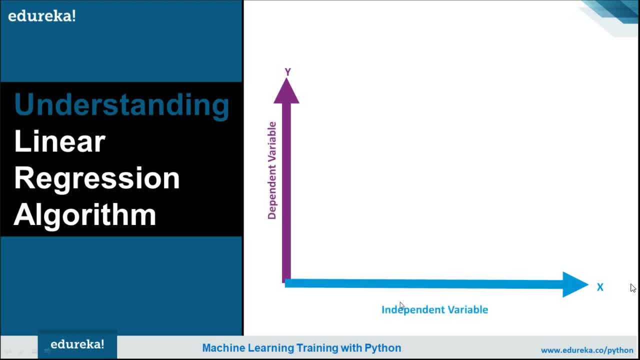 Why would be my tomorrow's temperature? Right? so this is so. we are keeping it very simple by saying one input variable, because for visualizing, it would be easier for you guys, right? So you might be looking for the path in the past. what happened, let's say, when this was. 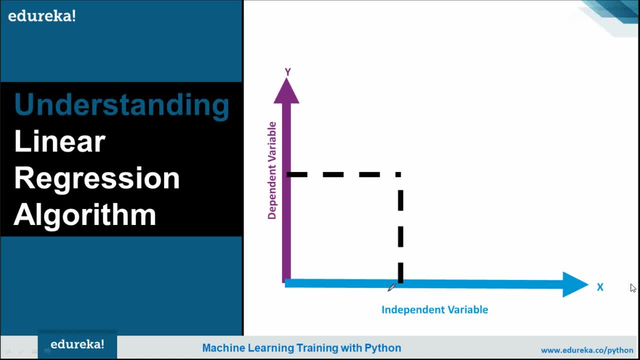 the input variable value, right? So I will just take this thing. then this was the input variable, That is, the X value, then Y value. was that in the past case right? So when the X value, let's say 23 humidity, then the temperature was, let's say, 27 degrees. 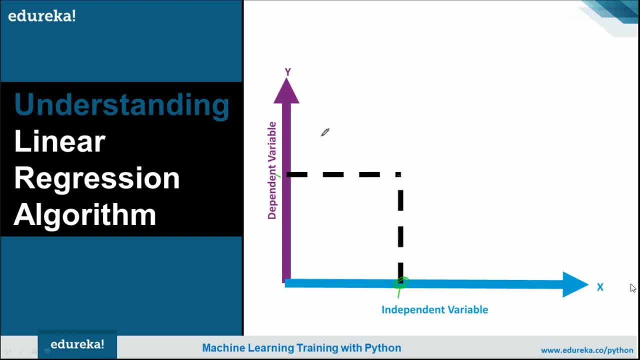 Celsius right, So this become a point. So if I have to define this point into this two dimension, then I will be saying: at this intersection it becomes a point right, or one data point is there. I can say: this is, as a data point, right and we, this is a line, we, even though we are drawing. but how this line? 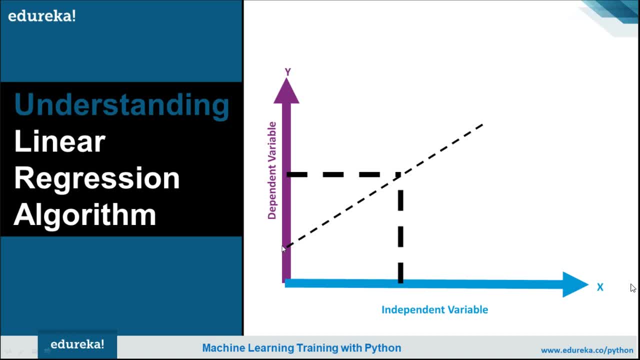 should be drawn is again, You can. I think the another data point is here, right? So, for example, X is 0, when let's say, humidity is 0, then the temperature is this value, whatever, right? So then if you join these to find why a straight line, then you get this straight line using. 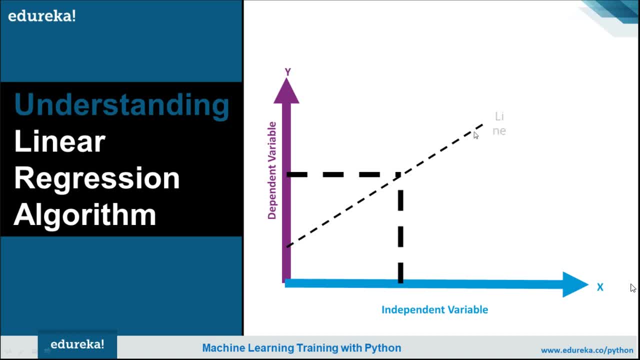 which you can do the prediction further in the future, right? So linear regression is all about finding that straight line, right. linear mean linear, right, So the line simple line. or if you are talking about the plane, it might be, but the plane would be again. 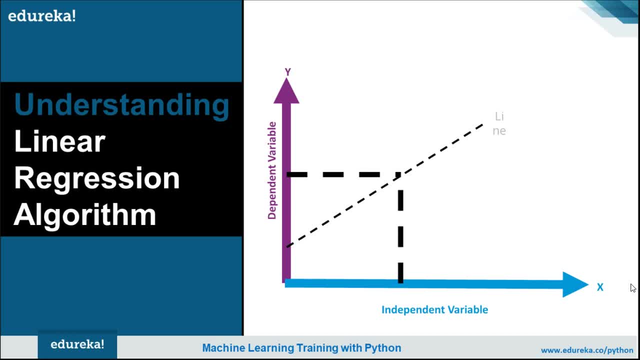 So depending on how many input variables are there, right, We are not saying it would be polynomial, but we are saying it would be linear, right? So here, for example, here from here, if we switch, let's say if I increase this value and it 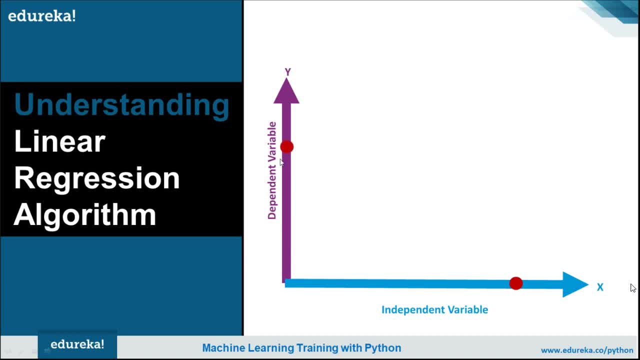 becomes. let's say why this way? right. So it increases from here to here as I increase from here to here. this increase from here to here, They're showing that if you are changing different value of facts by value is changing right. So it is showing. 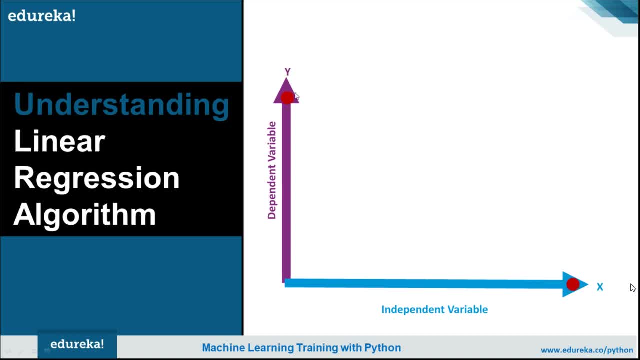 How, when you changing the x value or input variable value, how the output variable is changing, that is, by, and then you, when you try to find out all the changes can be shown by this particular line, right? So whatever early changes we saw, those can be seen by this thing. 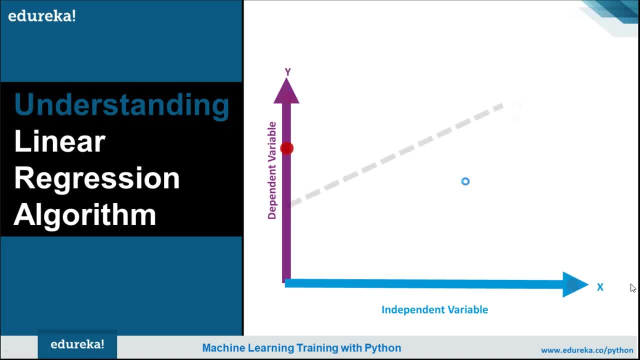 So here we are saying it is a positive relationship. What do you mean by positive relationship? as I am increasing the value of x, y values, also in different right, So we call this thing as a positive relationship, Right? So here, if we increase this value, let's say: and this value decreases in this case, what? 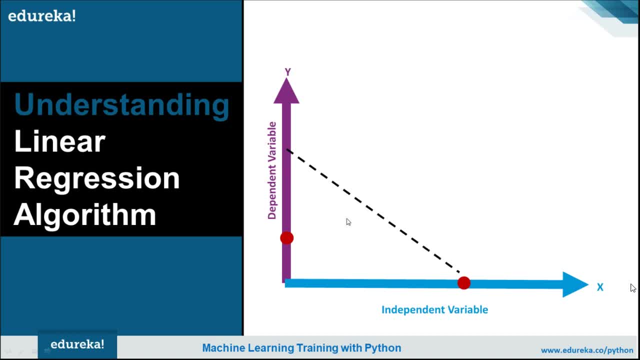 would be happening. then we will say it is a negative relationship. actually said we going to the reverse direction. So you might have seen earlier how the line was going. in one cases line one line was going upside while there was a positive one, and in the other cases that was going downside. 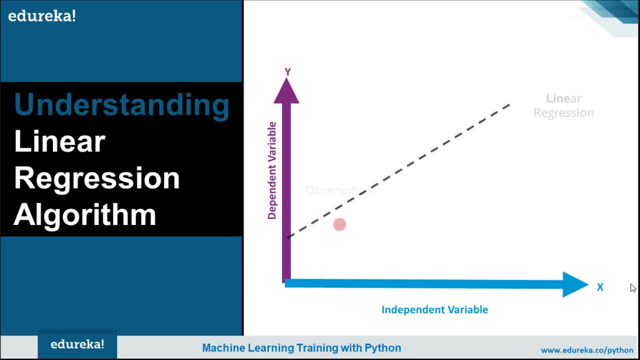 which we say as the negative one. So drawing these lines? No, This is a linear regression, right? So we will be getting the observation. observation is nothing but the data point. Let's say, for past one month, you collected your data set right where it showed that if 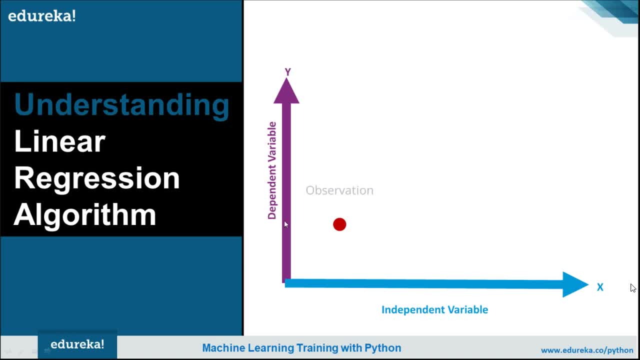 this much is the humidity, that much would be my temperature, right? So let's say this is the one observation of one data point. Let's say it was of, let's say, 20th of September data point. It was that when the humidity was here that the temperature was here, right? 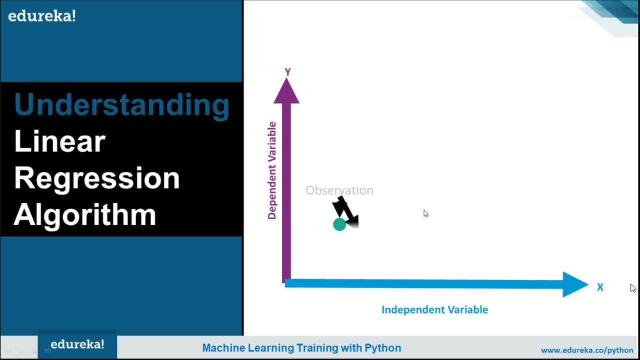 So this is the one observation of one data point. So this is the one observation. find you say, and let's say: this is another data observation point. So, as you, you see, this is showing when the humidity was this much than temperature, because this much right. 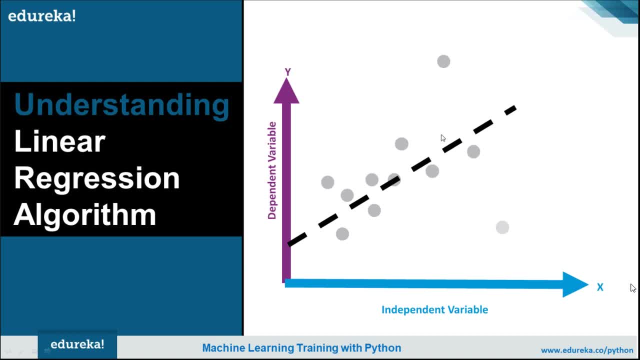 So what do you start doing? is you basically start taking all the observation, right? So let's say, this is a data point, These all circles are defining a data point, right? Then you try to find out a line which can go through these data points. 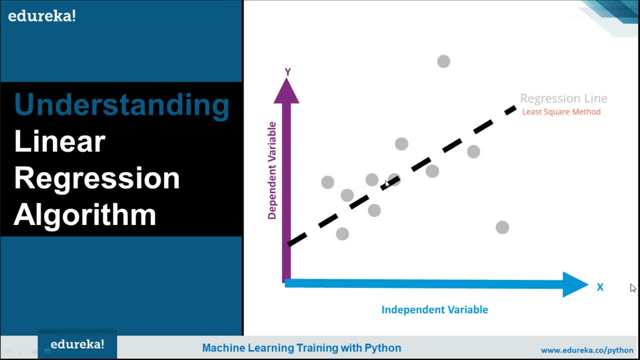 But you will see, it is not possible to find any line which can go through these all data points. So what you will do, you will try to find such a line which can go through maximum data point or, if you find out the, how much away these lines, these data points, are from the line. 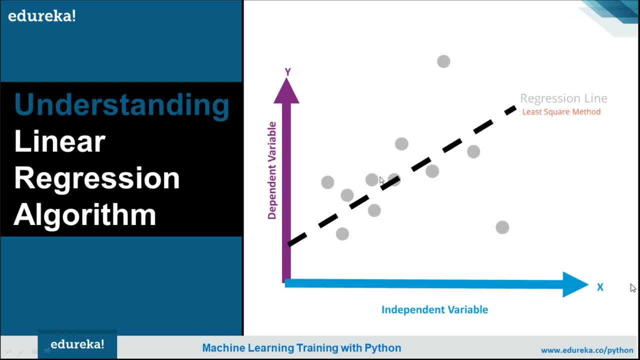 It should not be much far away from the line, right as close as possible data points to the land. It would be good, right? So we call that the error should be less, or the error method which will be using is the least spare method actually right? 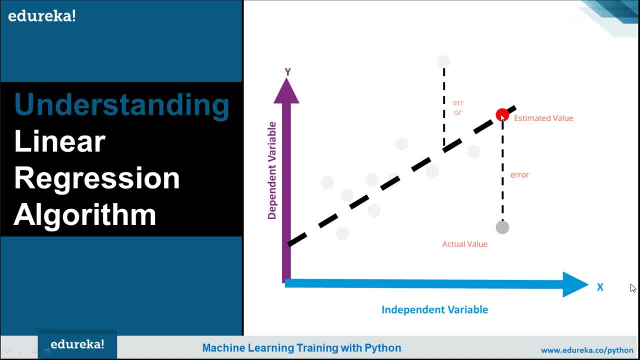 So let's say this is the estimated value, right? Let's say so what we are showing here, in reality, this data point is existing here, right? So when the x value is this in reality for this data point, y value, is this much right? 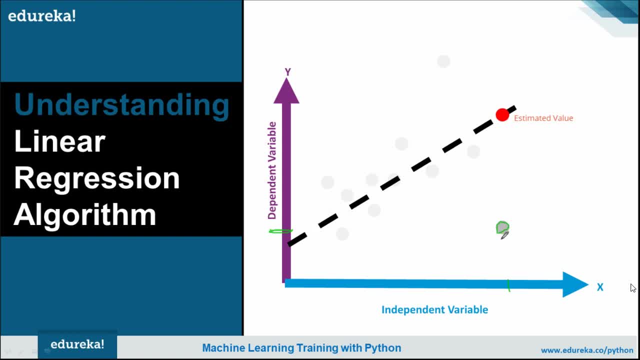 But if you are going to use this line to estimate this value for the this output, so what you will? If somebody say: okay, this is my x value, then because you are using this line to predict this value. according to this line, when x value is this, then y value is going to be this much. 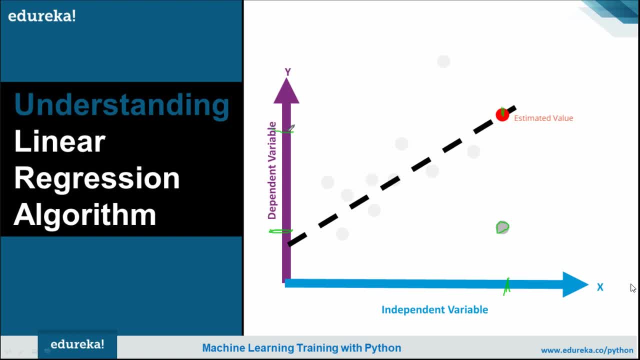 right, or here it will be showing So- how much error it would be. that much error is there into your data point, right? So this is what we are going to see here, right? So you see here that much error we have into us similarly for this data point, that much. 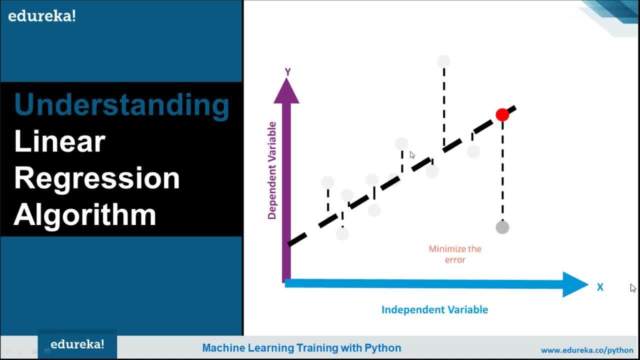 error. So for each data point We calculate: Okay. So basically error right. so for this, for this, for this, so far, this it would be 0 for all we find right. So here it is very less. So we will try to find such a line which can minimize the error, right. 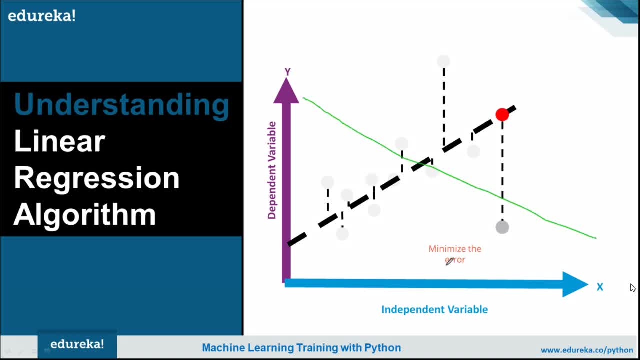 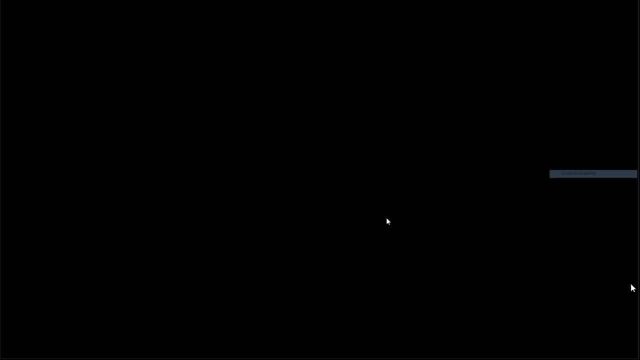 So we can have many, many lines, right. You might say, why not this particular line, or why not this particular line? right, many lines are possible, but you will see, the one which we are looking is which can minimize the error, right, So we need to find out the way which can minimize the error. 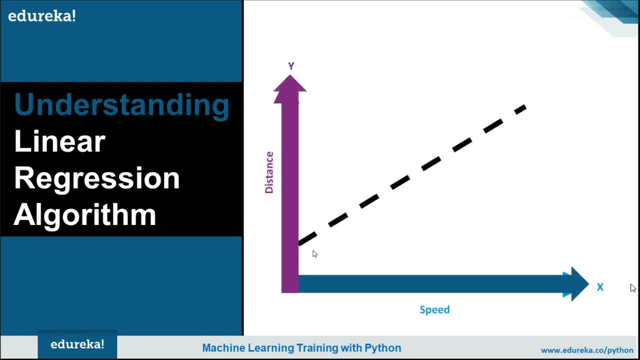 Okay, so here they are showing we can think that it might be anything, right? So, like it might be speed or distance, just showing the relationship for the equation. Let's say so What would be the line equation? line equation is always if you're talking about one dimension. 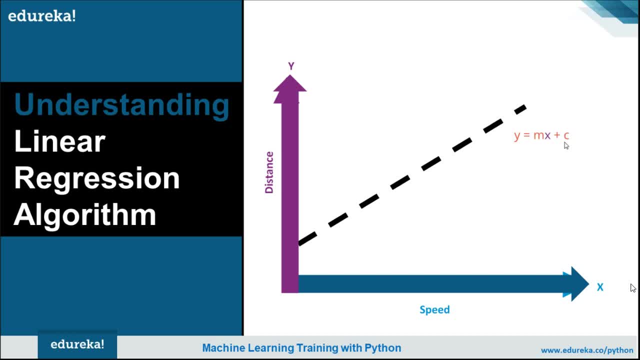 Y is equal to MX plus C if we are talking about two dimension, which becomes Y is equal to. if we are talking about three dimensions, where we have, let's say, two x values, right, or two input variables and one output variable in this case, So you will have, Y is equal to m1, x1 plus x2 plus C, right. 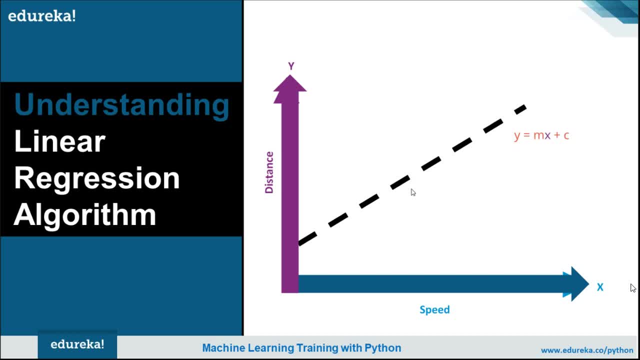 So this is an offline equation, you say, but this is line equation. We are getting only one, one input variable and one output variable. So here this is Y intercept right. So what is this? C is defining. What is the Y intercept right? 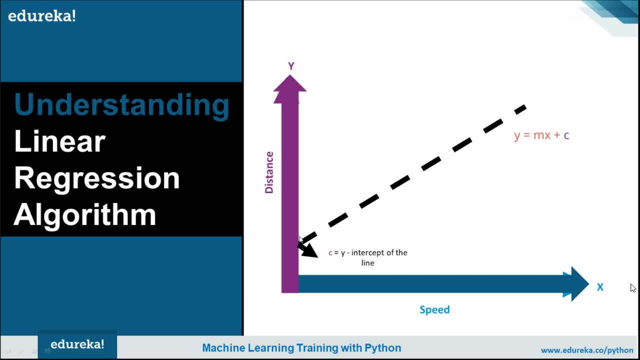 And what is this? So we, what is Y intercept? You guys might be knowing already these things, Okay, From your 10th class mathematics, if you remember right that in equation Y is equal to MX plus C. C basically tells where this line is cutting or intersecting the Y value, right? 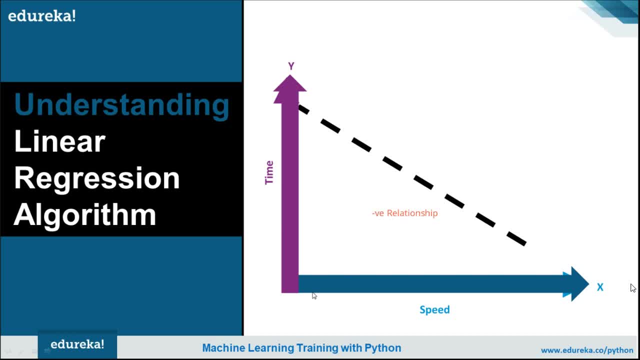 So if we have this kind of line, then we will say negative relationship, because as we are increasing the value of X, the Y value is decreasing, So we call it as a negative relationship. right, and here, when we have such equation, In reality slope value would be negative actually, right? 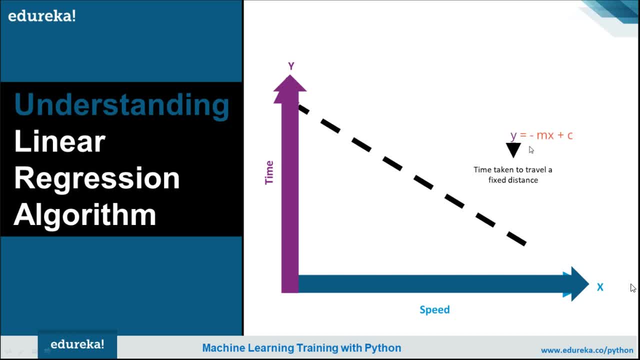 So if you take M as a positive, always that this negative would be there, right, depending how do you take the app. so I am defined the slopes right. So in the earlier case also it was defining the slope right. So here, but if in this case slope value is positive, right. 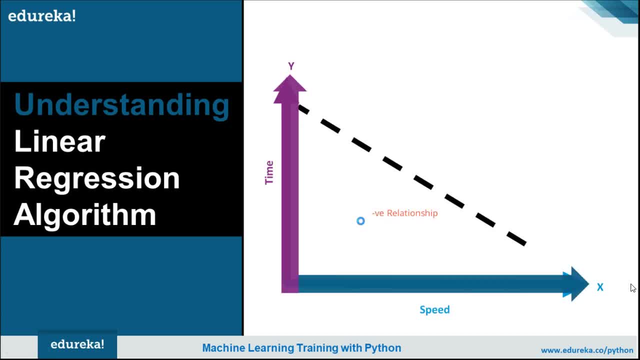 It is increasing because. but while if you see, in this case slope value is find as a negative value, right, But you doesn't need to write two different equations. as such, You can write Y is equal to MX plus C directly where and can take negative or positive value. 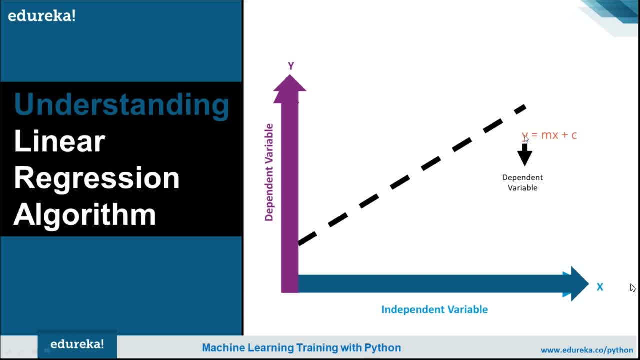 Right. So this is the way things are. so why is our device nothing but the dependent variable right, which is our temperature? X is nothing but our independent variable. Let's say, this is our humidity right and C is intercept. So for finding this, so data points is given. 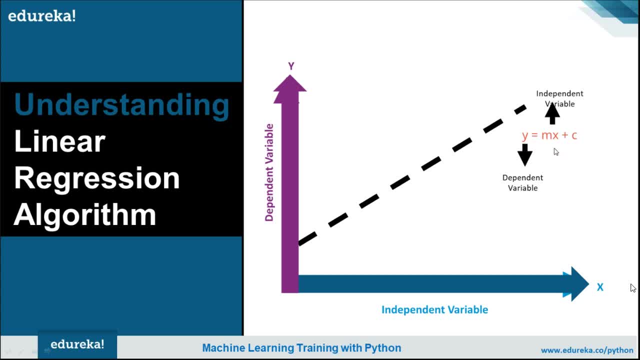 So, in reality, what we need to find is what is the value of M and C, right? Somebody will give us X value and we will be predicting What is the Y value. if I meant C, value is given right. So if we can calculate now I meant C- and then whenever X value would be given to us. 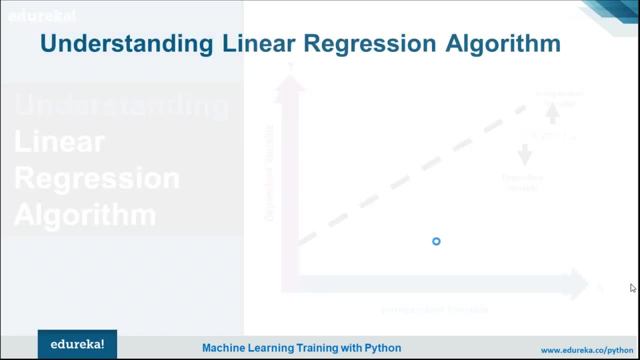 We can do the prediction here. So let's understand the linear regression. Let's say: these are the X values are given to us, or input variable values are given to us and corresponding to them, these Y output values has been given to us. It's so we can draw. 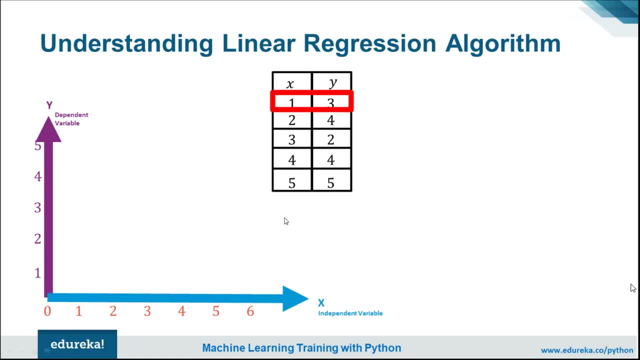 Each of these data point, right? So we are taking first, first data point, which is 1: 3.. So if you draw here, one is here on x-axis, 3 layer on the y-axis. So this become our data point here, right? 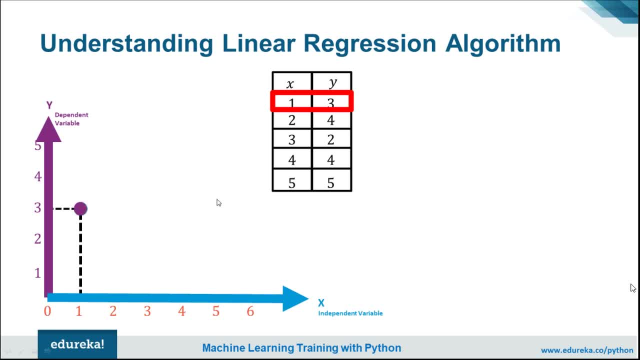 So here it becomes our. this is our data point, right? Normally we got one data point, 1, 3 would be here. Similarly, we will put all the other data points as well, Right? So 1, 3 comes here. Similarly when we draw all the other data points. so like 2, 4, we get here, right? 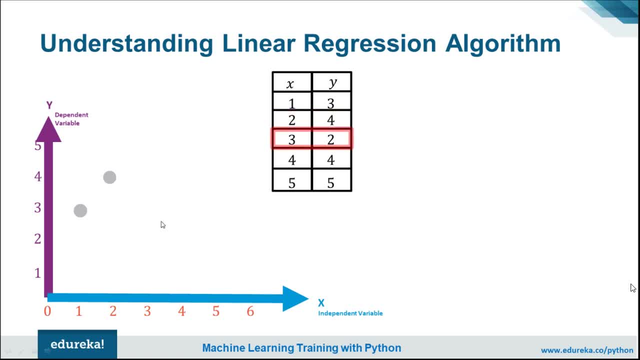 X value is 2, Y value is 4.. Similarly, we get the 3, 2 next which is coming here, then we get next 4, 4 coming here, The next 5, 5 coming here, right? So these are the data points, right? 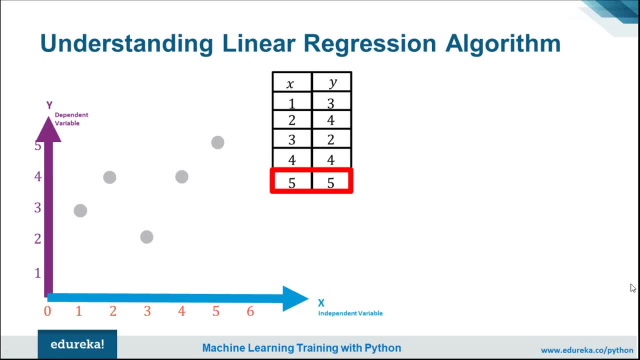 So this is the data point has been given right. So this is the input value that has been given for the from the past and what was the corresponding Y values given from the past. So what we want to do is we basically find out a line which can go through this. 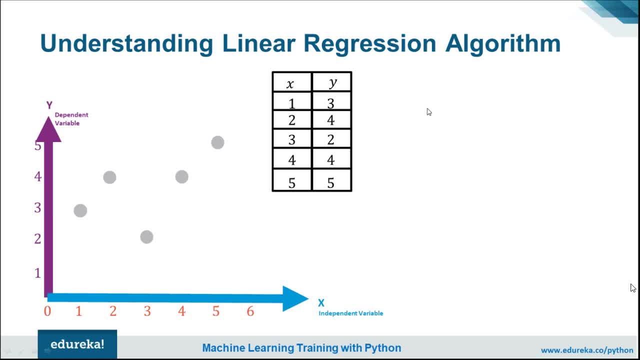 So Kadri Hassan is saying: it's looks like variable chat. Variable chat means: Are you doing it on the fun part or like what? You have a query here, Okay. so if we doing Okay in physics, Okay, I okay. 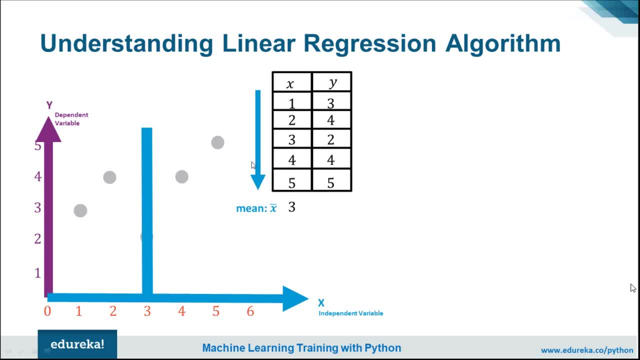 Okay in physics. Yeah, it might happen like this. I don't know about this thing, physics- I'm out from the physics background. Okay, great, So we will be finding the mean right. So on the x-axis, we will find the mean, which is 3, right. 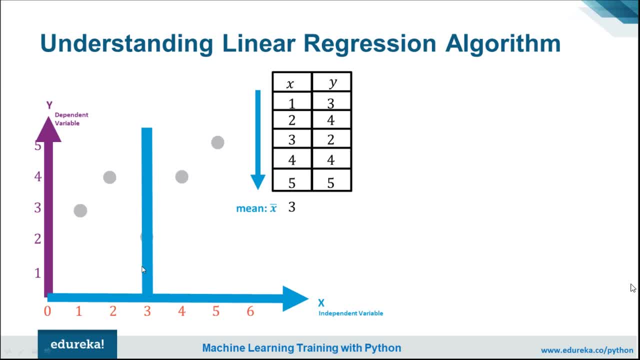 So what we want now, actually, in reality, We want to find out such a line which can be closer to all of these data point as much as possible, So that the atom can be reduced right. So which we are talking about. So, first of all, what we will do, we will find out the X mean. 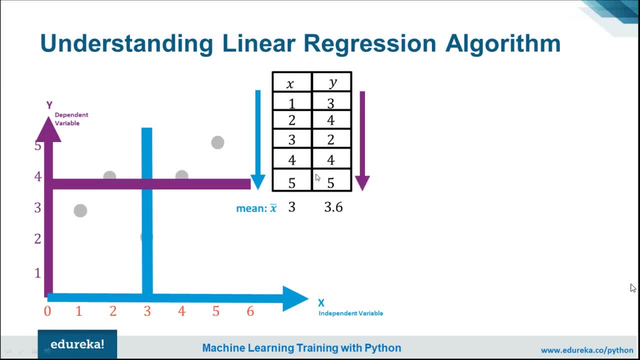 So here X mean we are getting as a 3, then we find out the Y, mean by mean, if we take, it will be: get the 3.6, right, And then the we get this fine. So we will say our line might be going through this particular, this point, that is 3, 3 right. 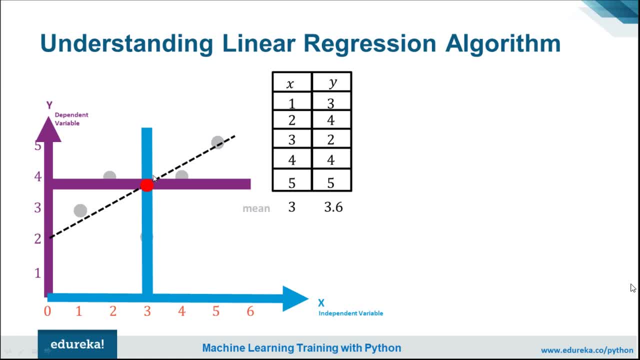 So, but here, how this exactly 9 will go, that we have to see, right. Okay, So here it would be, definitely it would be going somewhere from here, Right? So we call this point as a 3- 3.6.. Then we have to calculate the value of M, right? 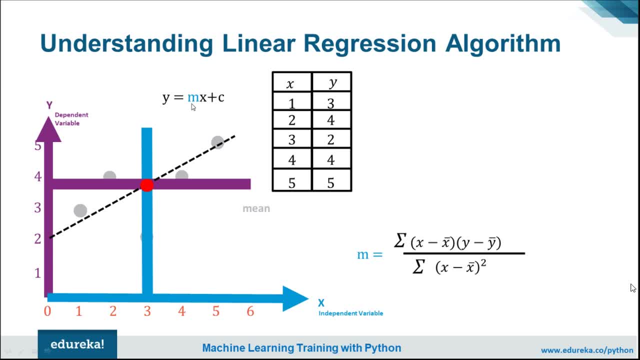 So one thing: we just called the X and Y bar. So how we can calculate the vibe M value? So we need to calculate the M and C value. X and Y has been given to us right, So normally we can if these all are falling in. 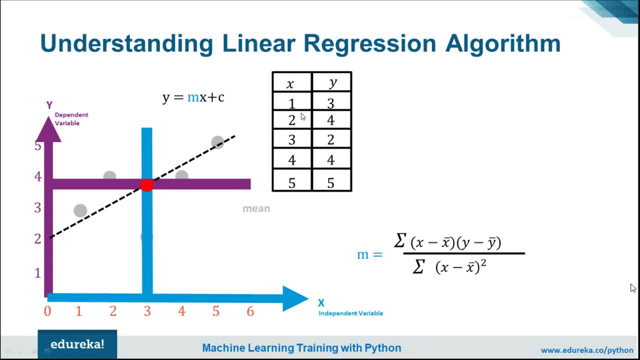 Okay, If these all are falling exactly onto this line, then we can just take two variables to unknown, right, So to data point. we can take, so it becomes to two equations and two unknowns. But here we. these are little bit away from each of each other: patterns. 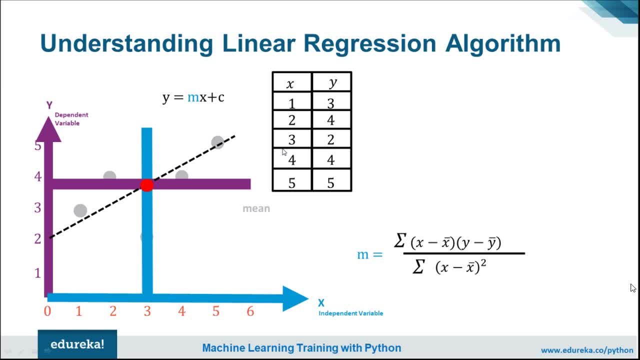 So we need to find a common ground which will be doing it using the mean. So how this M would be calculated is this way: summation of X minus X bar multiply Y minus Y bar, divided by summation of X minus X bar. So there is a whole mathematic behind it actually. 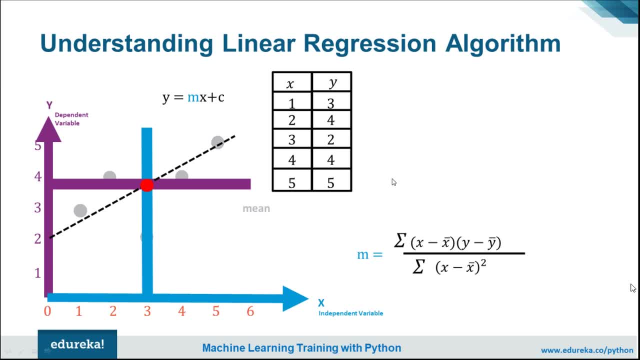 So if anybody is interested, in a short, quick way, I can tell you- if you are good with the mathematics you might understand it quickly- that you basically just think this is an equation. right there You keep the M and C and for each of these x-axis value, put them right, and these are 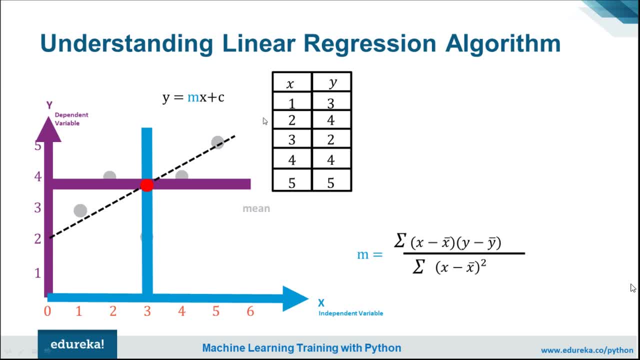 the corresponding Y value and then you take the summation over them. That is error right. How much it is debiting from this? You take it as an error and then differentiate it right with respect to X, and then you differentiate it So it will give you minimum error value. that what you are looking for, but as to keep it. 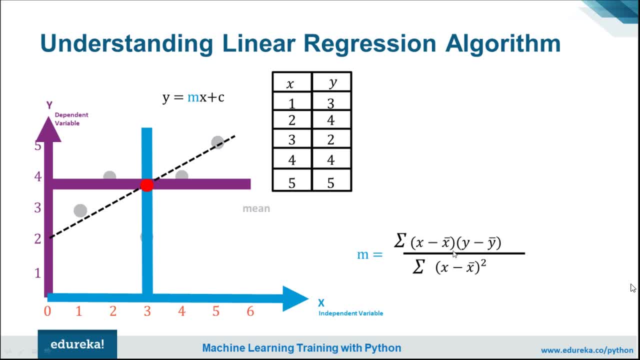 simple currently. you can just remember that for finding out the M, This is a formula. This is what we guys would be doing. So we know the mean for X and Y, that is, 3 and 3.6.. So we need to calculate the X minus X bar here. 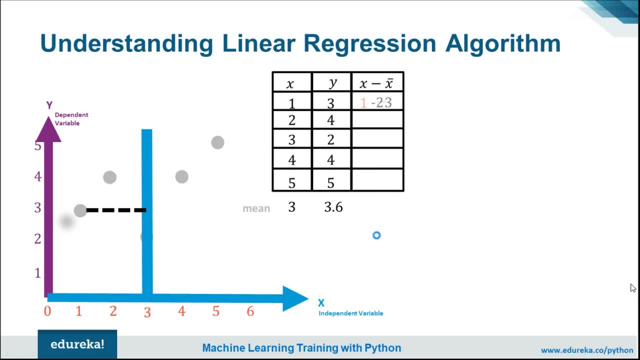 So we do it quickly: 1 minus 3 becomes 2 minus 2, and so on. We do it for all the values, Right. So this way we get all these values in such a way right. So we got X minus X bar right. 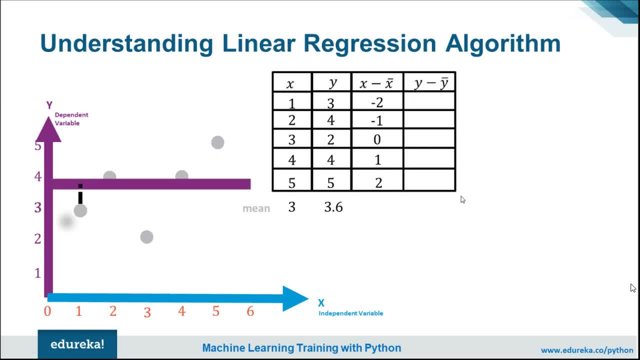 And now we want to take the Y minus Y bar. Similarly, we calculate, So we know the Y. here We have the Y bar 3.6.. So we remove deleted, So this becomes So. there is like little bit editing. 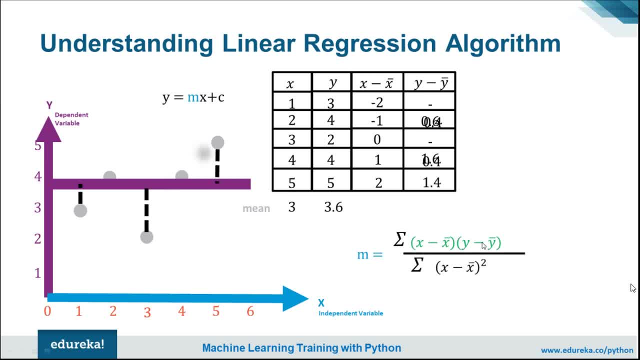 Take care, Right, But I hope so You understood completely. You got 5 minus 5 bar. Then you can get X minus X bar, whole square. So you will be taking the square of all these values, Right, So you get the square. 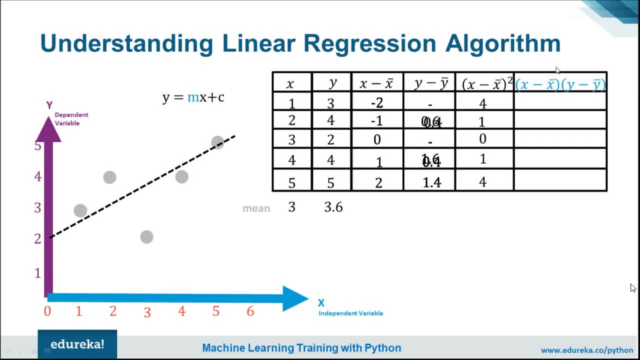 Okay, Done here. We have to multiply both of them right before taking summation. So we multiply them. This is the table We got And we take summation over that. So this is 10 and this is 4. Right. 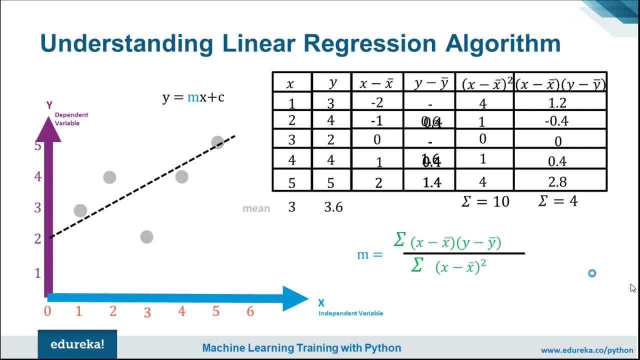 So 10 we get in the denominator, 4 we get in the numerator, So we get here 4 by 10.. That's make it M value as a 0.4.. Right, So we get M value as 0.4.. 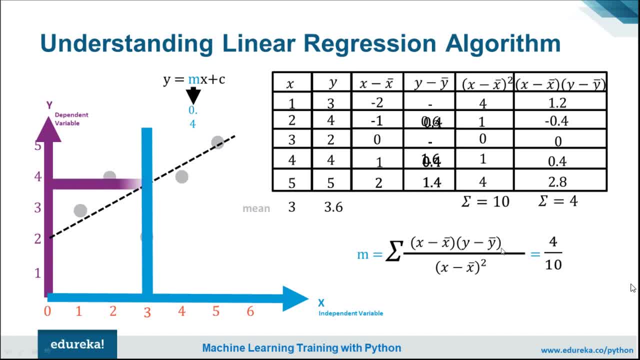 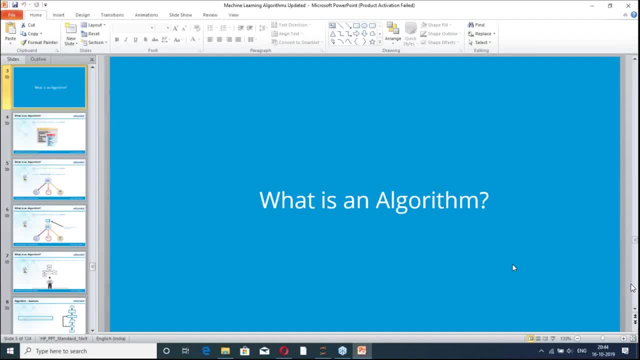 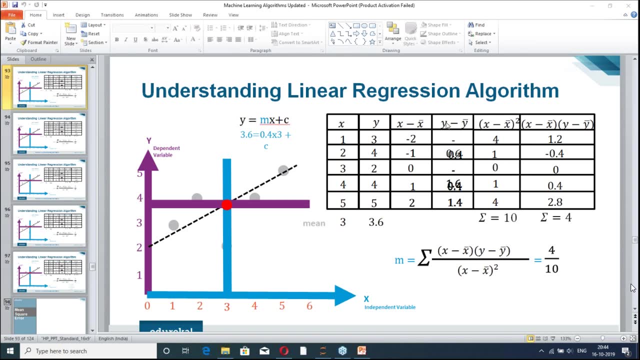 So here, Just take you guys. This is repeating the same thing on this, Just stuck here somewhere. Okay, Webinar is trained- is asking: I didn't understand. the X minus X bar is correct. This is not X minus X, This is X minus X bar. 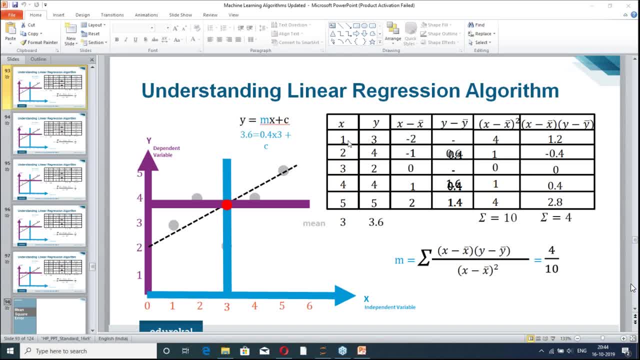 So X bar is the mean of the X, Right. So X value is this, Let's say 1, and X bar is this 3, which is mean here Right. So it is equivalent that I am subtracting from 1 minus 3.. 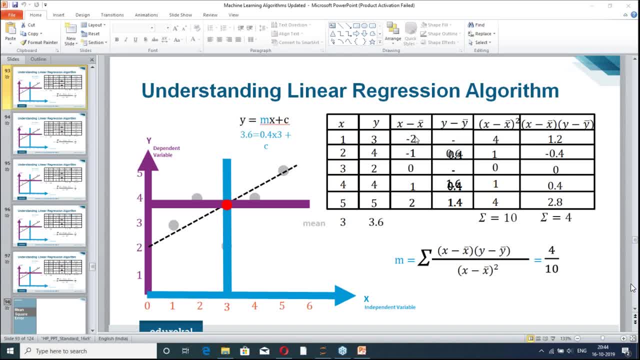 Right. So that becomes here This: one minus 2.. Right, Then I subtract. for the next row I take 2 minus 3.. Then it becomes minus 1.. Right, 3 minus 3.. It becomes 0.. 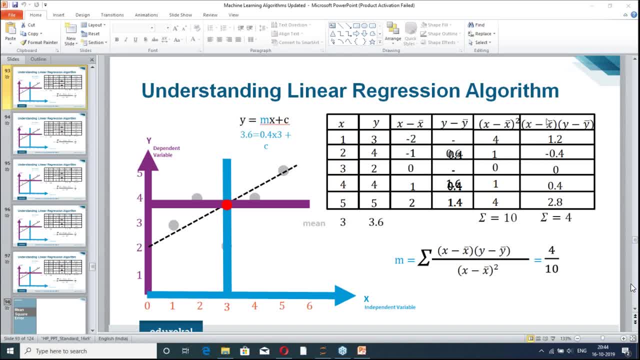 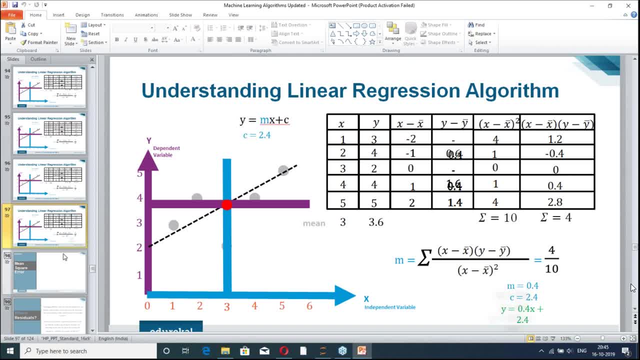 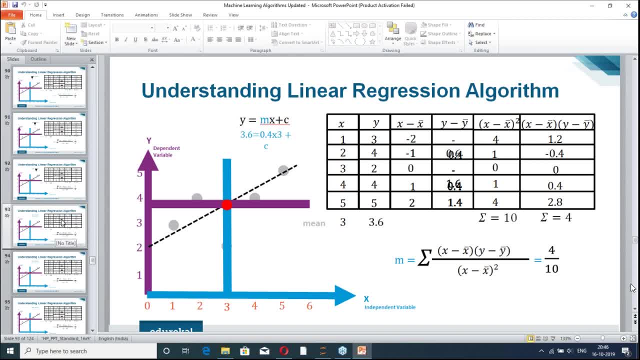 of the axe. similarly, we can put the five mean, which is 3.6, and then we get the c value. this way, by putting all these values, that is we get here. there seems to be some question. i will be taking in a second. that makes c is equal to 2.4. right, so we get the equation. so jaggery akhil is. 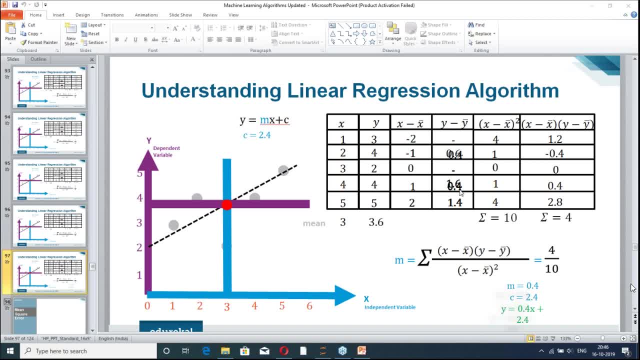 asking: can you share this ppt with us, sir? um, i am not authorized to share it, but i think you might have the support number of the uh support contact number or maybe email id of the adjudica so you can request them. they probably will share it with you, right? so i don't have any medium to. 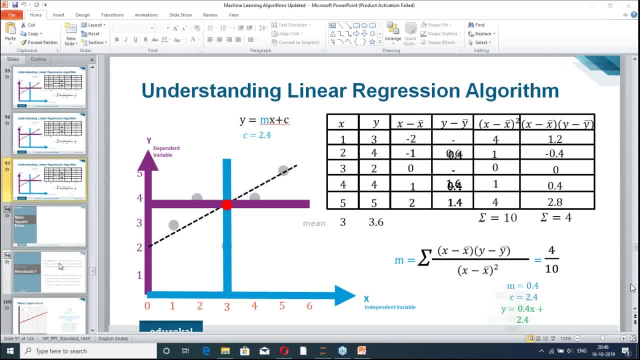 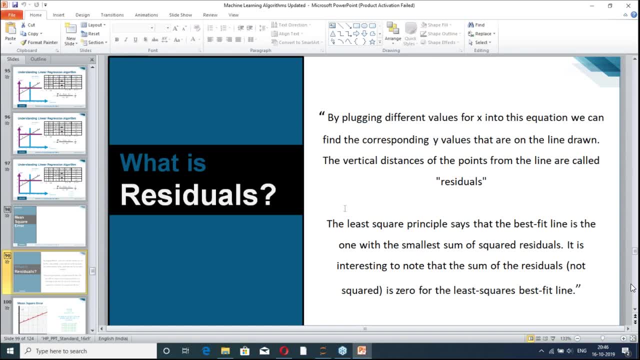 share here as well. um, they can share it with you, so they are the authorized person to share it with you. okay, so let's talk about the means. right, so we need to calculate the error, right? so for that we need to, we can use different, different measures, are there? so one measure which we are finding is mean square error? 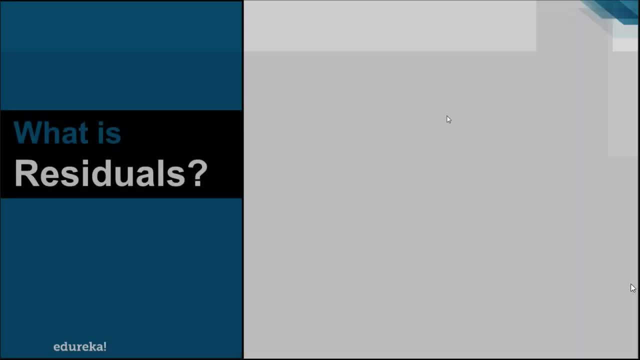 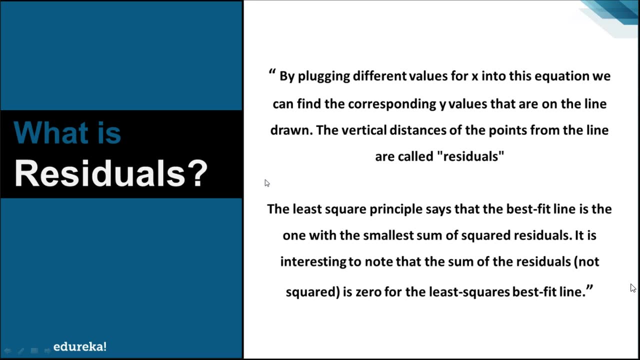 so by plugging different values for x into the equation right, so by plugging different values of x into this equation which we have calculated, we can find out the corresponding y values that are on the line drawn right. so we are predicting some values and in reality there are some values. 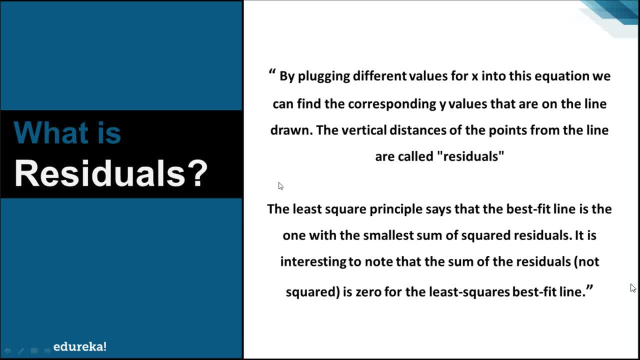 right and anytime it might be possible, the value which we are predicting might not be the correct one, right? so it might be somewhat deviated. so how much it is divided from the correct value, right? so let's say, if the correct value should be 28 degree celsius for tomorrow's temperature, and we are 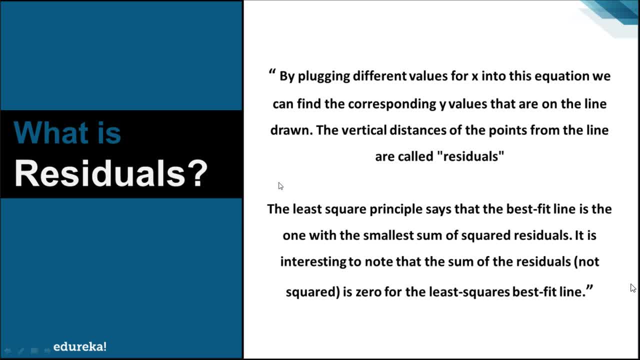 predicting as our 27.5 degree celsius for tomorrow temperature. so it means there is a 0.5 error, or we can call this as a residuals. how much? uh, we are not predicting it correctly. okay, so there least square principle says what we are looking for. then we want to find out the best line, right? 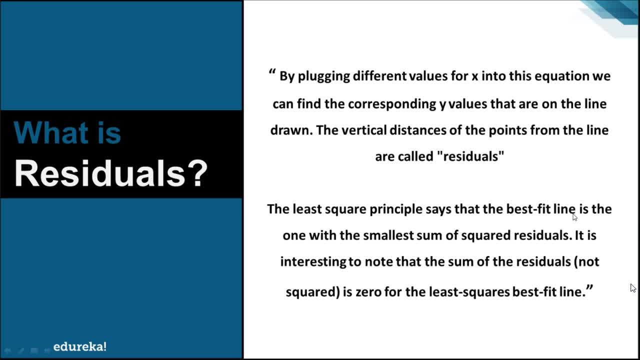 so best line where this error, if i add all these errors together, right, and then its sum should be minimum, right. so that is what is going to do, and when we say least square principle, we are basically talking about that particular line, uh, which gives us error, and we take basically some. 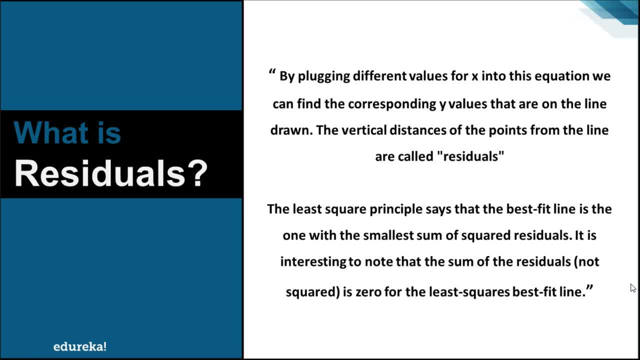 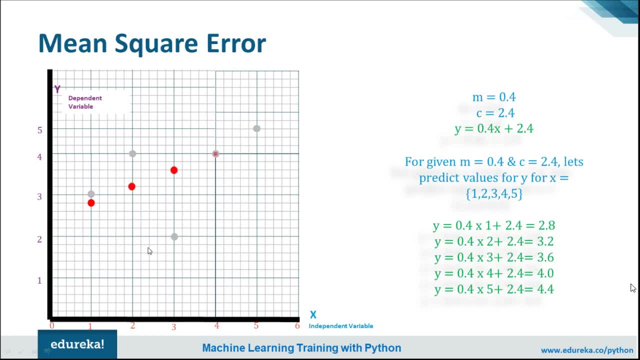 of those errors, right, and some of those errors should be as minimum as possible. so here, in this case, if we calculate the mean squared error, right. so we have all these data points and these are the predicted. one red color are basically showing the predicted values and the real values. are these one right? so basically the error is how much distance is. 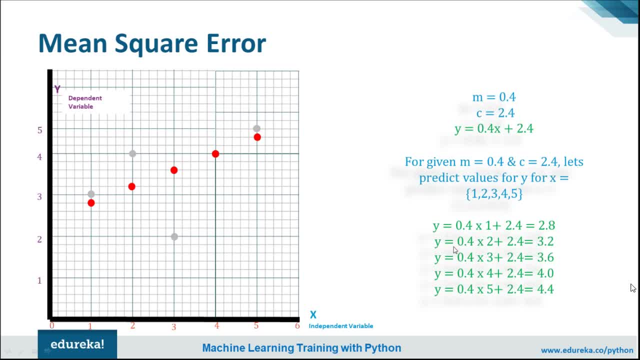 there and you take the sum of that right. so this way you can see the equation which we found was: y is equal to 0.4, x plus 2.4, and for this x value is one. so what we will predict by value is this: 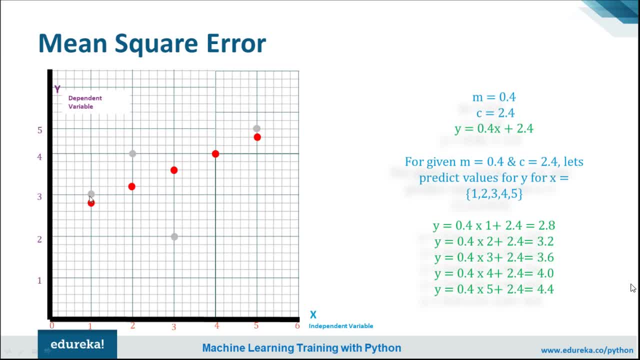 month, that is around 2.8 and the real value is 3, actually right. similarly for other, we see what we are predicting is 3.2. for other also, we are seeing what we are predicting here, right. so this way, we look for each one of them right, and then we calculate the distance between them and that is. 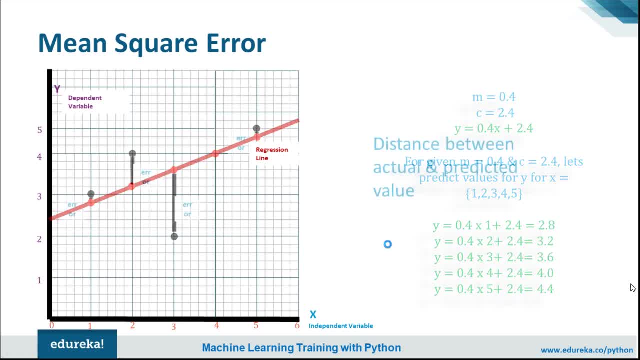 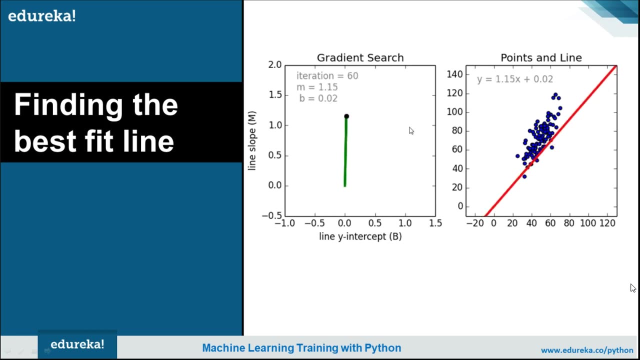 what we are call as a error actually right. so that much error is there. distance between the actual and the predicted value is known as the error right. so here you see. so this is gradient search. how do we find right? so it is showing. so if I will take 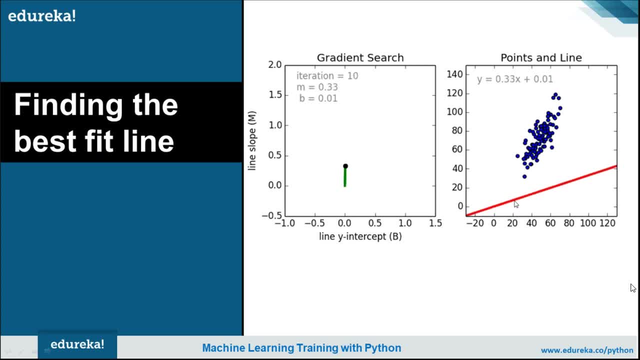 you again from this way so you can see it is trying different, different M and C values and, as it is doing here, you can see here it is coming coming. these were the data points. so it is saying what is the different value for M and C? it is. 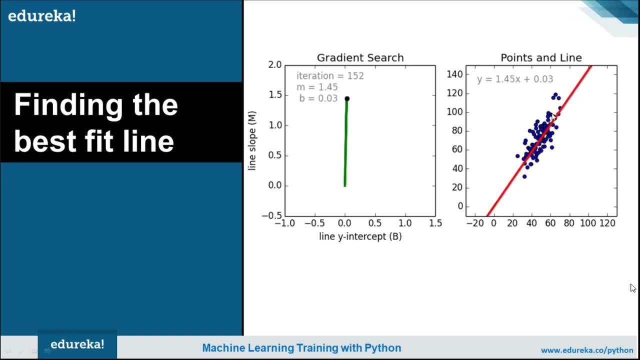 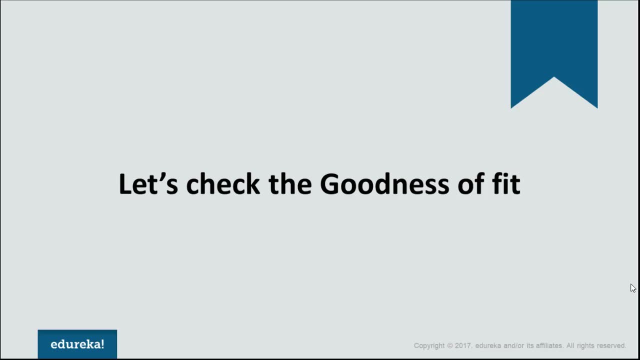 using and when it reaches to some particular place, then the error would be minimum right. so this is a particular red line which we are getting here. for this case, our error would be less right. so you can use the method which we showed or you can use the. this is gradient search. 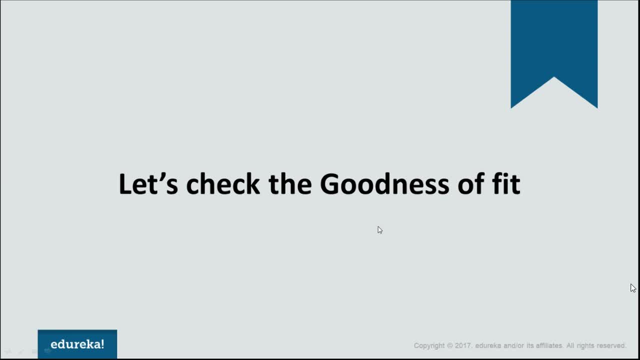 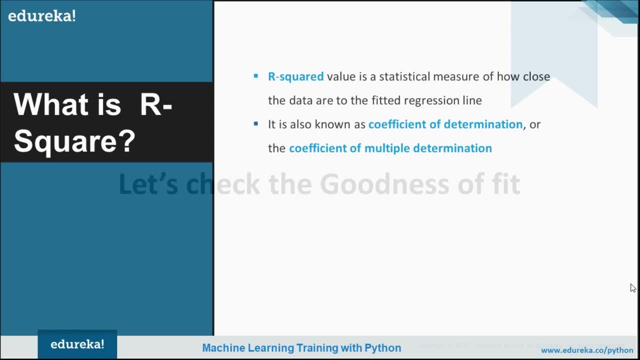 method actually, which we are not able to talk here, but because we have to do some, some code as well. so let's keep it quick, face. and what is the other measures we can use? so one is definitely: you can use the mean squared error, right, how much the 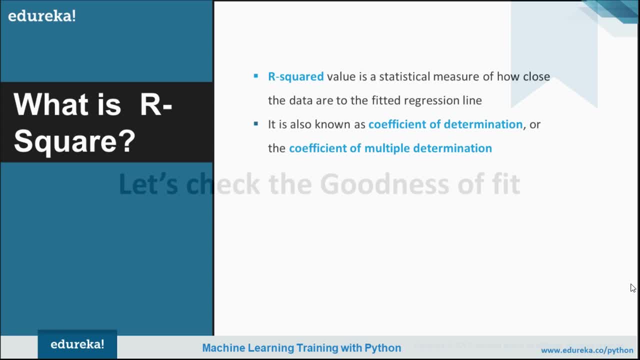 when you conduct the test right. initially, I told you one thing: that you are teaching to your machine, right? so machine learning techniques, that is why. or your software. you can say it is learning from the data you gave the data to your machine, right so machine learning techniques, that is why. or your software. you can say it is learning from the data you gave the. 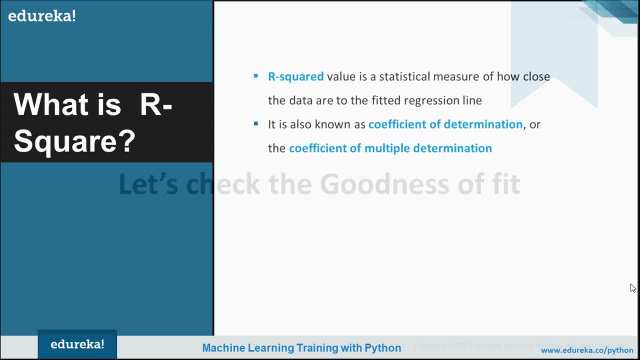 data right. so let's say I teach them on the 70 data points and then 30 data points I kept as a secret with me so that I can test how much it has learned onto those 30 data points, right, and that is where R squared is. so for those 30, 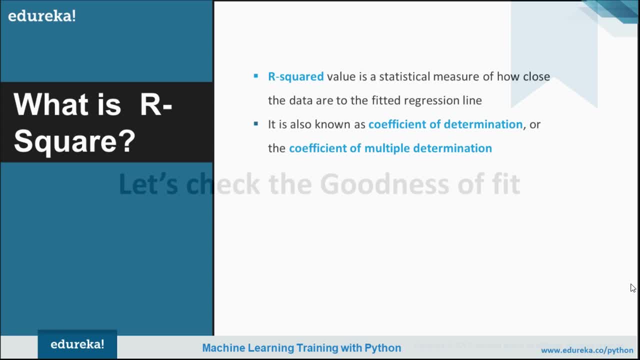 data points. you may use whatever way. you want to test them, or you want to look how exactly how good it was. you can use the R square value, or you can use the, or you can use the mean square right. so there is a whole theory about that. we. 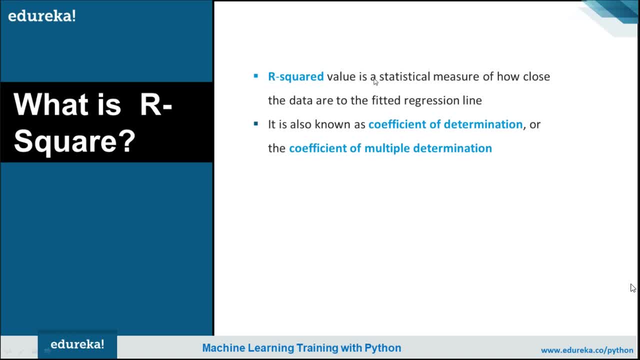 will keep it very simple and short here. so R squared value is a statistical measure of how close the data are to the fitted regression line. so using R square, you talk or you say how much close our data is to the fitted lines. right, so the line which we have chosen, how much close it is to that line, and we call it as a 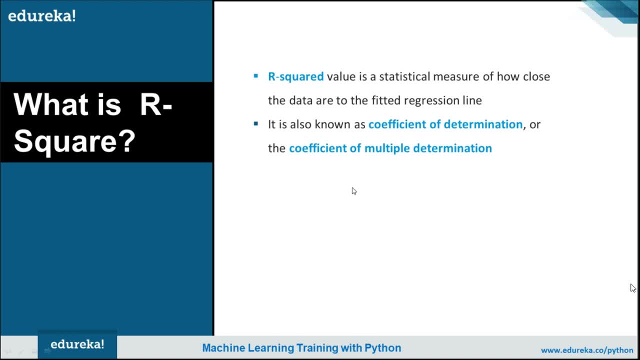 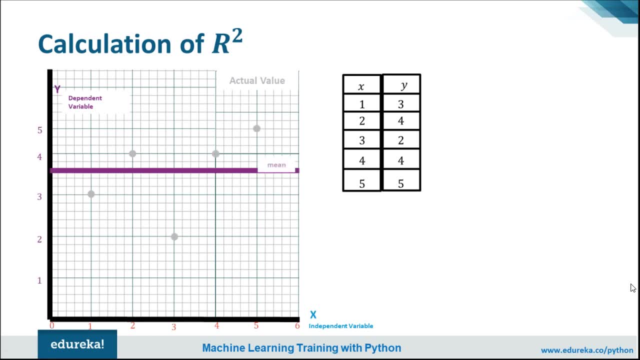 coefficient of determination or the coefficient of multiple determination, right? so let's see what does it mean? R square R, how do we calculate it actually? so, first of all, we normally so we calculate the distances, that is, actual minus mean, right? so we take all of these data points. so these are the. 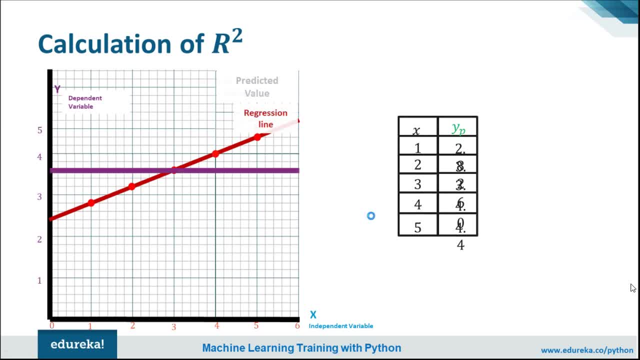 predicted value Y, P, right, and then we have the actual values also for that. so how do we calculate it? so this is actually that if you take the distance actual distance right and you subtract its value from the mean, and you are drawing it with the distance predicted minus mean right. so what you 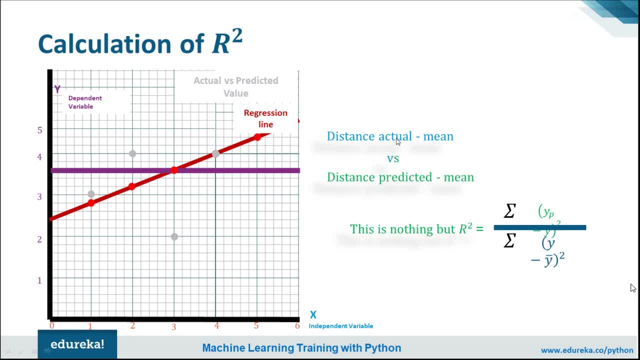 are doing here. you have the actual distance and so you are looking for actual distance from the mean value, right. so whatever value, you caught exactly that. okay, this is my data point: how much far away it is from the mean right. so you do this thing and you compare it with if you do the same thing. 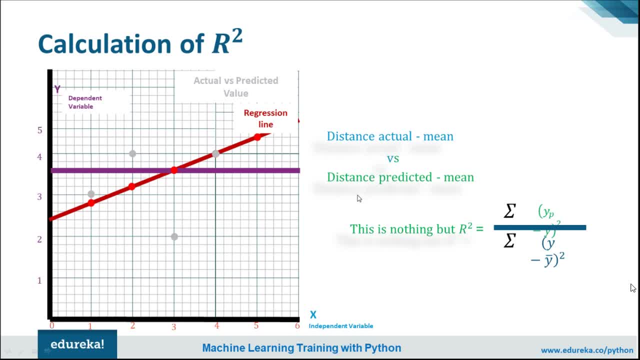 with that predicted value, what you are predicted, how much it is away from the mean value, right? so the one which is predicted value and the one which is your real value. so your R square formula is: what summation of Y P minus Y square? actually, this is numerator. 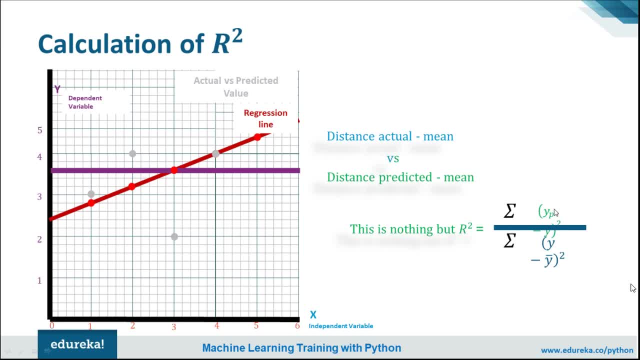 green color is your numerator completely, that is your Y P minus Y square right, and your denominator is Y minus Y square square. so what is this Y bar? so Y bar is same in both the cases, because this is a mean. but what is this y piece, the predicted? so, for each of the values, 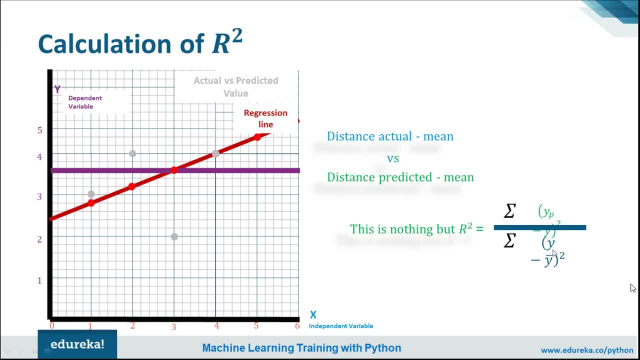 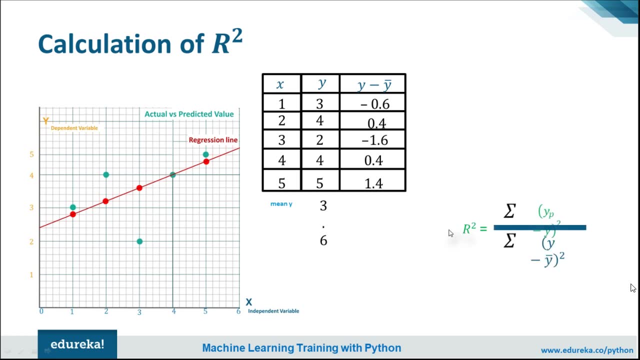 we what is the predicted value, and then you will hear, by defining that real value- so you are comparing both of them- how much far away it is from the distance, right? so let's talk about R square here. so we have this formula. so for this you will calculate. so 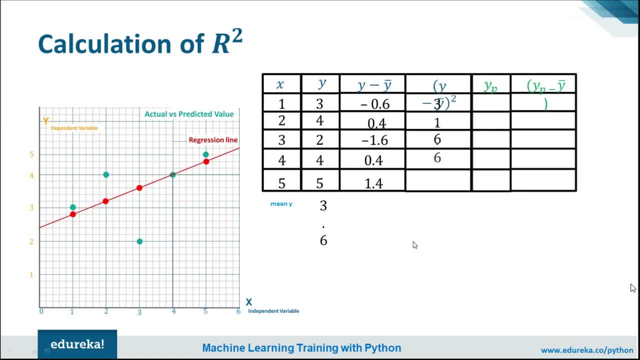 for Y, right, so we know the mean for Y, so we to be. so. this is actually a little bit overlapping, is there? but we have the Y value, real Y value is there. we have predicted by values also here, right, which I show you by using the equation: Y is equal to MX plus C, our MX plus C. and here you can. 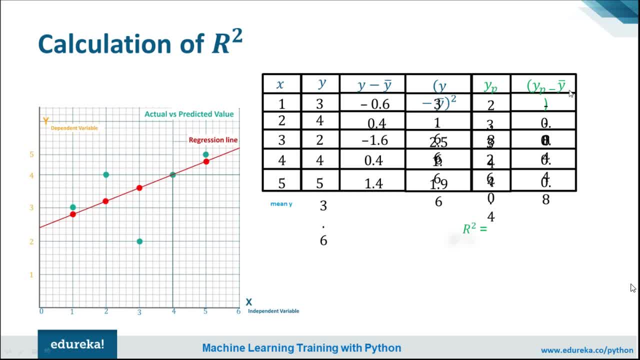 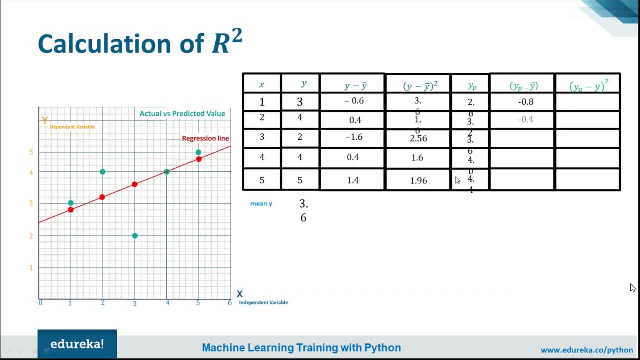 see, this is our Y minus Y bar whole square and this is YP minus Y bar whole square. right? so this way we do this formulation and when we do the summation calculation further, then we find in this case this is coming 5.2, this is coming as 1.6. yeah, Bharat is saying table data is overlapping. 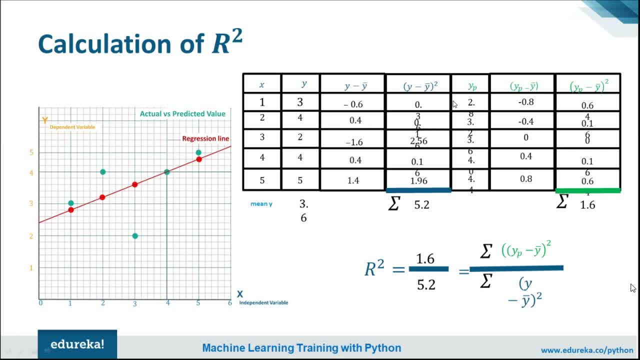 yeah, data is little bit overlapping actually, so this PPT has been made actually special. table: data is overlapping actually, so this PPT has been made actually special for you guys. only so because we were thinking to you know, do it for you basically, in which they were unable to test it actually. so because of its little petitions are there, but it will not happen. 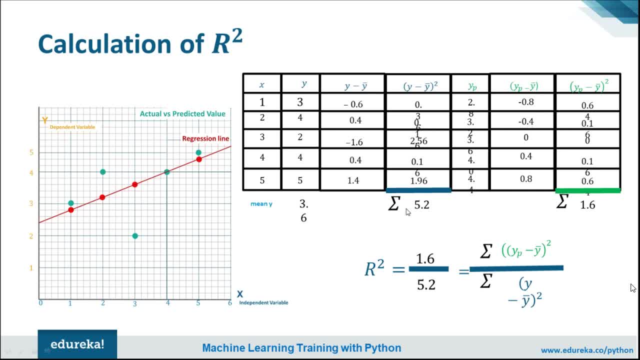 from tomorrow onwards. okay, so this is the final values which you will get here, right? so summation: five point two and this is one point six. so you divide one point six by five point two and then you've got your R square value. so what is the R square value in this case? you are getting 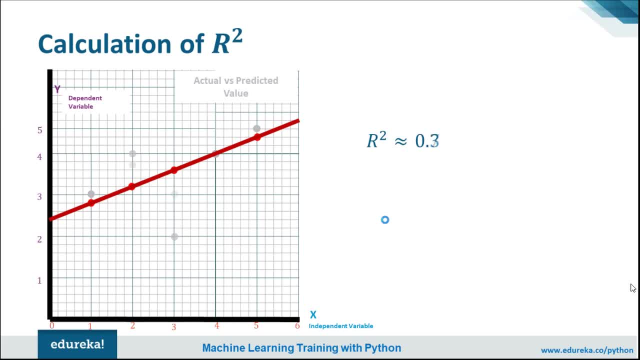 is fine, three, right. so now, what would be the good R square value, right, so for a particular case here? in this case, is R square its fine three. in some cases it might be R square. so if we take the different data point, right. so if these are the data points here, right. so here, here, here, which? 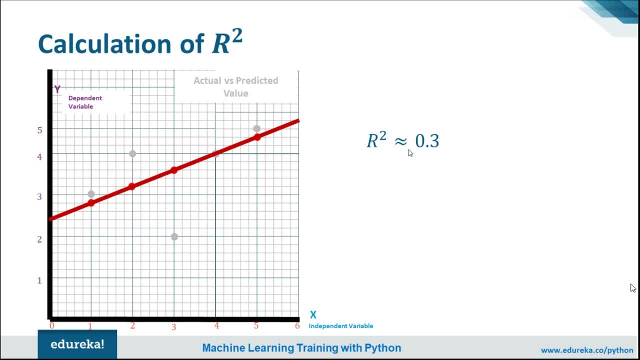 is far away from your this line, right? so what value you are getting? R square is equal to 0.3. but as you start bringing them closer to the line, then what do you will find that R is equal to 0.3, that R square value increases, which is 0.7, right, and as it becomes more than R square. 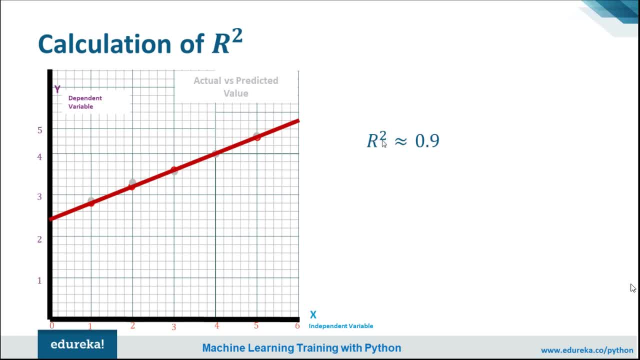 value would become 0.9.. Jaggi is asking how we get yp values. yp values, you remember? yp is nothing. but once you calculated this formula, right? that is, y is equal to mx plus c, right? so when you know the m value, when you know the c value and you have already x value, then 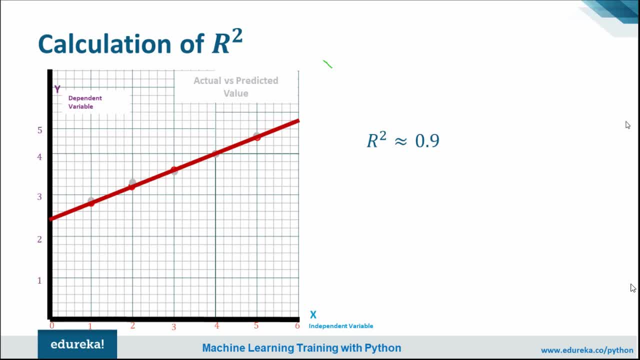 yp value you can calculate by writing mx plus c, right, while the real y values already given into the table, while yp is the one which you have predicted. is it okay, Jaggi? okay, great, so you can see, as the data point is coming more closer to the line than it is R square. 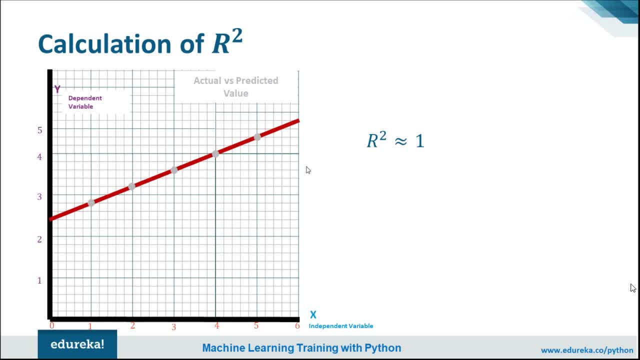 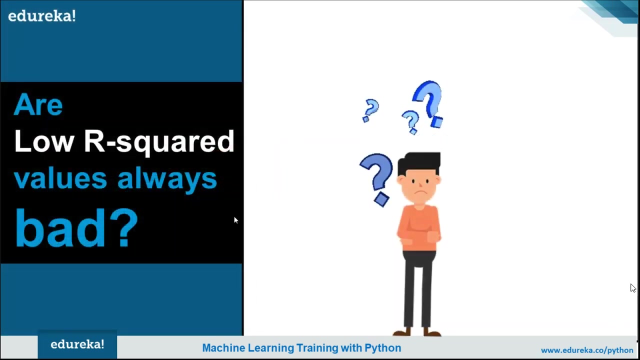 values increasing right. So when it is exactly on the line, your R square value would be one, right? so if we see here R square, if we see the data's are far away from the correct value, so, like here here, here, in this case, R square value would be so much less, which is 0.02. so there are question are. 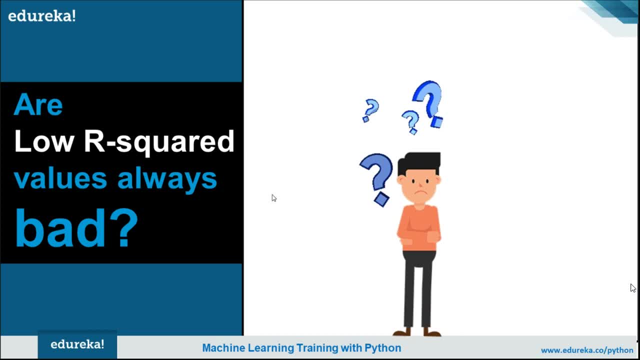 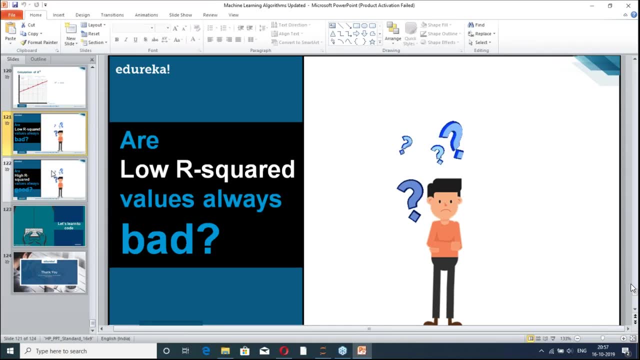 low R square values always bad, or like mostly we will say: yes, it is, but that's not always the case. we we can't talk currently here mathematics and the cases here, but currently you can keep it in your mind that the high value means good, low value bad, but not always right. we. 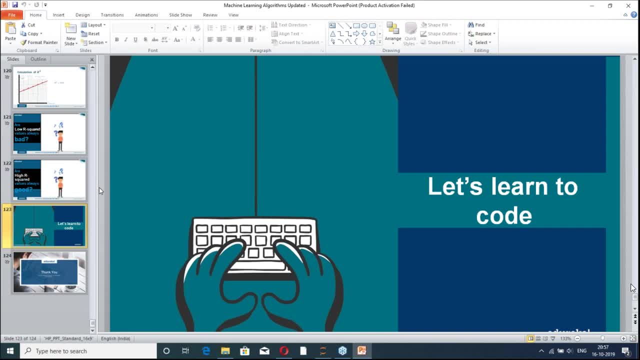 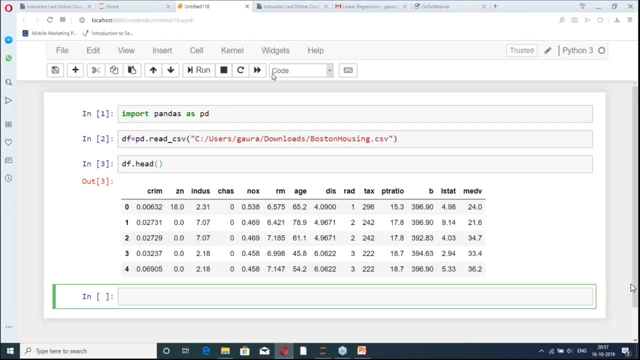 will be discussing it when you will be going through the course. now we don't have much time actually, so we have to do some coding as well, right? so we'll be doing some coding here. so this is the data set which I have taken, right? so this is a we are going to do. 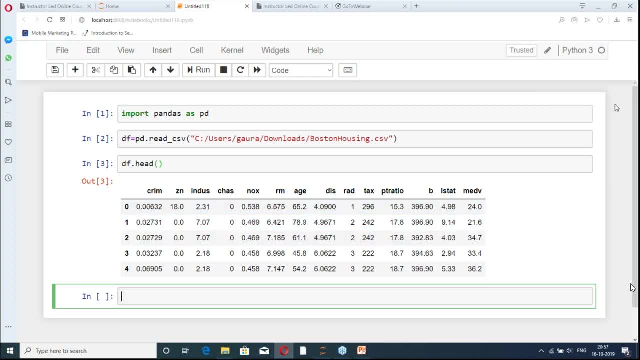 the coding for this data set, so what this data set is actually. this is a Boston housing data set, and so first of all, let me should tell you what I have done. few lines of code I have written here already, like I am importing Pandas PD, so basically I am importing this. 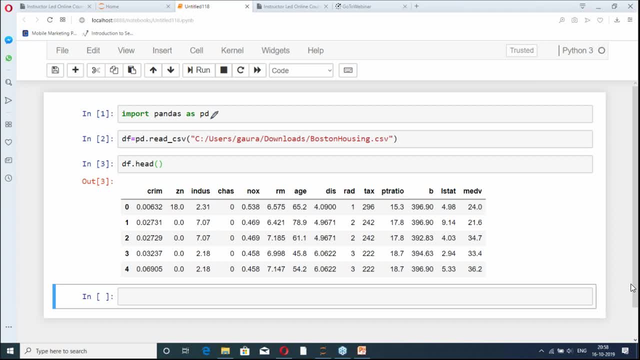 library, Pandas library, which is used to create the data set into a tabular form. particular form is there, which is we call as such in Python as data frame right, so it's pretty easy. I can import this library and because this is my data set in the CSV file, which is Boston. 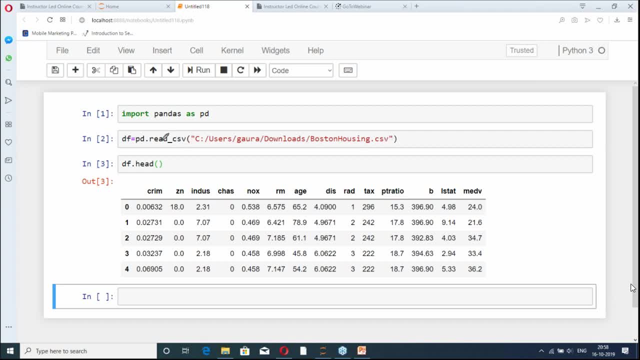 housing dot CSV. I can read it by using the read underscore CSV function, right, so here I'm reading it, and then I'm just printing those top five rows: 0, 2, 0, 1, 2, 3, 4 rows here, right? so top 5 rows. if I want to print, I will use head function df dot, head right, or if. 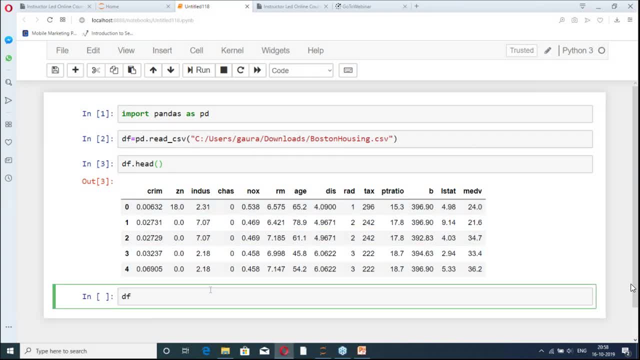 I want to. so if I write df, it will be telling me that I want to print df dot head, right. so if I write df, it will be telling me that I want to print df dot head, right. so if I write df, it will be telling me: show more about these. so lots of values are there, right. 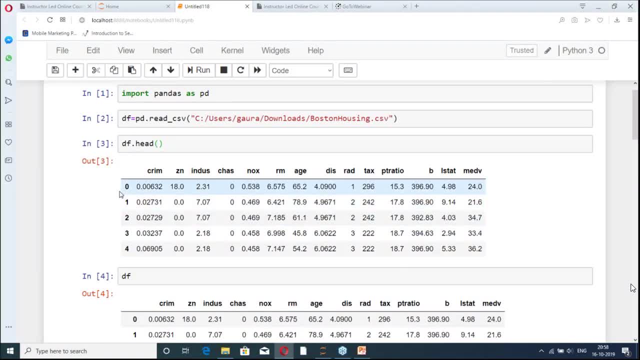 so let us huge data set. we want to see just minimum top five rows. we can see this thing. so what it is showing actually here? this is my first row, right? so this is what data set it is actually. it is a Boston housing, let us say some real estate company. come to you. 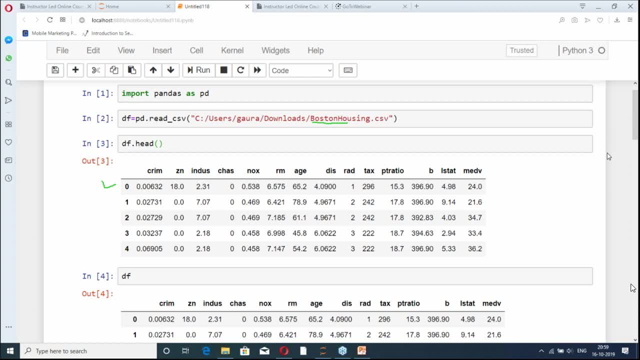 and they want you to make such a model so that they can predict what would be the prices of house, right, if, if, if values are given to you right, or if some properties are given to you of the house, then you should, your model should tell what is the good price for this house, right, or what should be the expected. 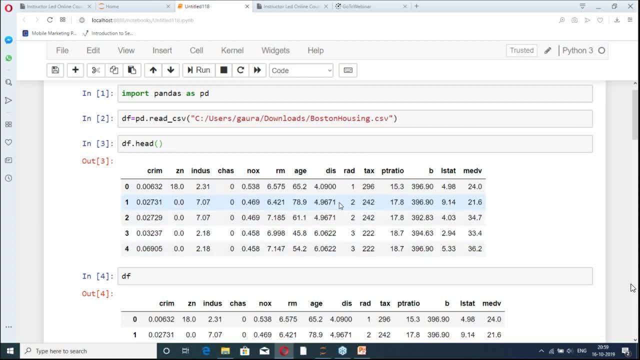 price for this house. so they have collected the past data and in the past data they route like this: this is the first row of data which they collected- zero through means first row here- and they were showing that crime rate. crim is a crime rate, which is they were showing crime rate. 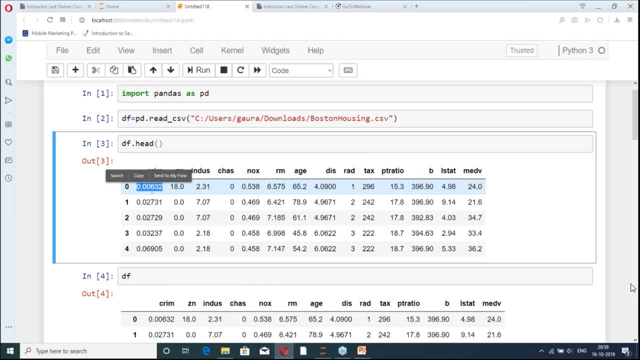 in which society this houses is around: point zero, zero, six, three, two. then they are. this is another one. let's say this is zone. so let's say how much green zone is there around? let's say 18. so these are different, different values. are there how old the society is, or how this 65.2 years? let's say: 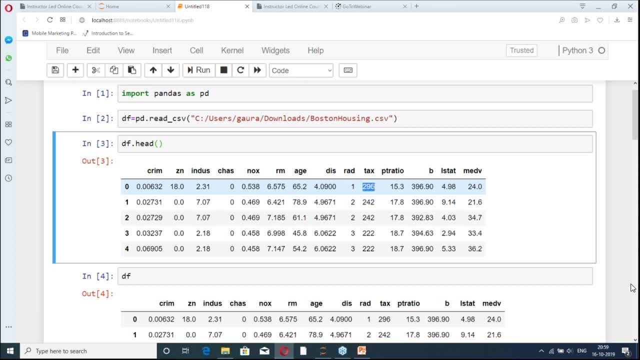 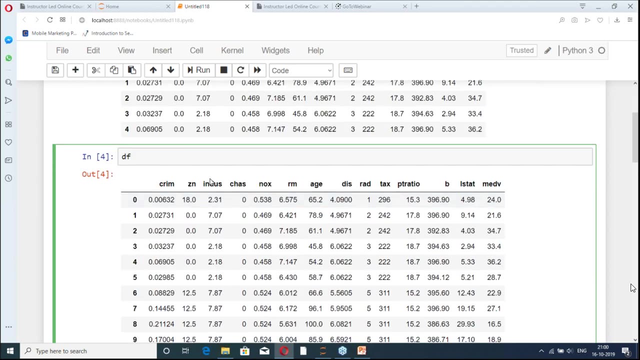 right and so on. so what is the normal tax being paid into this society? house tax and all is this much and this is the median value of the house, into this particular society, and all right. so this way we have lots of data set. so we want to do all here is to make a model so that whenever anybody give us 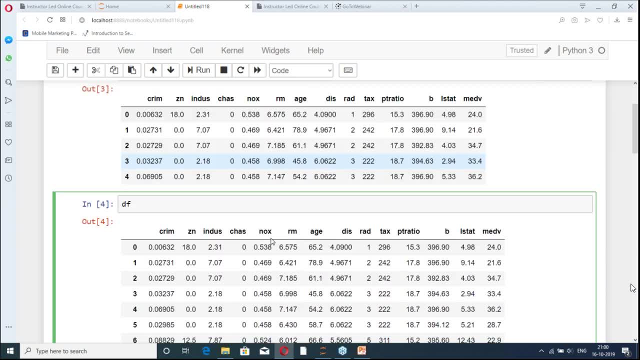 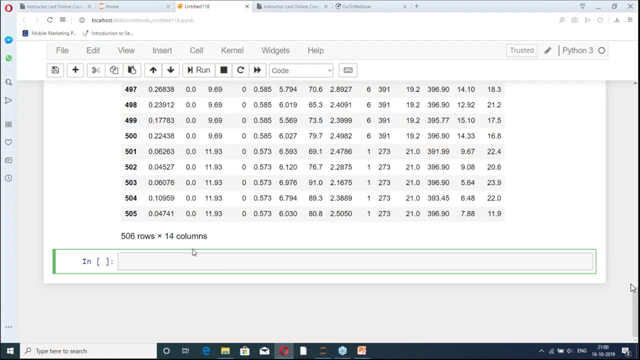 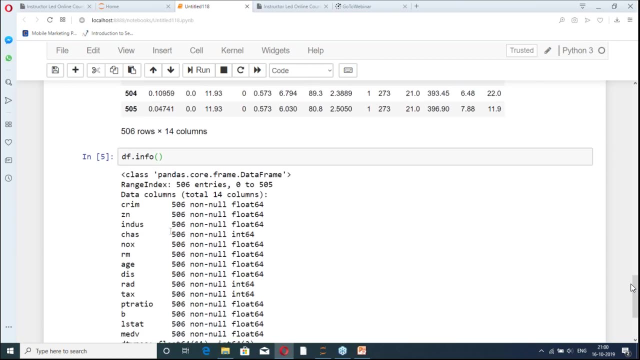 these different value, we can predict what is going to be the correct value, right? so for this, let's say: if we, if you want to see this, so here we have the 14 columns, right? so if you want to see in what exactly these columns, so how many rows of data they have given us? 506 rows of data they have given us. 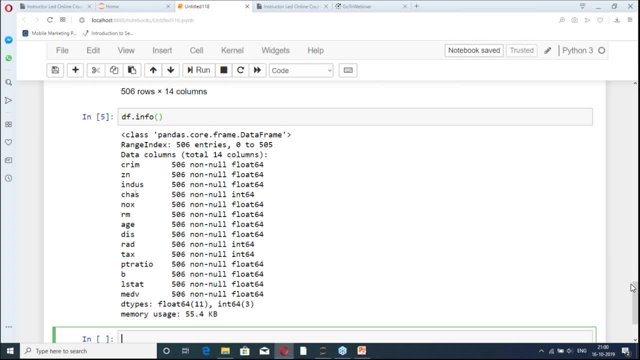 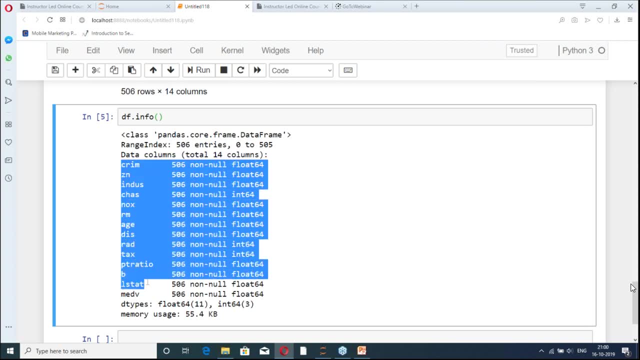 where these are different, different values, crime values, zone, it does, and all and this is our output variable, actually right. so this is initial variables. these are our input variable, we can say, or independent variable, we can say, right, and the median value is our dependent variable, or we can: 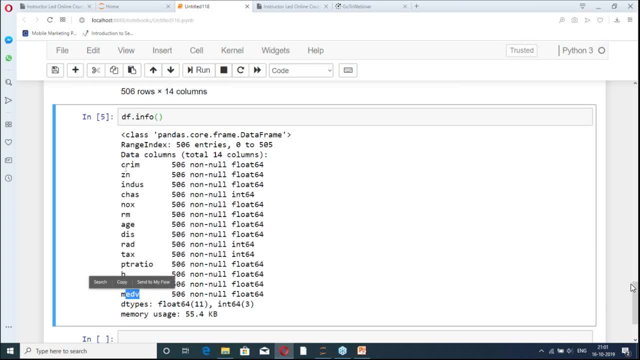 say y, right? so like you can think, all these things are my x values right and this is my y value, right, because this is what i want to predict it. okay, so now we are going to apply our technique. that would be machine learning. so for that we need: 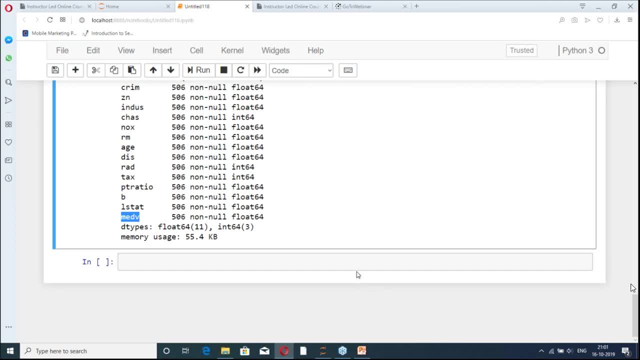 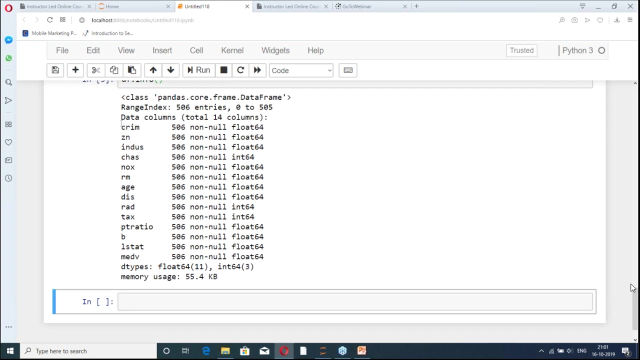 to import few libraries, right? so, first of all, what we are going to do, we will divide our data set into the two parts, right? so what is those two part would be exactly? so these two part would be our. we will take one: our training and testing. so you can think that let's say this is the 506, uh, how this data has been given. 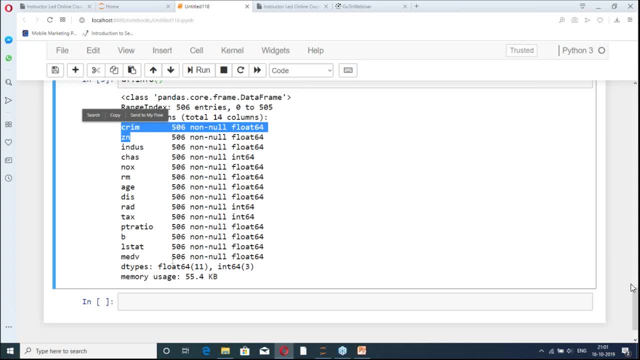 to us, right? so what is the output value for them has been given. so what we will do? on 70 percent of this data, we will train our this linear regression algorithm and on the 30 rest of the algorithm data, we will test them. that what result it can give? right, so, according to this exactly is asking: 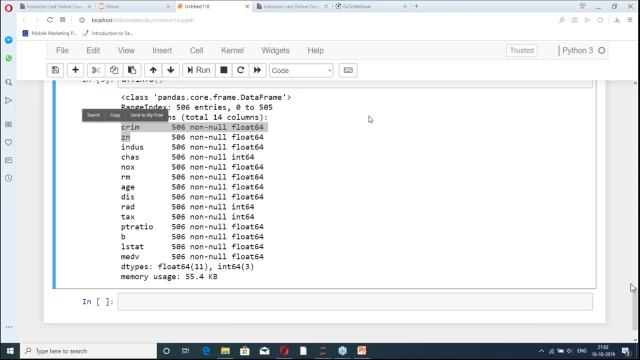 according to this example, it will become an independent variable, correct? here we have n independent variables, right, or actually 30 independent variables. we can say we have total 14 variables, in which this is our output variable or dependent variable, and the rest 13 variables are our independent variable or input variable, right? so, first of all, 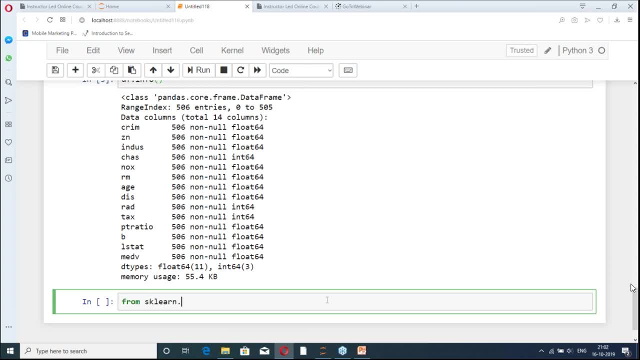 we will take from sk learn dot. so there are. so, first of all, what we are going to do. we are going to divide our data set into training and testing side. so training is on which my machine learning algorithm will try to- uh, we'll try to learn, right. 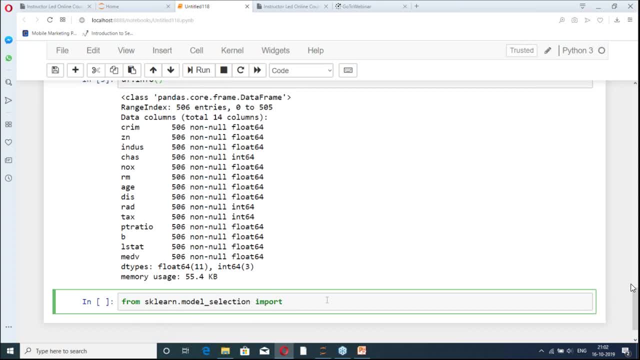 we'll try to learn right. it is equivalent because this is supervised learning. it is equivalent that 70 questions we are showing with their solution and for the rest, 30 questions we will do the testing that how it can generate the result right. this is uh. this is a library which is within. 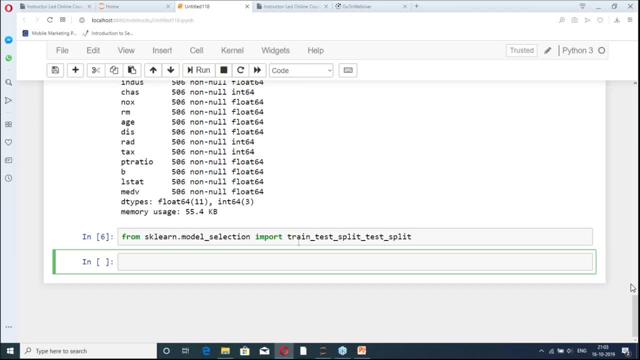 sklearn, we have this module, model selection, in which we have this function, train test split, right. so we imported this thing and it will divide our data set into two parts. so before applying this thing, what i am going to do, i am going to tell what is my y value in this. 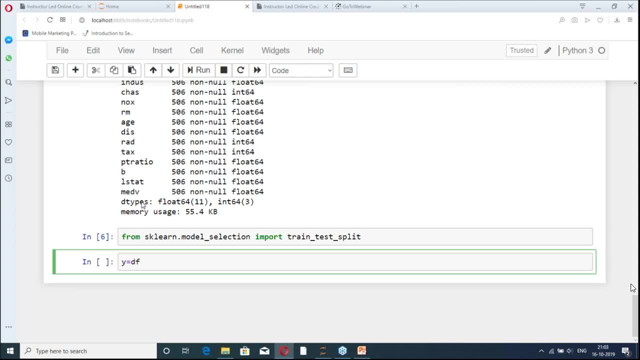 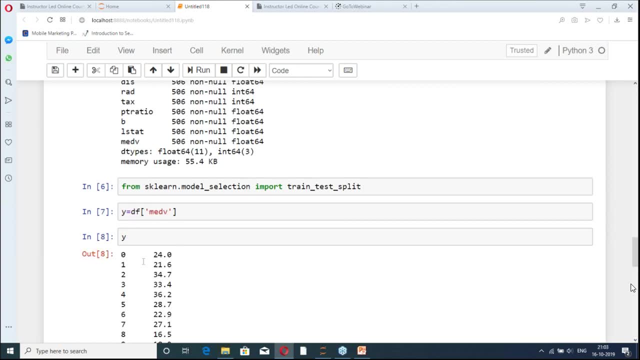 so y value is my median value. so i will write: y is nothing. but in my data frame if i take median value is my y right. so basically i have taken y here separately, right? similarly i will take x, the rest thing i will take here. so i will write df, dot, uh, drop. 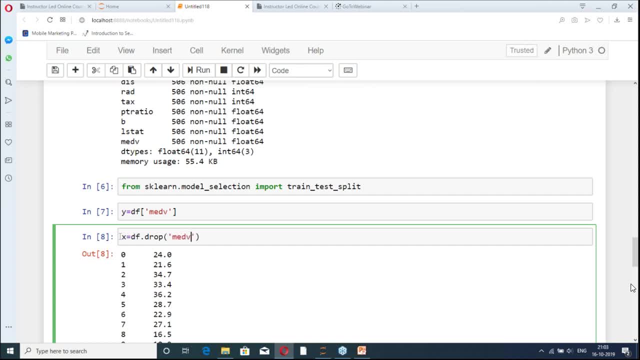 and here i tell which column i want to remove. so i do not want to have the median value and because this is a column i want to remove, so i will write: x is equal to 1, right? so if i show you now what is x dot head, so the top five rows we can see here you can see. 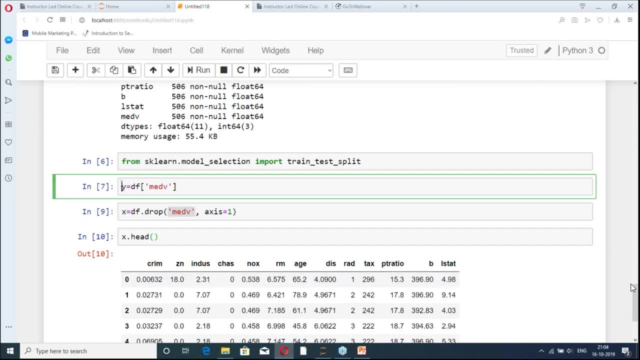 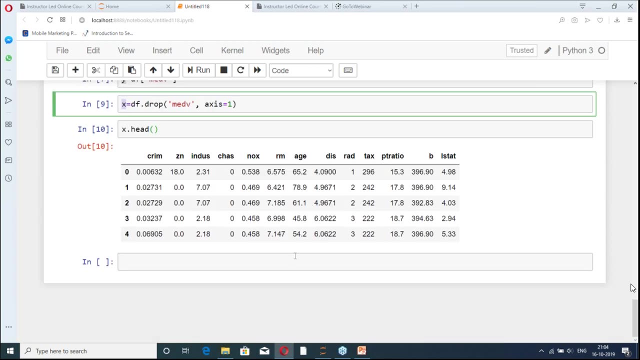 median value is not coming because i have removed from here and i am storing here, right, so i am going to keep all my output variables, uh, dependent variables, uh, one dependent variable only. here we have into y and the independent variable i am keeping into the x, right, so now what we will do. 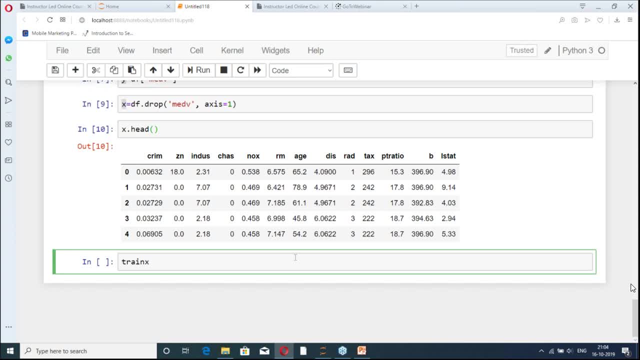 here. we will keep train x test x and train y test y, right? so there seems to be a question i will take in a moment. train test split function. i will call and i will tell what is my x, what is my y, and as well as i will tell what is the uh test size i am looking for, right? so let's. 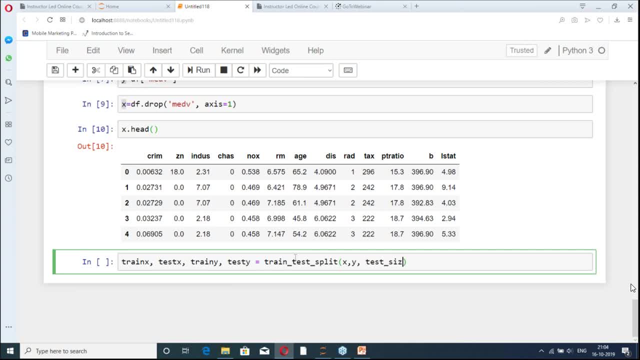 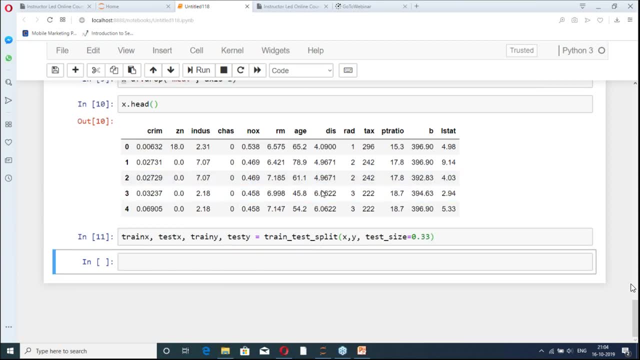 say, if i am saying 33 should be my test set, then i will say test size is equal to 0.33. so here we divide our data set. so jaggery is asking what is the use of faxes? so, as i told that, if i write x, 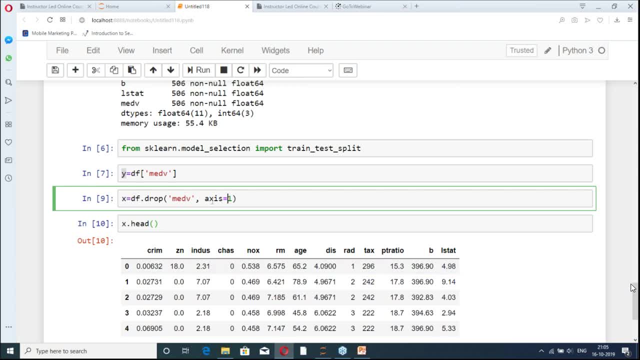 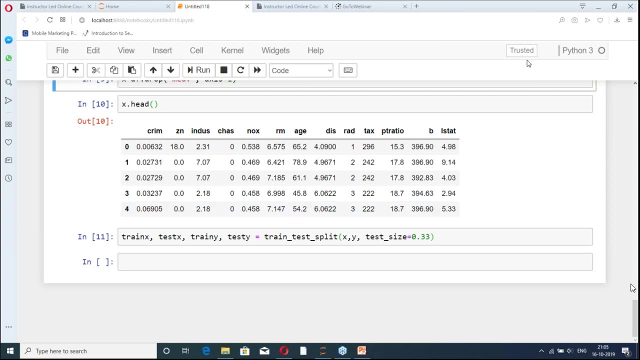 is equal to 1, it understand that i want to remove the column. if i do not write x is equal to 1, or i write x is equal to 0, it will think that i want to remove the row, right. so by writing the axis value, we are telling whether it's a column or row. okay, is it clear? i hope so now. 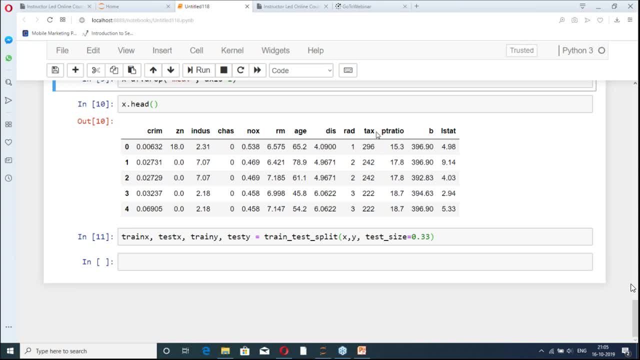 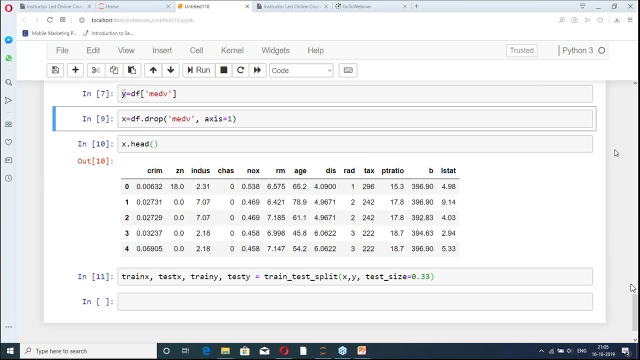 so bharat is saying: can you explain last line again, which line you are saying? line number 11 or 9? which one? bharat uh class. can you just write completely again? do you mean line number 9 or 11, line number 11.. okay, yeah, i'm coming to that. i didn't tell. 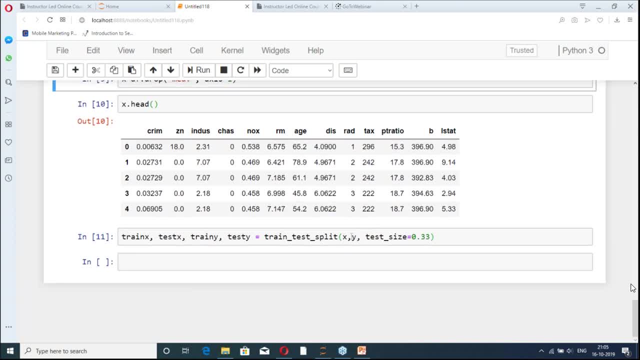 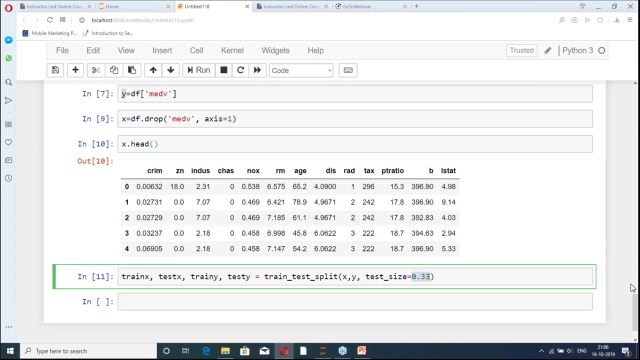 it completely actually till now. so x and y. i told you already what is my x right. so in x my all independent variable right and in y my dependent variable. all we can say output variable. writing here 0.33. i am saying i want to divide my data set into two parts. one is training, one is 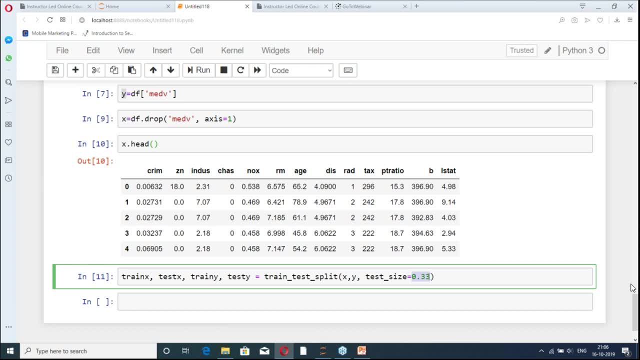 testing, the training on which i will give the solution, as it is equivalent that, uh, here i am telling. so here i have this book, in which this is a book of questions and this is the book of solution. so what i am doing using this particular function is: i am dividing by this book 100. 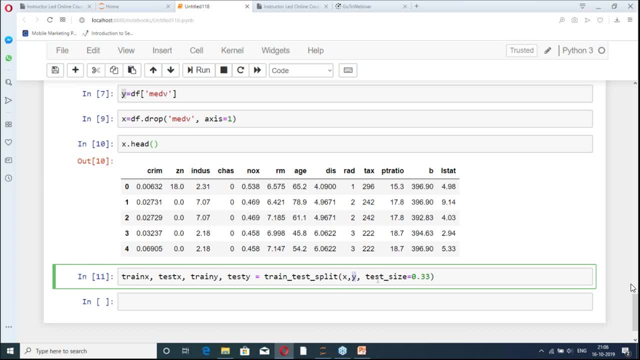 questions were there, let's say, earlier. i am dividing 77 questions i will take for teaching right, and when i teach those 77 questions i will show you the solution as well, while the 33 questions i will keep intact with me and i will not show you the solution to them, but for 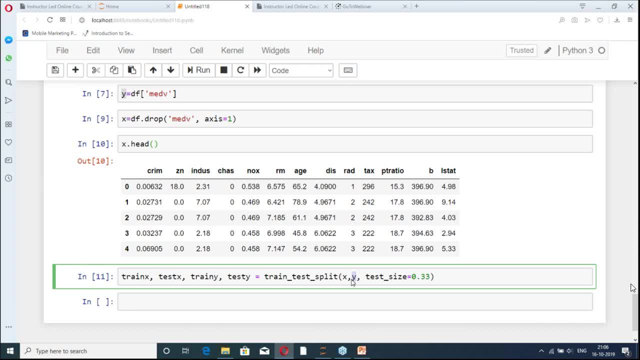 conducting your test. i will give you the questions, those 33 questions, and then i will match how good result you are giving right. that is what it is written. it is returning us for thing. this train x is my training questions. this train y is my training solution for these training questions. 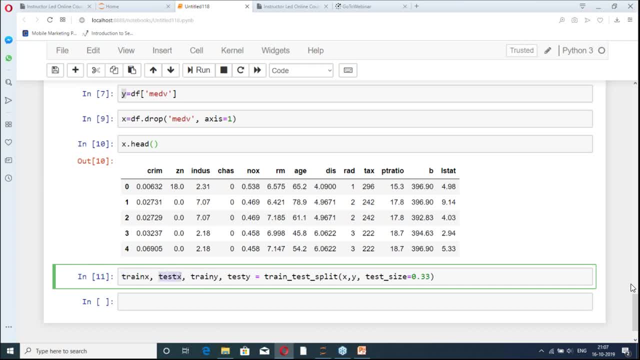 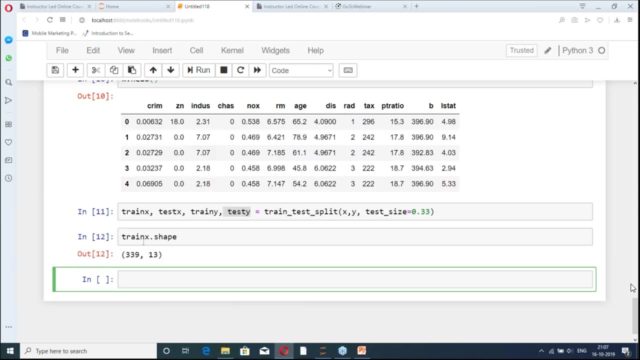 these are my solution and for these testing questions- these are test x is my testing question. for them, i have these as a solution. that is my test y. so if we see also, first of all, let me show you how many values are there. so in train x there are 339 rows or data points and 13, 13 column right. 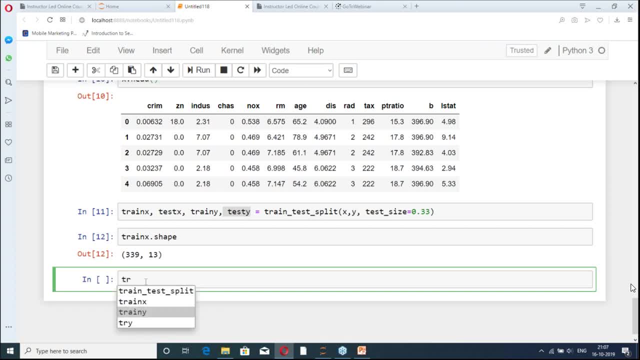 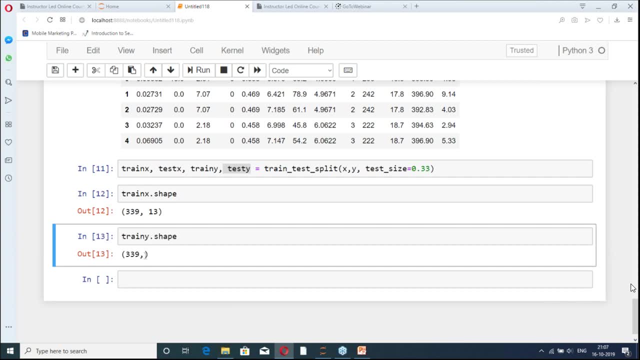 and if i show you about train y dot shape, then what do you see? only 3, 39 rows are there. so when it is nothing, it means one column. so it means this is exactly the result for all these questions. similarly, if i show you test x dot shape, then it is having 13 columns again. 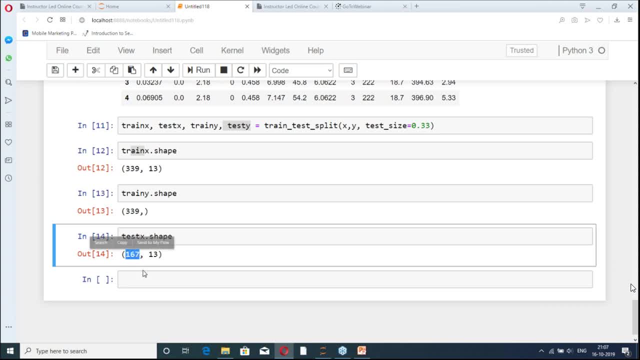 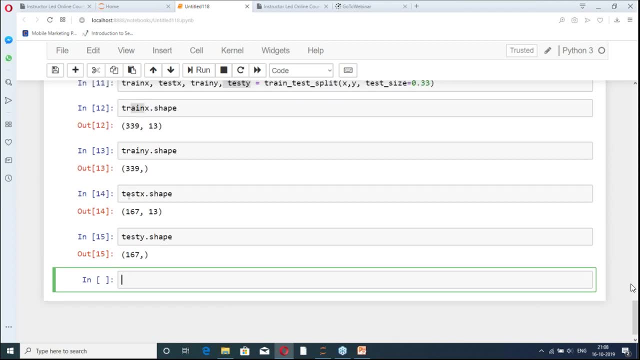 right, because all the input independent variable would be but 167 questions it has. We look test y dot shape, Then it is having solution correspondence to these Questions, right? I will show you also few of the top values, like if I write train X dot Head so that you guys can see top 5 rows. 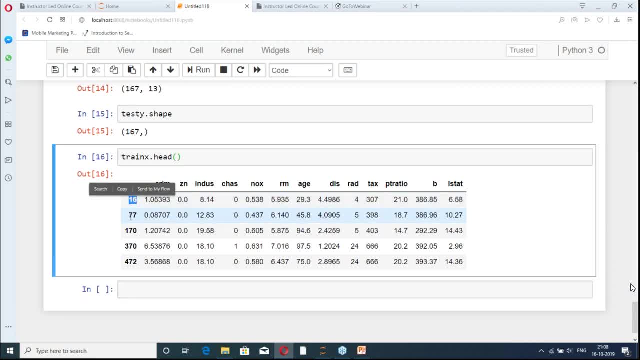 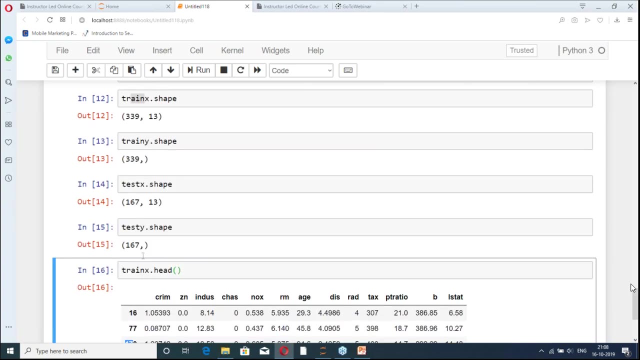 These are top 5 rows right and you can see randomly it has been chosen. first row becomes 16 row, then randomly chosen 77th row, 170 row. so randomly it has chosen 339 questions Right out of all will be as my five and next six questions, something like we had right. 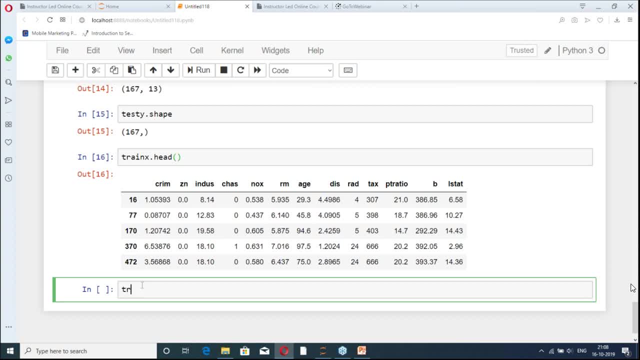 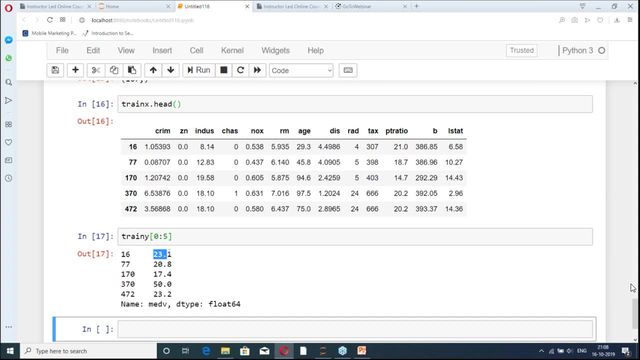 Similarly these are so corresponding to them. We have train why? Right, these are the top five solution. you see, this is twenty three, point four, five. So this is daily the sixteenth question, sixteenth here, seventy seven, seventy seven, so that you can match it with each other, and 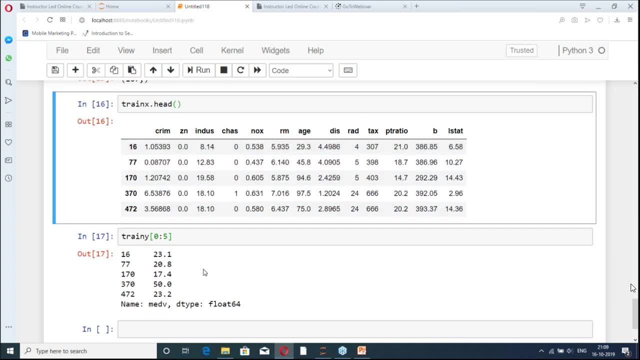 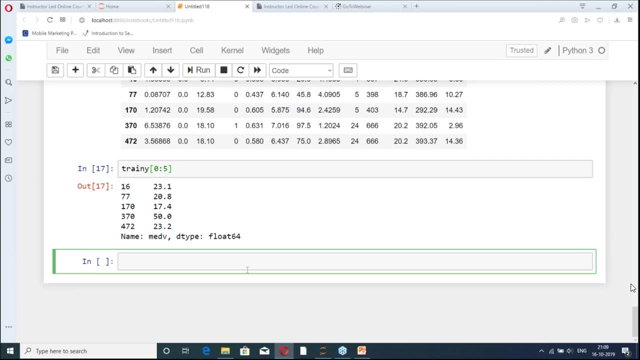 correspondence to this particular row of data or Variable. this is my output right. Similarly, we have in the test. So what we are going to do now, we are going to teach it Right using our Using our these training set. so for that we need to import the linear regression. 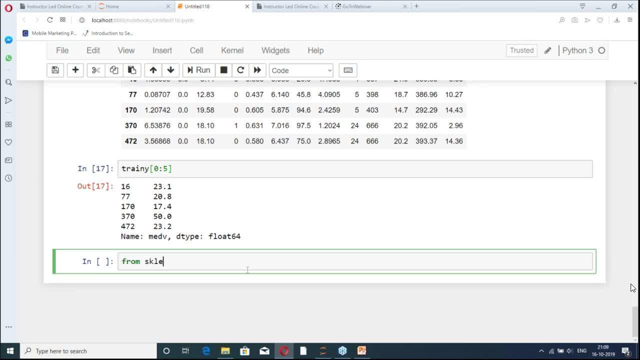 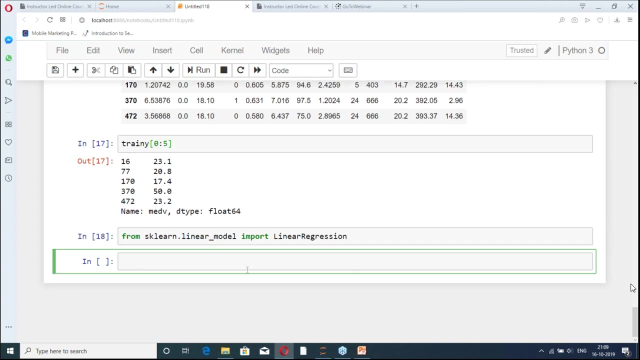 Model. so how we can import it. So we have again this library from SK lemon dot. into this We have a linear model family right. So this from this we are going to to import the linear regression right. So this is a particular class. 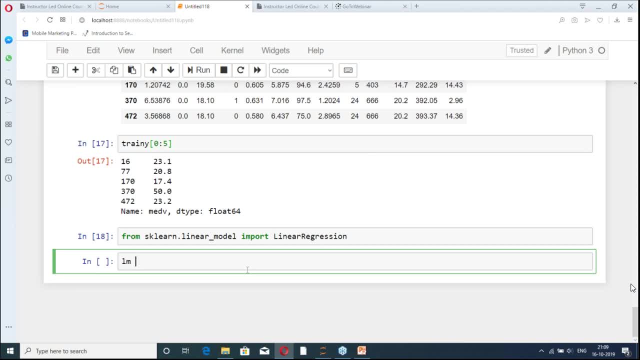 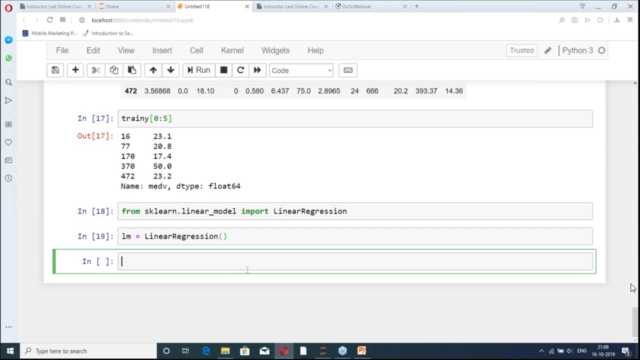 We have imported, now We can create its object. We create its object by just writing. LM is equal to linear regression. its object is ready, Now we can execute our model, So we write LM dot fit. So basically, fitting means I'm saying: learn right, how to learn. 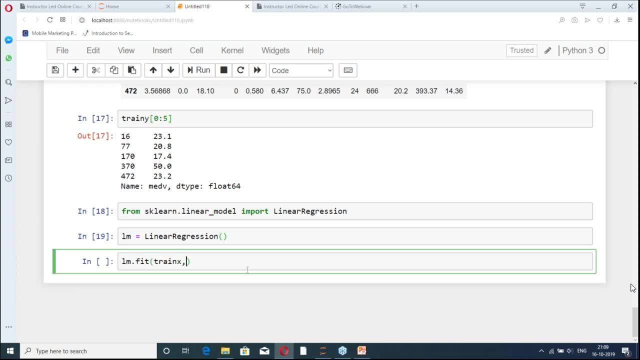 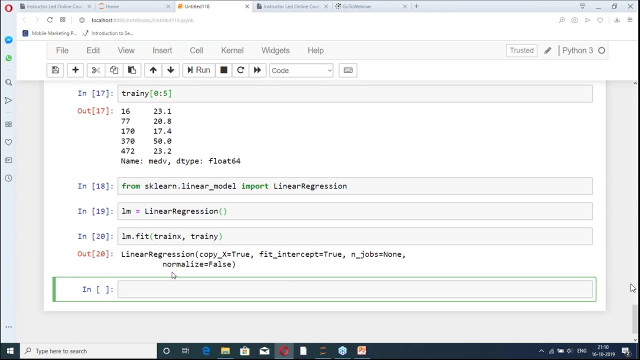 I will give it the questions that. these are the question. that is my train axe and these are my solution. So I am giving it questions as well as the corresponding solution, so that it can learn from it or can find out the solution. So it has learned it now right? 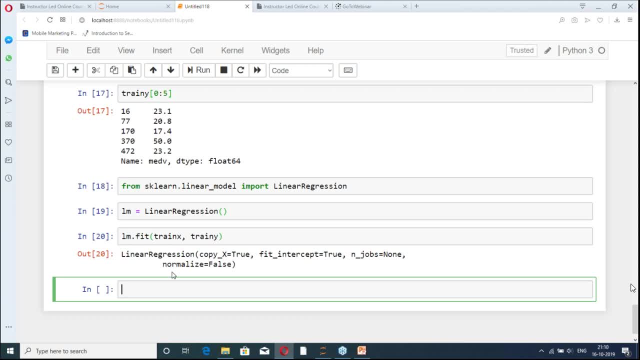 And now we can test it. So how we will test it? basically we will do the prediction right. So we? how do we predict the values? So I want to predict now what output it is giving. so I will use predict function in this. 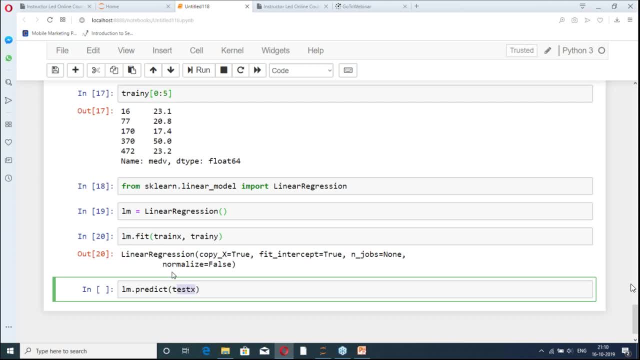 I will pass only test x. now you can see, I'm just passing the test x, right, so that I can see what it is predicting. and let's say, YP is my predicted output. So LM dot predict. we can say: here is the one which here we are predicting. 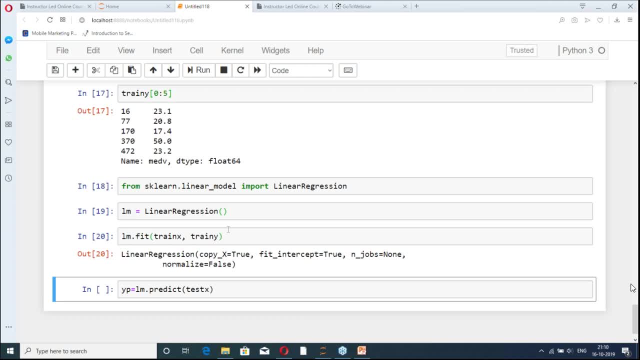 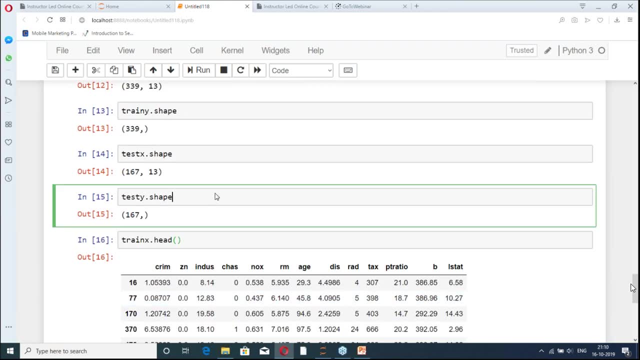 We. she is asking: Can you please explain the 16 and 17?? Yeah, I will go again to this line. right, 16 line. So we had our data set initially right in the DFB, had all the data points right. 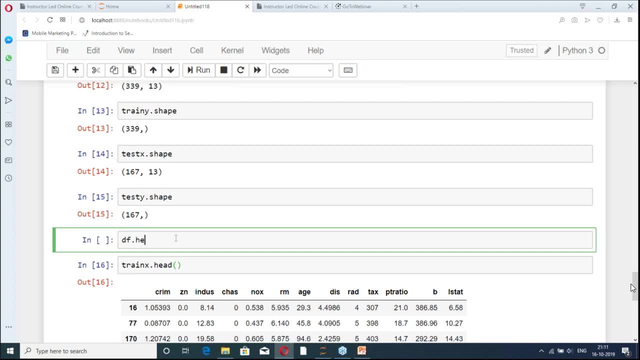 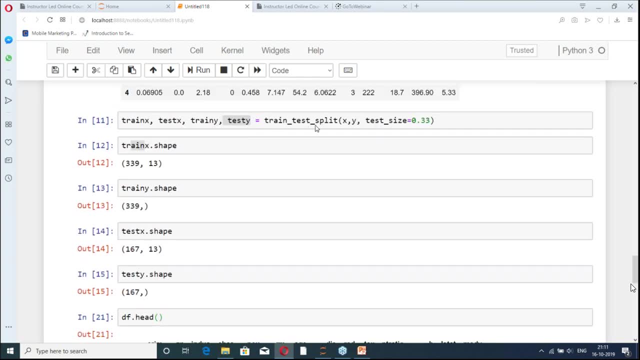 So if I showed you have taught in head, then it was having rose: 0, 1, 2, 3, 4, right. But when I call this particular function, train test displayed so randomly takes 339 value and put it into train X and whatever 339 value takes into train X, correspondence to them. 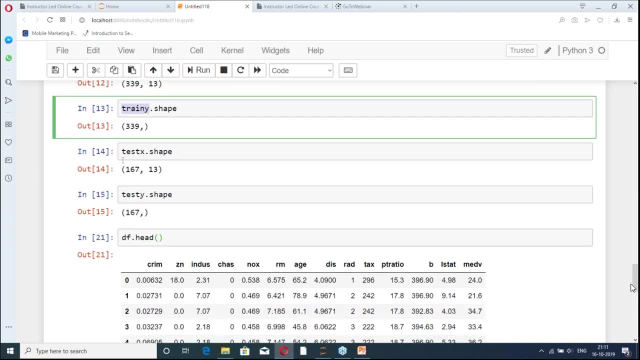 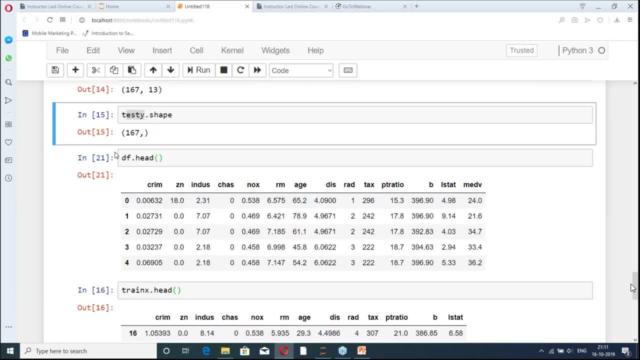 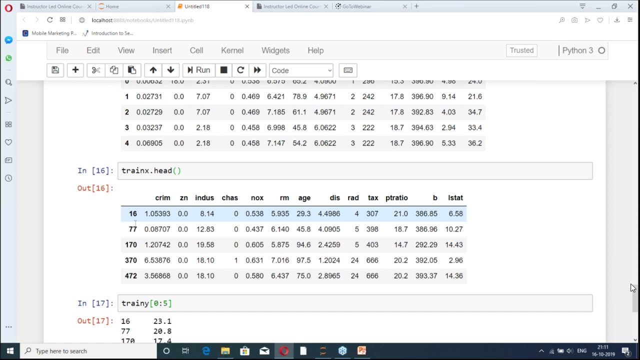 It takes 339 output values into train Y. Similarly, take test x randomly: 167 values and correspondence to them. output values were written here right. So this train x dot head is showing because it has chosen randomly. So first way to choose them randomly was 16. next to it choose. 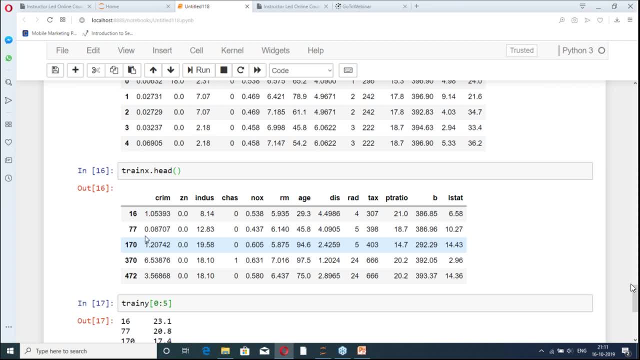 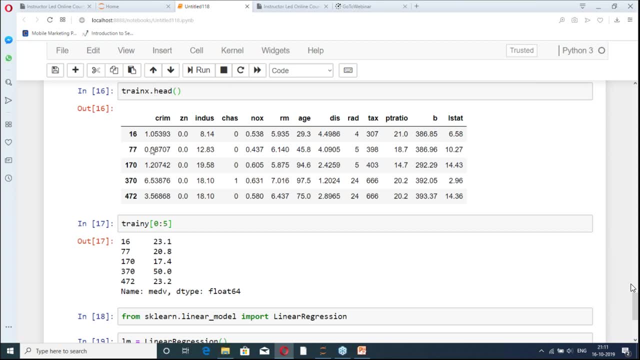 and randomly was 77. next to it, choose and walls up 170, right, So this is the way my data set is train X. That is my questions. You can say, if I am talking about question and solution train, why is my output values correspondence to them? 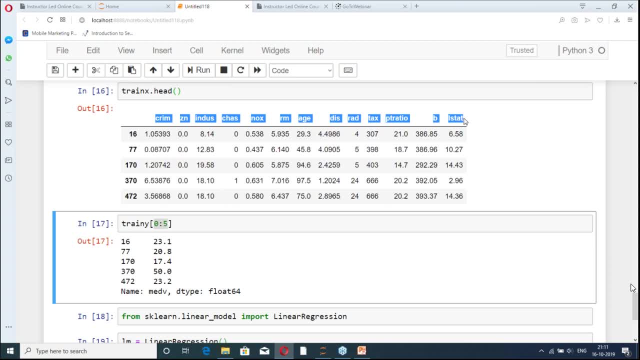 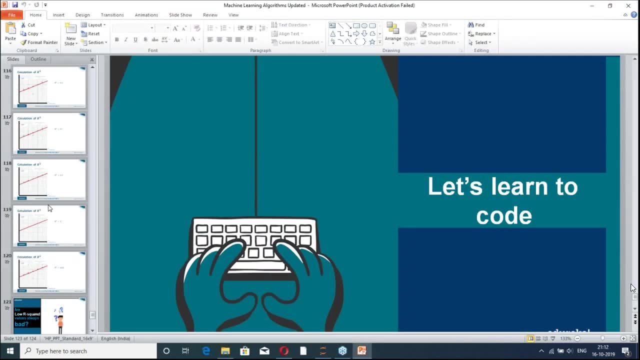 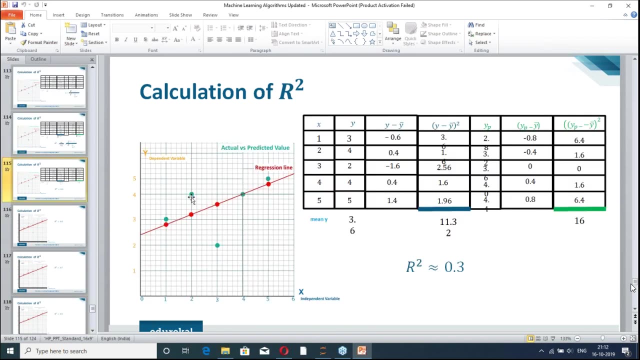 So within the train X, these are 339.. I have, or you can say, 339 data points or data observations are there, right? You remember from the slide we were having the observations right. So, like these are the observations right. 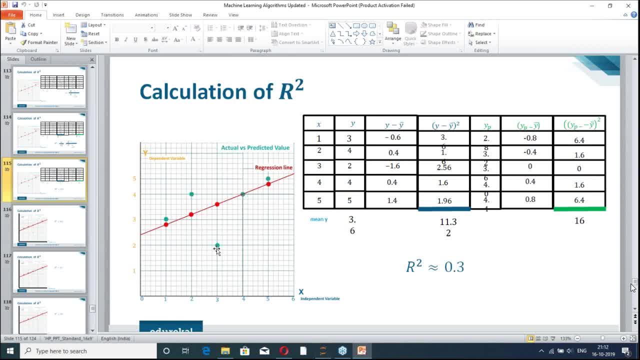 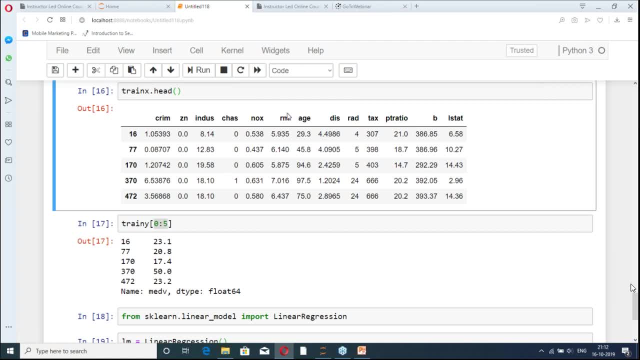 So these are the observations are there. This is nothing but so. X value is in my hair right. So these are defining my x value, because I have more than one dimension, one variable right, And Y value is coming into it, right. 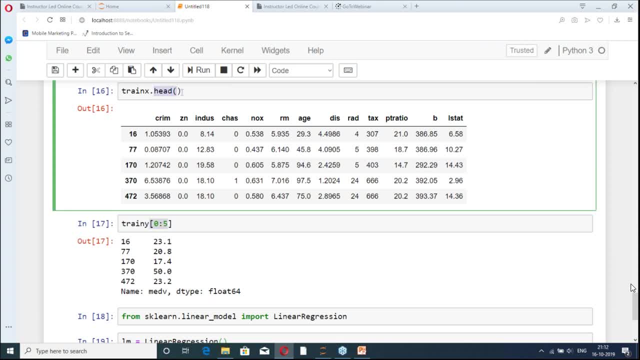 So I just showing you a top five rules. when I call with the data frame dot head function, It shows me top five rows only, right? Otherwise, if I do not write it, it will show me the whole thing. It will take a lot of space, right. 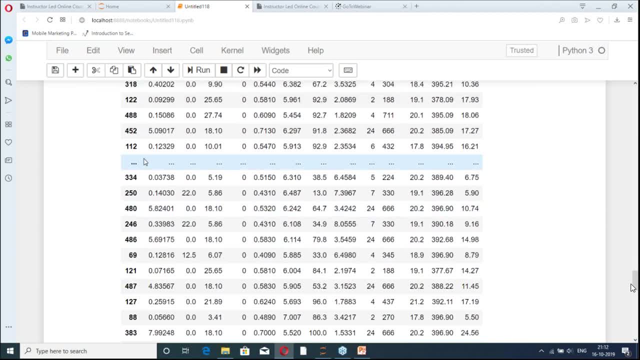 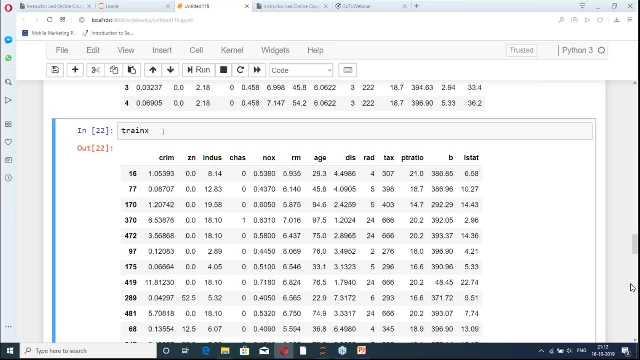 So if you see, here it is showing me all, nearly all the data points, right, Like here it right, dot dot dot. It means there are a lot of in between also there, right, But I do not want to take it to space on my screen. 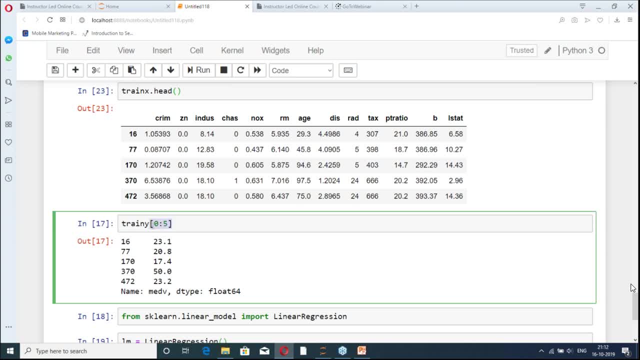 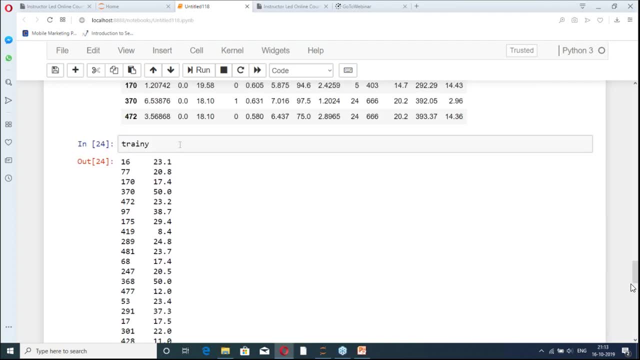 So I just show you the top five rows. Similarly, if I write train Y here, it will be showing me a lot of values like this, right, But I want to take on the top five, So I write here. So why I am doing here had and have I here 0 to 5. 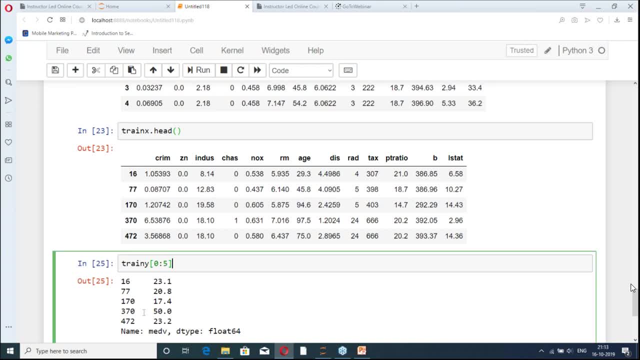 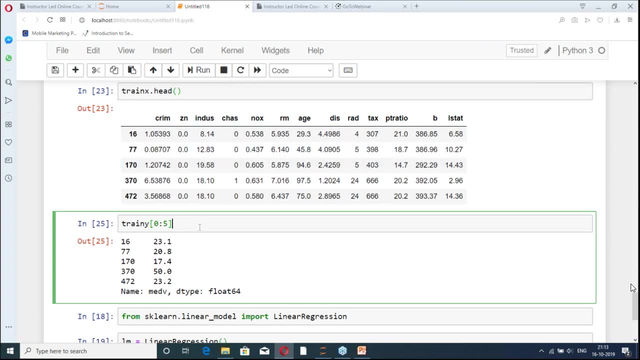 because this is a data frame, This is a series, right? So there is little different, that both things are handled in little different way, right? So whenever you have- so I will not go into that much, better be, keep it short- You can just say: this is a different data type. 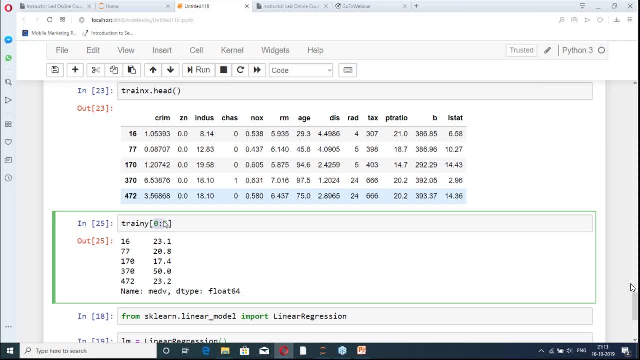 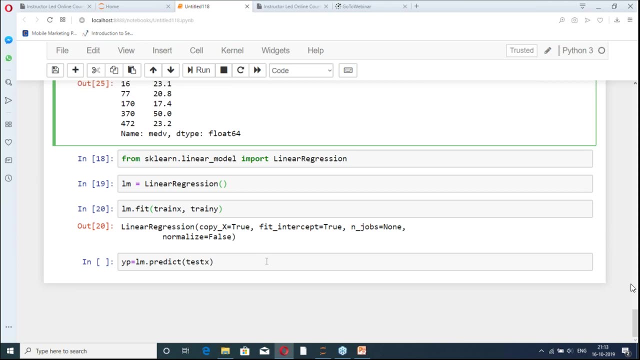 This is a different data type And in both, the data type for accessing them is little different way. Okay, Is it clear? Okay, great, So let's go ahead. Now I am going to preach the value: right. So this is modern. has learned it right. has learned now. 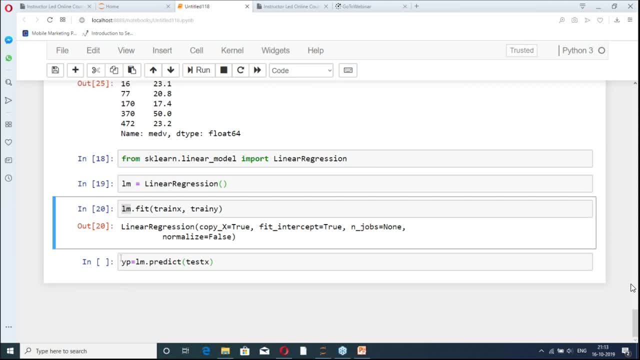 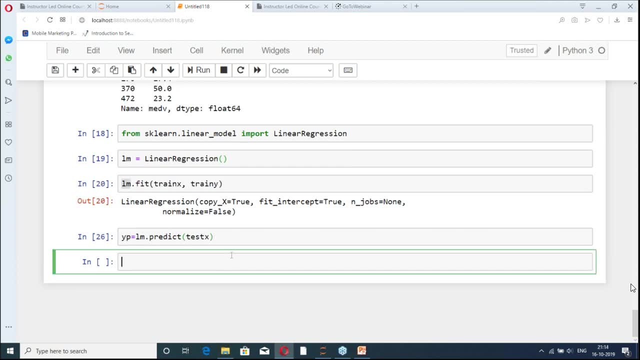 I am going to predict the values, So I will how I will predict the value I will write by. P is equal to L, Dot predict. So this is a function for predicting the value. So I, if I execute here, it has predicted the output value. 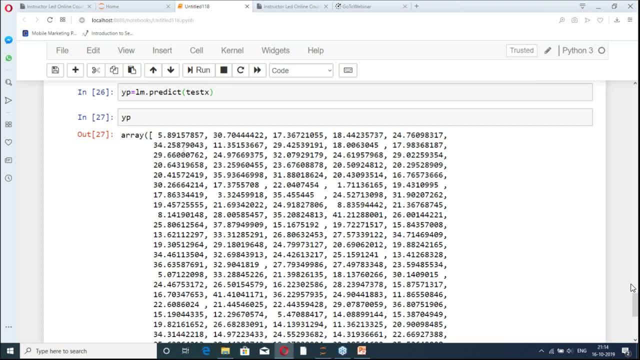 So what is the output? you predicted output values are these: 5.8 is the first one, 30.7.. Zero is the next one, right, And if I talk about the correct value is in my test tax, So it test, why right? 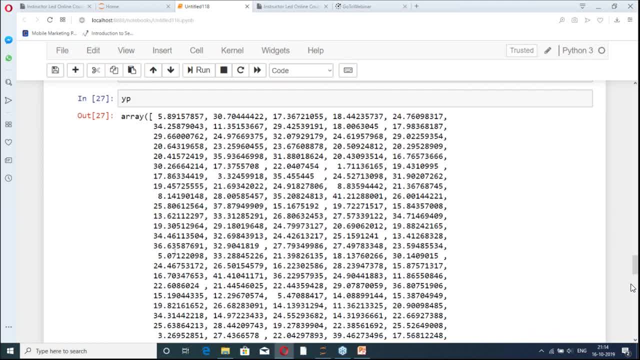 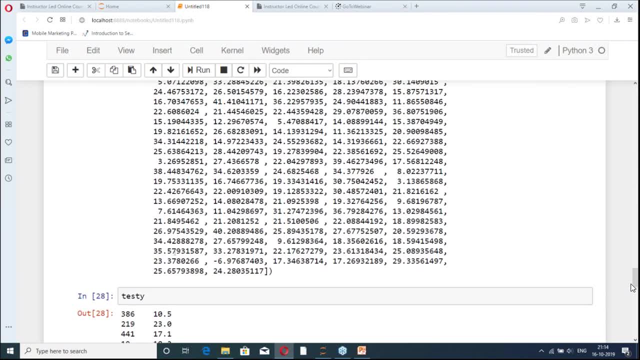 These are the correct value, that is 10.5, and on so on, right. So if you want to compare them as well, you can. we can compare it in different ways. We can compare it so we can show them together as well. 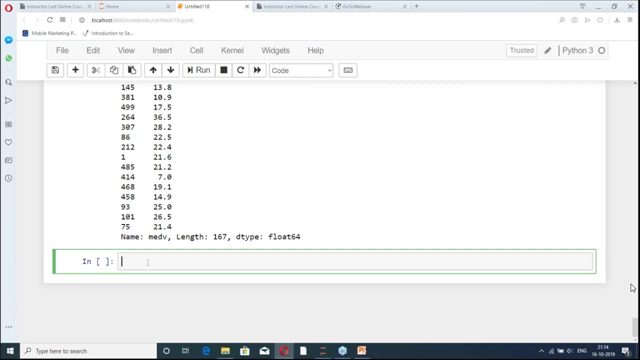 Let's say, let me make one data frame. Let's say I call it Opie data frame is equal to PD dot data frame, Right? So we make a dictionary. Let's say: real value, Real value is in our test, Why? and then we keep the another one. 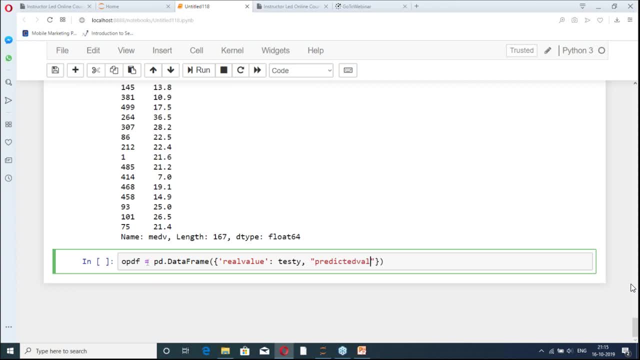 which is predicted value And that is into our Y right. So if I have executed or good data frame, if I show you so you can see, to the real value, 10.5, right It is showing also, row number was 386.. 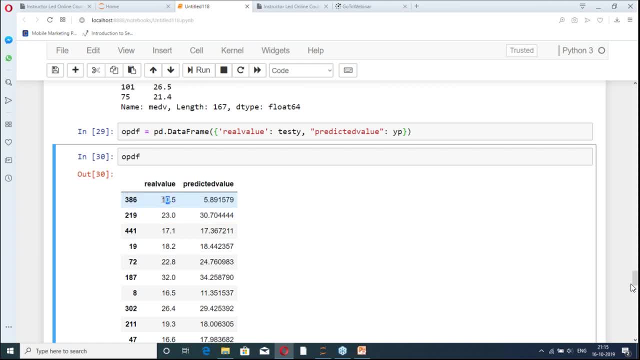 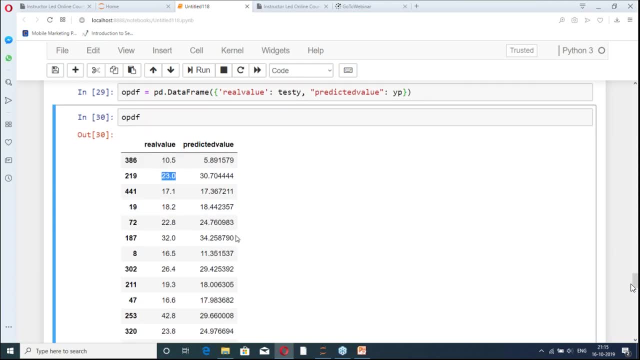 Let's leave it. look these two values. right, It's real value is 10.5.. But the one which we are predicting here is 5.8. here, The real value Real value is 23.0 and the one which you are predicting is 30.7 here. 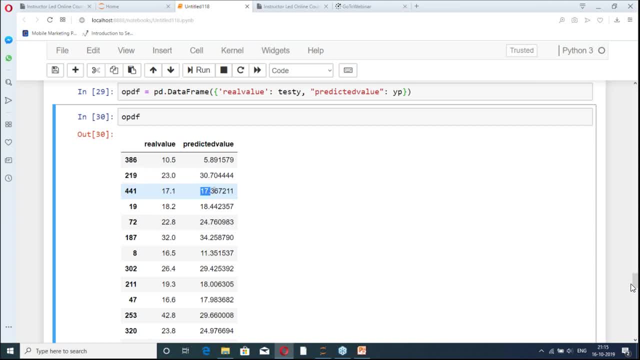 The real value is 70.1 and the predicted value is 7526.. So, very much closer, You guys can see 18.2. predicted one is 18.44, right, So this way, you guys can see 22.8, 24.. 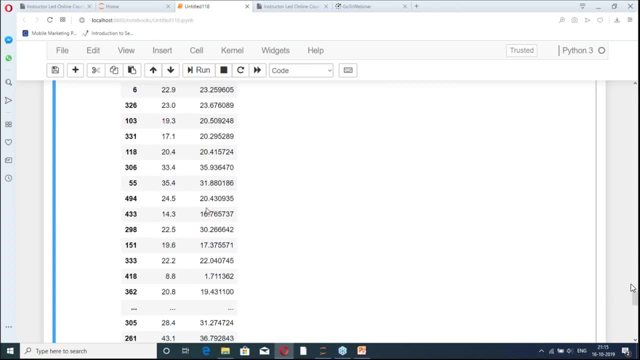 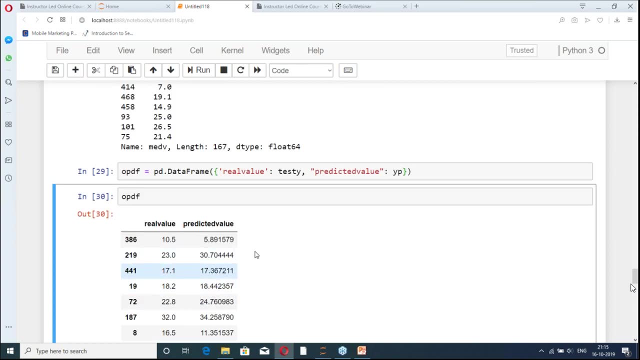 So you can see less error actually, right? So in reality, this might not be following exactly the straight line, right? So that is why we will have always error sometime. It is good to use nonlinear model, right? So this is: we use linear regression here. 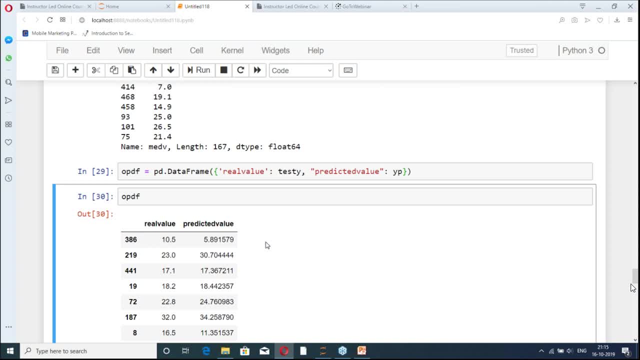 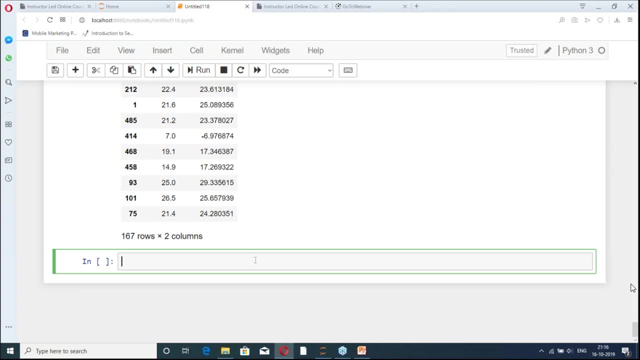 but some places it is good to use the nonlinear model, right? And let's say: if you want to calculate The, let's say: if you want to know exactly right. So we talked about: y is equal to MX plus C, equation, right? 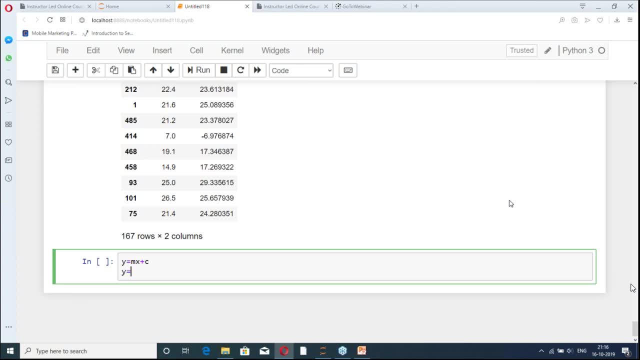 Or if we have more than one variable. so it is actually: y is equal to M 1 X 1 plus M 2 X 2. Plus and so on, right? So if we have 13 variables, it would be 13 X 13 plus C, right? 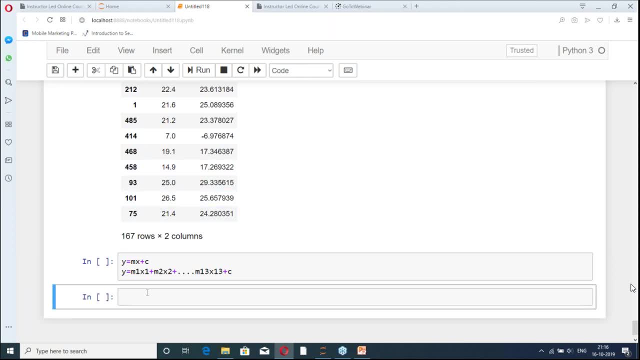 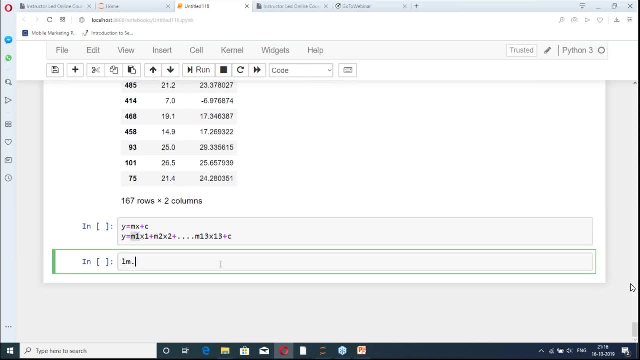 So this would be the thing here, Right? So let's say, you want to know what is my M1.. I'm going to see where you, how you can get it. So if we write LM dot, right. So if we write coefficient underscore, then it is showing me these coefficients. 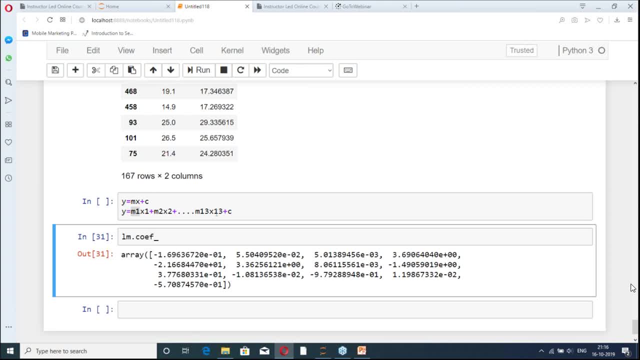 So this is first, second, third, fourth, right? So you can see, because we have 13 coefficient, So it is showing 13 values, 13 variables are there, right? I want to, I'm 13.. So this is the first coefficient value. 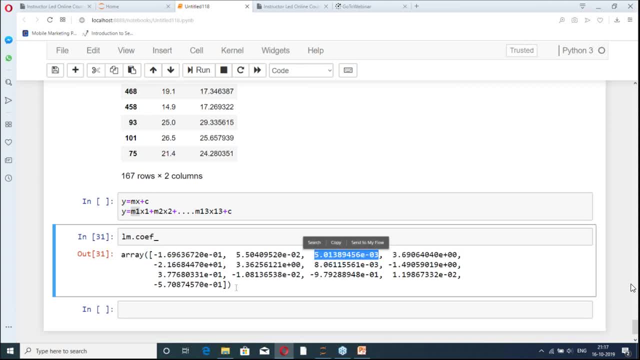 This is the second coefficient value. third coefficient, fourth and so on. So we have 13 coefficients. We get all these values. Similarly, you might be interested in finding what is the this C value. Then you can write a lamp dot intercept right. 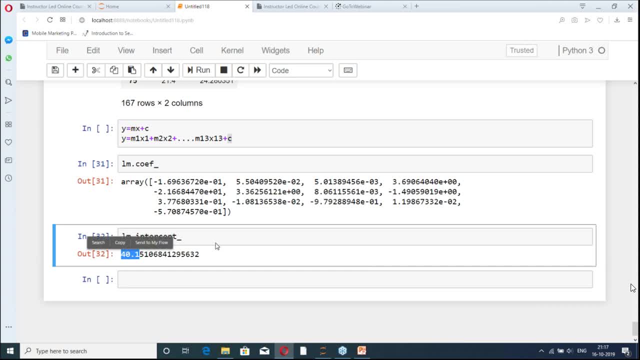 So the C value is 40.15.. So then become your equation here right, So you can see This way how easily you can apply your linear regression technique right. And there are a lot of things you can do here, like alarm dot. 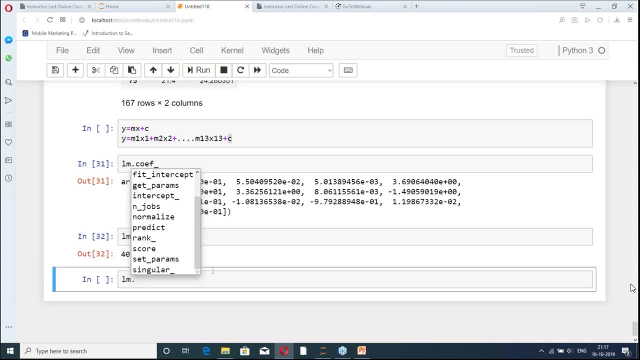 I will just keep it currently like. you can choose your score. but let me not do this thing. Let me show you one more thing, that is mean squared error. Let's say, if you want to calculate the mean squared error, how you can do is from a skill and dot matrix you import. 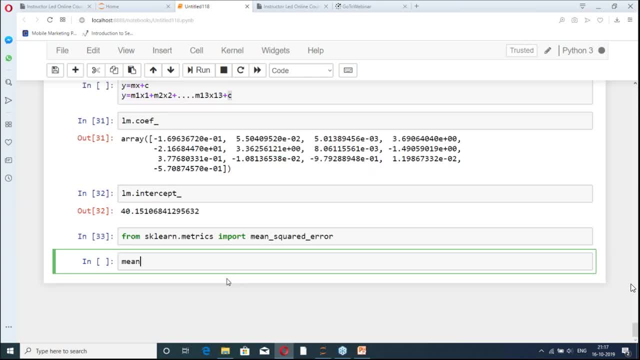 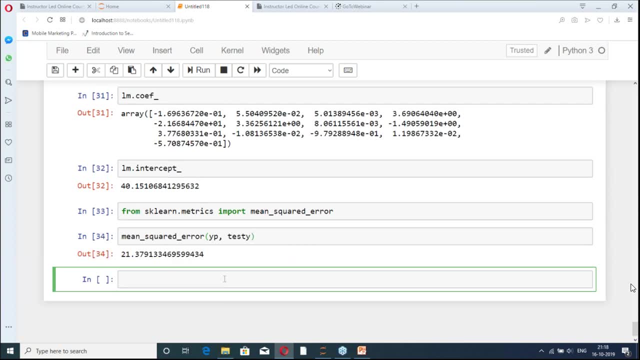 Mean squared error, right, So this is a function. you call this function. to this function, You tell what is the predicted value you have and what is the real value you have. That's right. right, So it is giving me. the square error is coming 21.27, right. 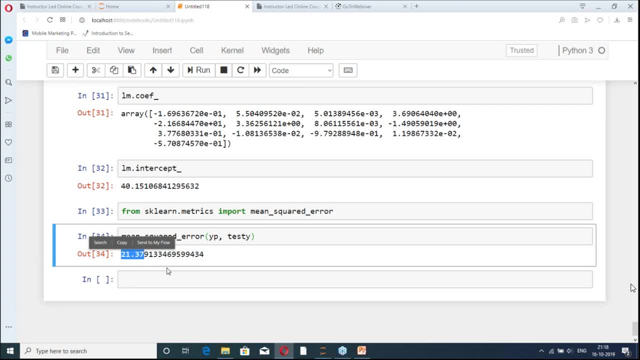 So it is little bigger in this case, actually, right? So sometimes linear model is not the good model. Actually, you might need to think that if shall I use some polynomial regression in those cases, right, But this is how you can apply your model. 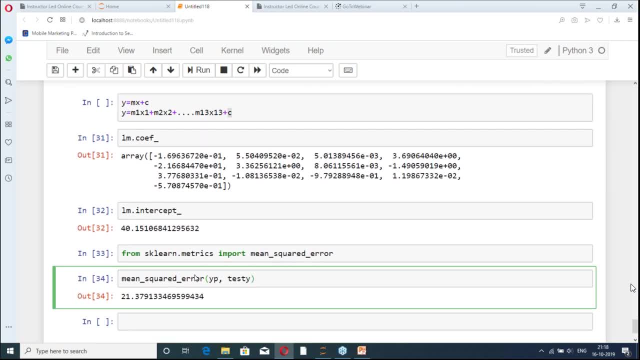 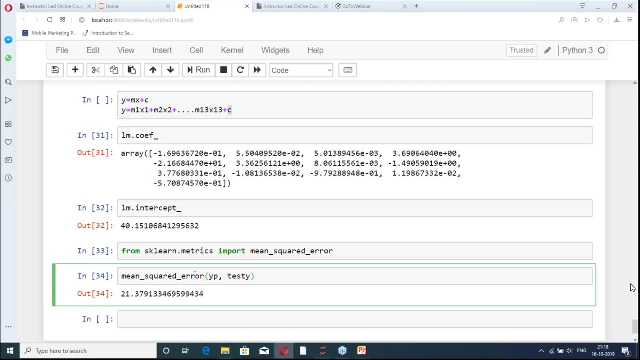 Okay, I hope so It is clear to all of you guys. Any question, Any doubt Do you guys have? If you guys have any question, let me know. Will you teach a skill and library? Yes, During the course it is being taught. 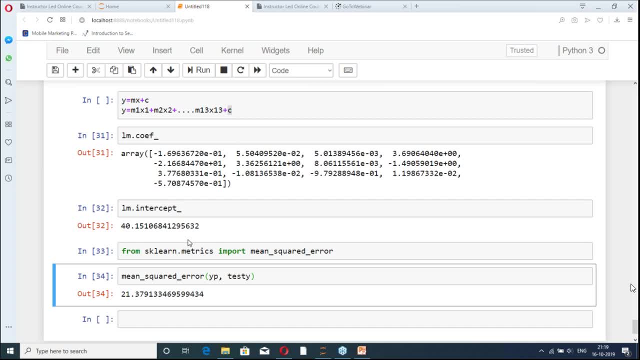 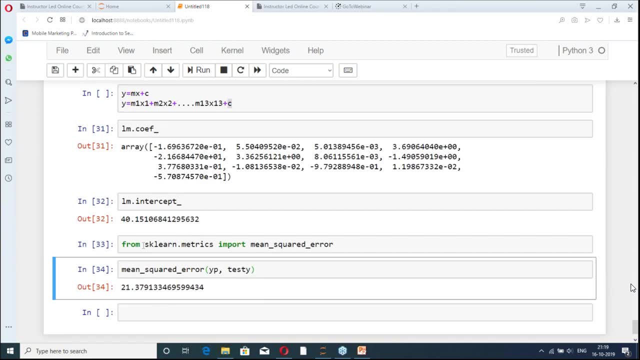 Right, And here in this case actually just for the basic part. So like maybe like tomorrow and day after tomorrow. So we have the going on. sessions are there and whenever some time few sessions get finished little earlier, So during that session I will be telling you also about these library exactly how you. 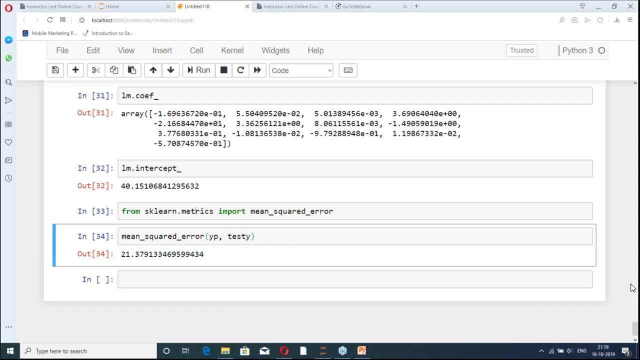 can understand these things right, Exactly What these are doing, What is the role of each of these, What is function, What is class and all So good. God is saying thanks, I appreciate your class. Thank you for appreciating. 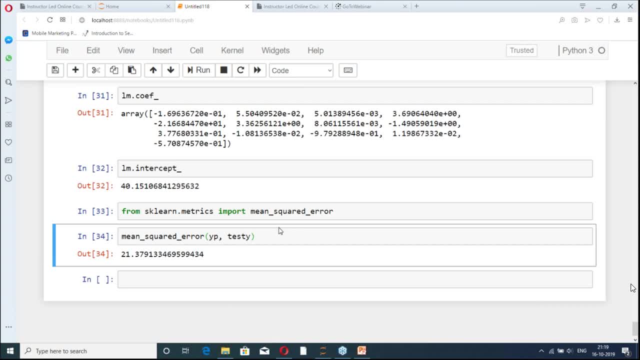 God, You have some jaggery saying why is requirement to learn math for ML when everything is predefined? See a lot of things. Yes, there is no need. In many cases is no need. But if you are going to do little bit research, work with the these stuff- machine learning- 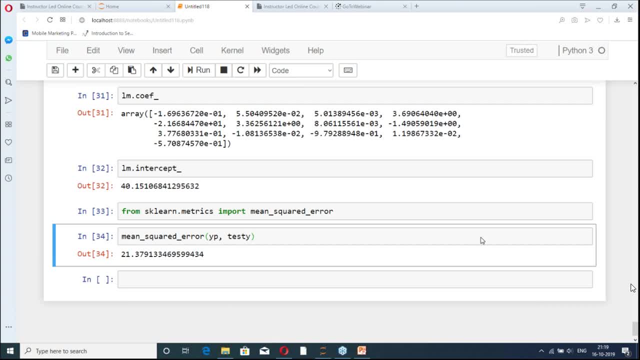 then for that you need to have the mathematics. But yes, for doing the application part it is perfectly fine. You doesn't need to go into the so much depth of the mathematics, or even you know, mid level of mathematics is also not needed. 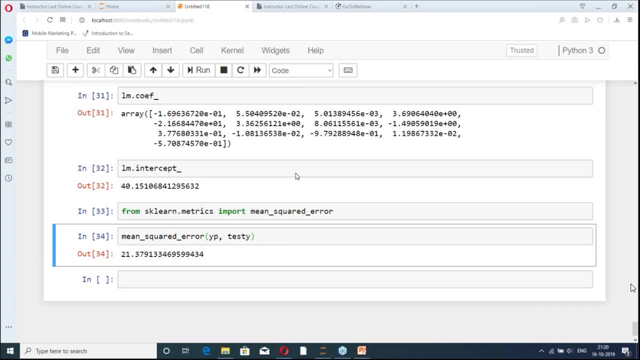 So webinar is asking: are these Python function? Yes, These are the Python function. Actually, There is a function right And that belongs to this within the SQL, And we have this model, which is matrix, within which this particular function exists. So that is what we have imported and we use it similarly earlier. 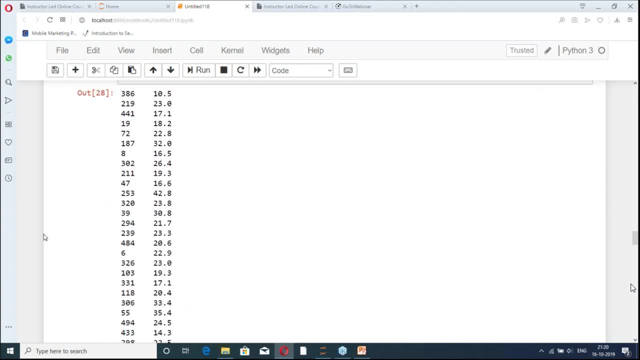 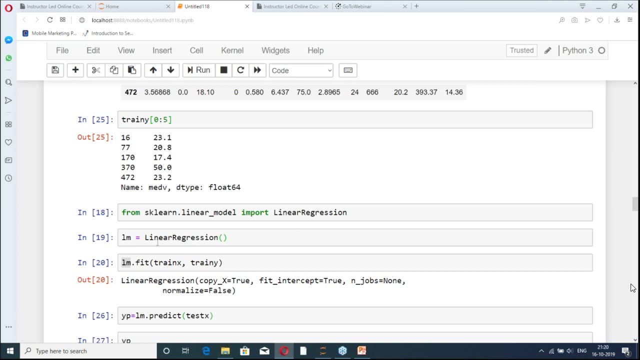 Also exactly the same thing, Right? So whatever we use a like within the SQL and this linear regression is a class actually and its object, We have created its object, right? Pascal is saying: thank you, You are welcome, Pascal. And what are they saying? 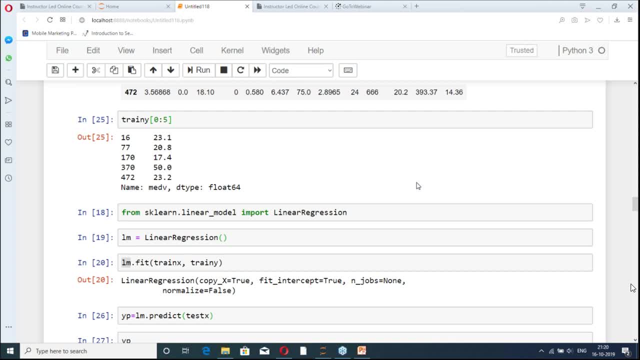 It's nice, I learned new today. Thank you, sir. Does we have certificate after this course? I during this free classes? I think the certificate will not be given, Most probably. I'm not sure about that. But yeah, if you enroll for the their courses right here, we will be doing few free sessions. 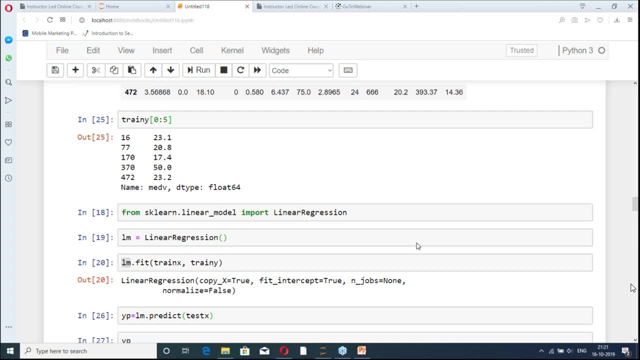 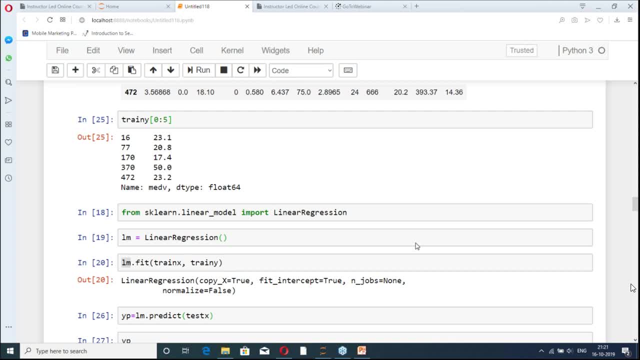 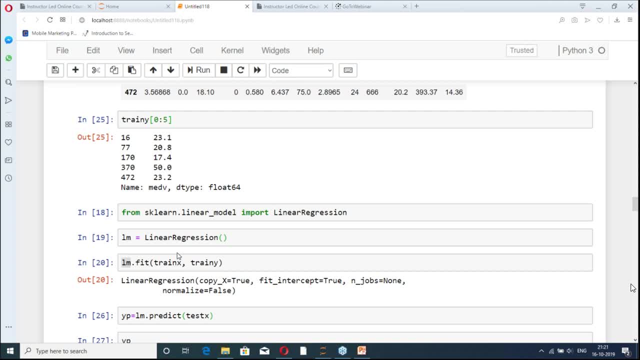 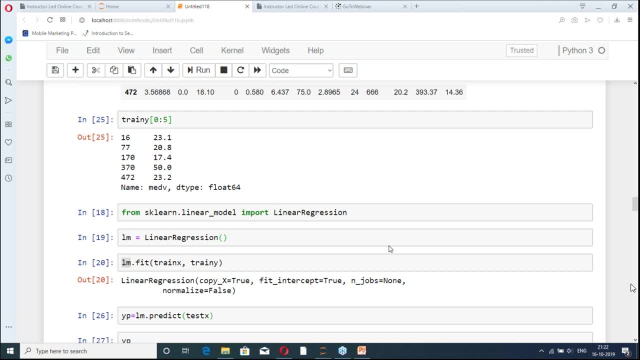 So you will get it on YouTube, So you go to that, You watch that session. It was taken by me And I discussed about the certification as well And what would be taught exactly in which certification. completely exactly right. Or, if you do not want to go, initial part, maybe you do not want to see who is data scientist. 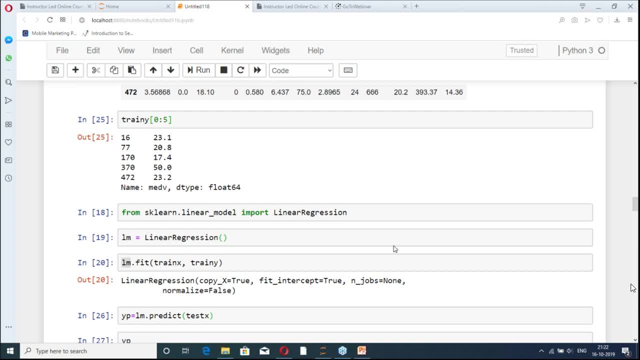 and all those stuff. You can go to the last 10, 15 minutes in the webinar, that particular YouTube video, and then you can get it. Okay, I have discussions in there. Okay, Yeah And uh, can you tell me where we can email for getting the PPT? 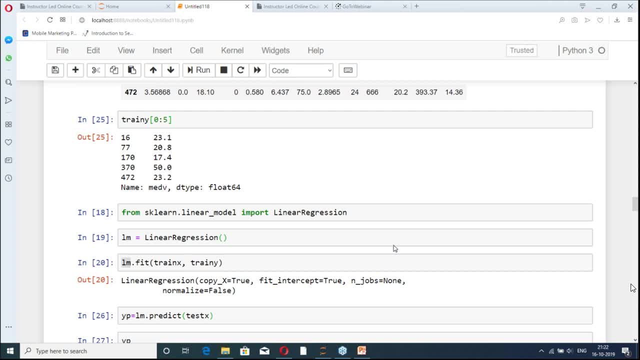 You go to their website. you will find some support email ID right, Or you will get some contact number there. You can talk to them and then they will- uh, they will tell you and you can come to tomorrow class. I will discuss with them as well. 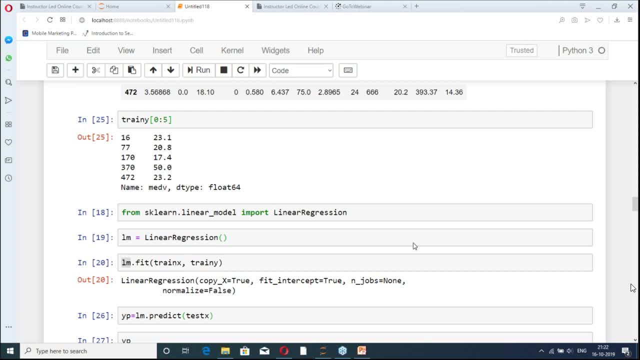 So when you are coming to tomorrow's class, I can ask them as well like today that what is the process or how they can get the PPT if they are interested? Right, So I can share it in the tomorrow classes. Okay? 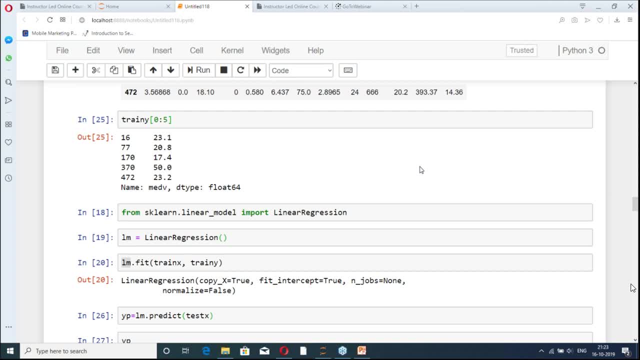 Okay, Okay, Okay, Okay, Fine, Thank you sir. Yeah, You're welcome. Okay, Okay, Great guys. Thank you very much for listening with so much patience and appreciating the- uh, appreciating the lecture session.